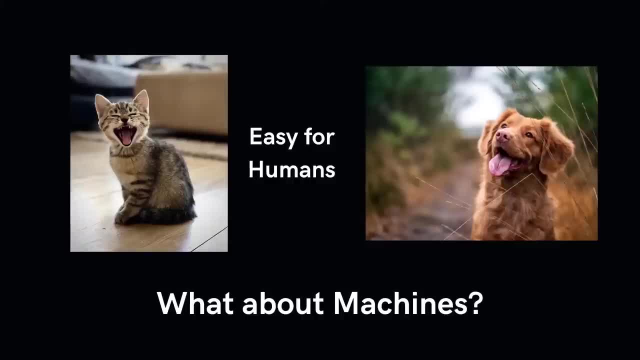 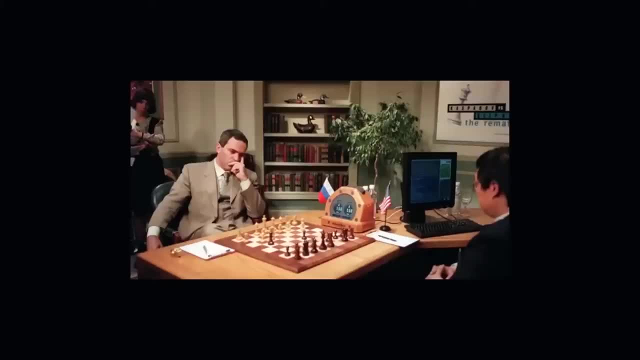 a machine to do this, and later on I will talk more about this in a later course. Before I do that, I want to give you a sense of the amazing successes of deep learning in the past. In 1997, Gary Kasperov, the most successful champion in the history of chess. 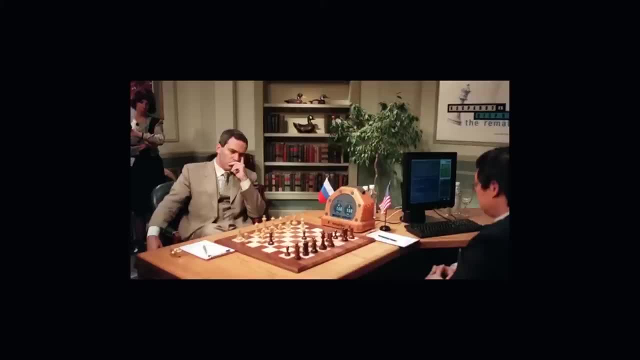 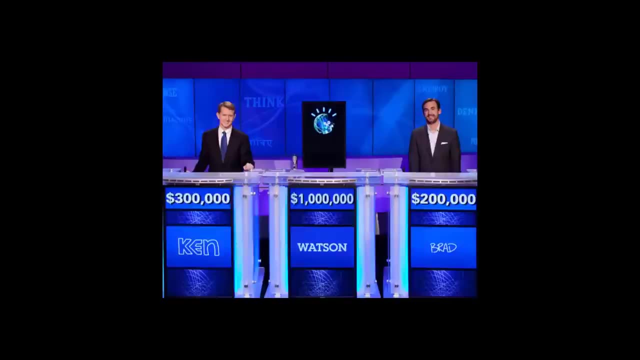 IBM's Deep Blue, one of the first computer or artificial systems. It was the first defeat of a reigning world chess champion by a computer. In 2011,, IBM's Watson competed in the game show Jeopardy against its champions Brad Rotter and Ken Jennings and won the first prize of a million dollars. 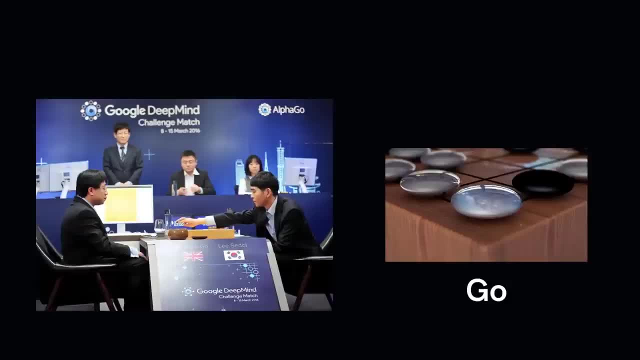 In 2015,, AlphaGo, a deep learning computer program created by Google's DeepMind division, defeated Lee Sedol, an 18-time world champion at Go- a game a Google more times complex than chess. But deep learning can do more than just beat us at board games. it finds applications anywhere. 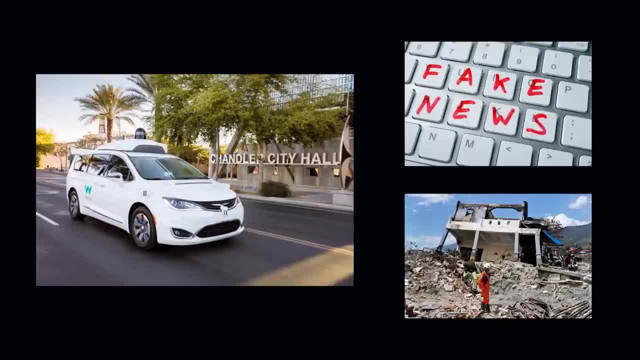 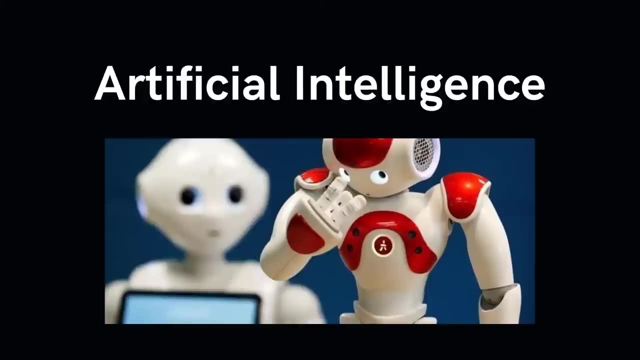 from self-driving vehicles to fake news detection, to even predicting earthquakes. These were astonishing moments, not only because machines beat humans at their own games, but because of the endless possibilities that they opened up. What followed such events have been a series of striking breakthroughs in artificial intelligence. 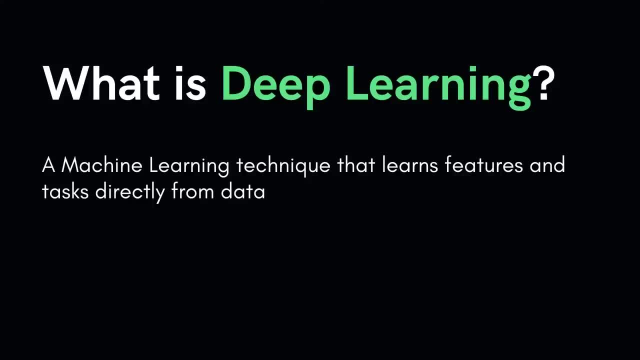 machine learning and, yes, deep learning. To put it simply, deep learning is a machine learning technique that learns features and tasks directly from data by running inputs through a biologically-inspired neural network architecture. These neural networks contain a number of hidden layers through which data is processed. 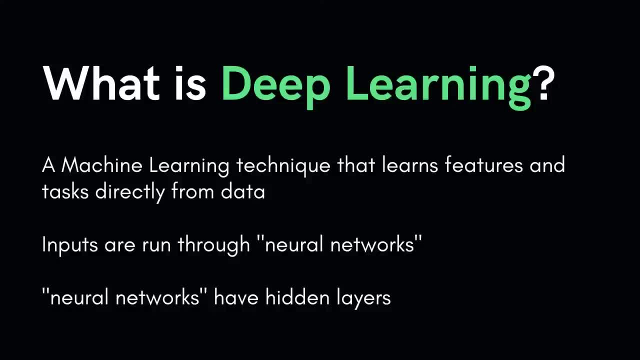 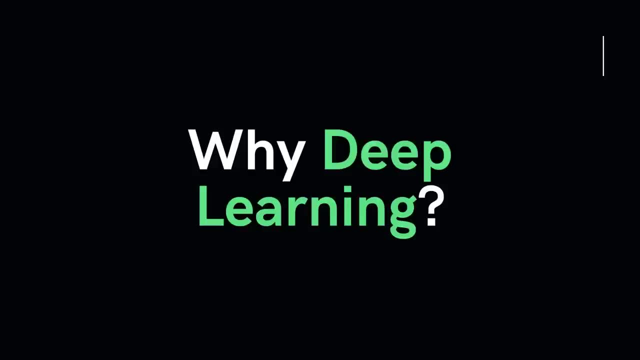 allowing for the machine to go deep in its learning, making connections and weighing input. for the best results, We'll go over neural networks in the next video. So why deep learning? 1. Maintenance: The problem with traditional machine learning algorithms is that, no matter how complex they, 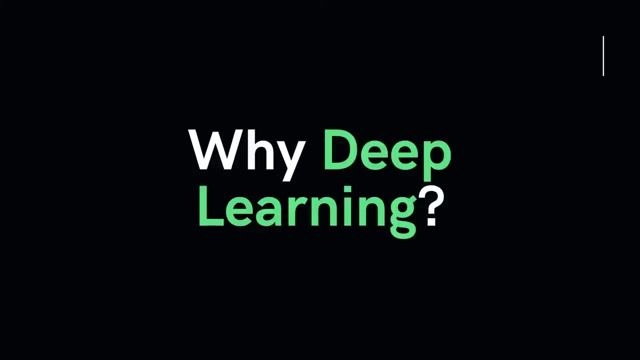 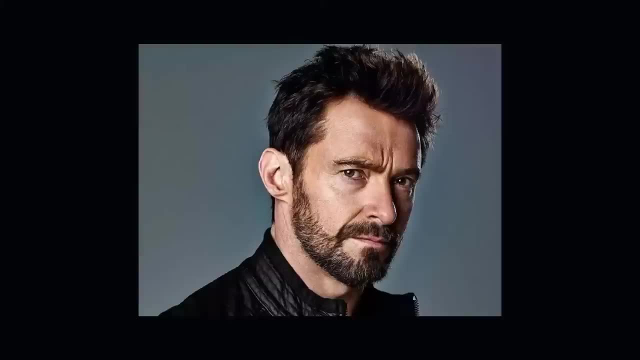 get. they'll always be machine-like, They need a lot of domain expertise, human intervention and are only capable of what they're designed for. For example, If I show you the image of a face, you will automatically recognize it's a face. 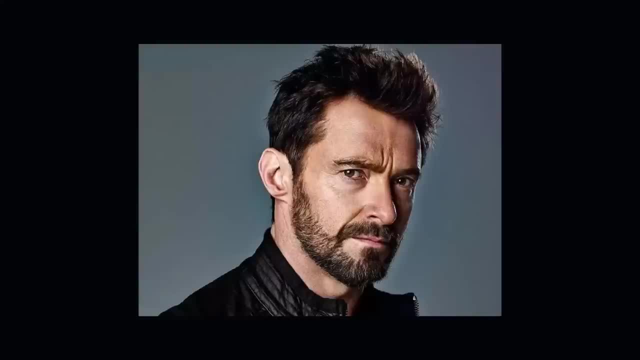 But how would a computer know what this is? Well, if we follow traditional machine learning, we'd have to manually and painstakingly define to a computer what a face is. For example, it has eyes, ears and a mouth. But how do you define a face? 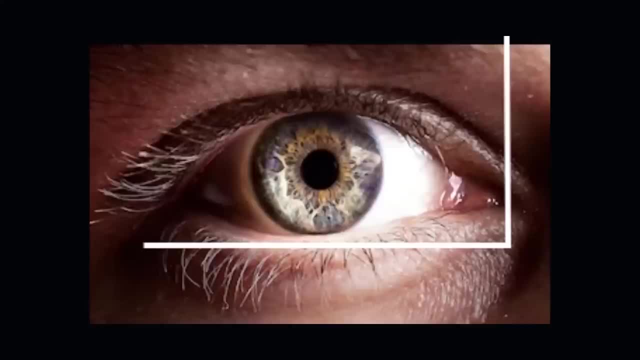 1. find an eye or a mouth to a computer. Well, if you look at an eye, the corners are at some angle. They're definitely not 90 degrees. they're definitely not zero degrees. there's some angle in between. So we could work with that and train our 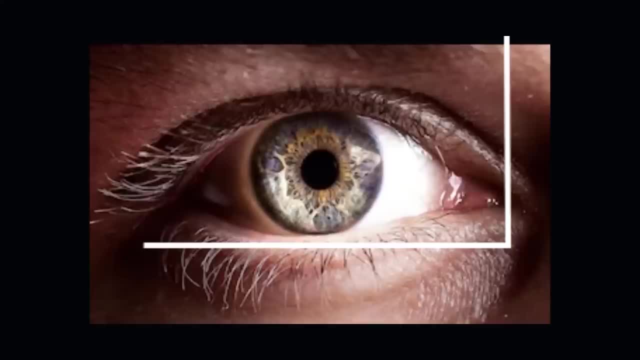 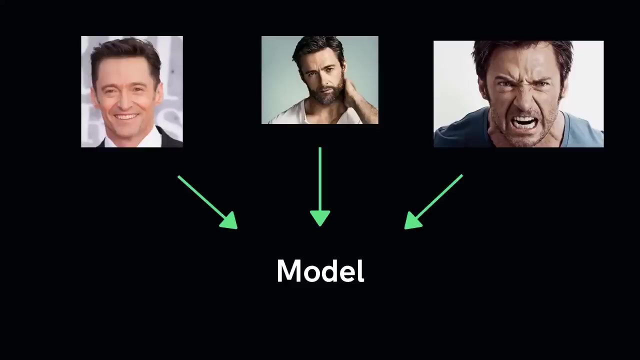 classifier to recognize these kinds of lines in certain orientations. This is complicated For AI practitioners and the rest of the world. that's where deep learning holds a bit of promise. The key idea in deep learning is that you can learn these features just from raw data. So I can feed a bunch of images of faces. 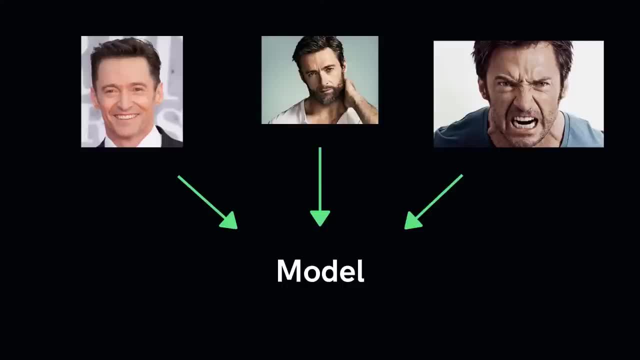 to my deep learning algorithm and it's going to develop some kind of hierarchical representation of detecting lines and edges and then using these lines and edges to detect eyes and a mouth and composing it together to ultimately detect the face. As it turns out, the underlying algorithms for 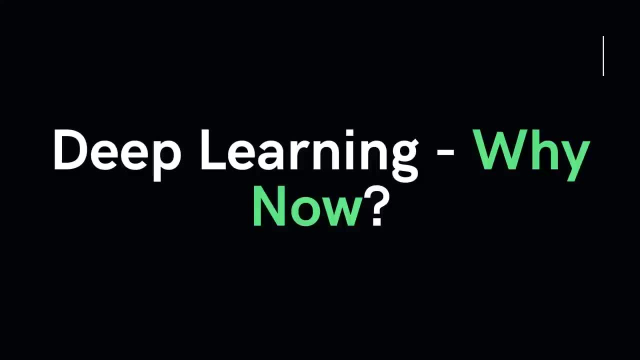 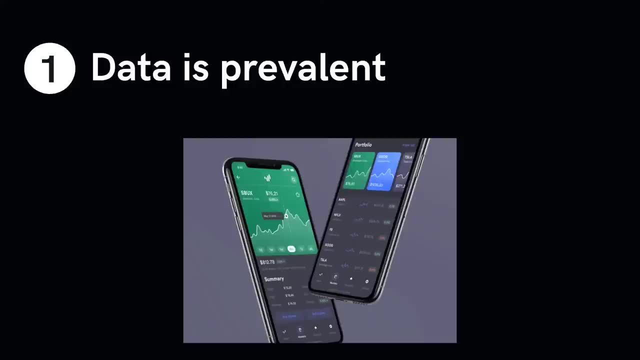 training. these models have existed for quite a long time, So why has deep learning gaining popularity many decades later? Well, for one, but data has become much more pervasive. We're living in the age of big data, and these algorithms require massive amounts of data to effectively be implemented. 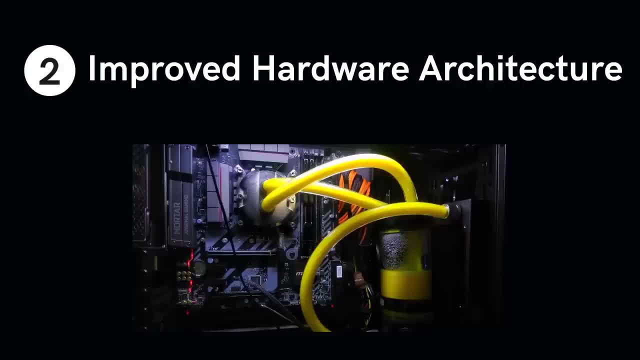 Second, we have hardware and architecture that are capable of handling the vast amounts of data and computational power that these algorithms require, Hardware that simply wasn't available a few decades ago. Third, building and deploying these algorithms- models, as they're called- it's. 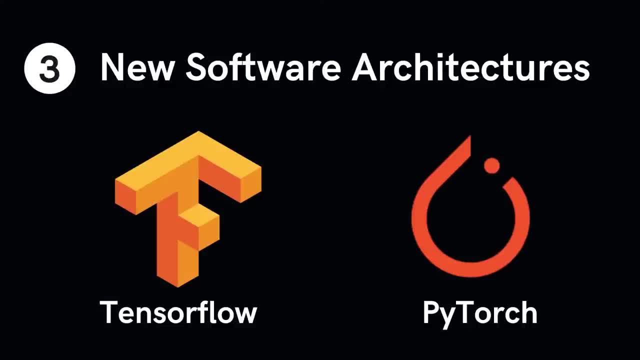 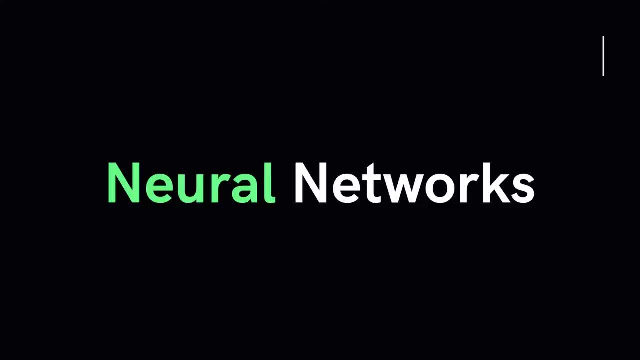 extremely streamlined with the increasing popularity of open-source software like Github, Like TensorFlow and PyTorch. Deep learning models refer to the training of things called neural networks. Neural networks form the basis of deep learning, a sub-field of machine learning where algorithms are inspired by the structure of the human brain, Just like. 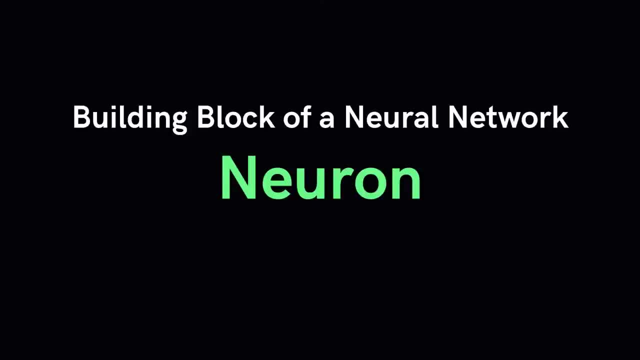 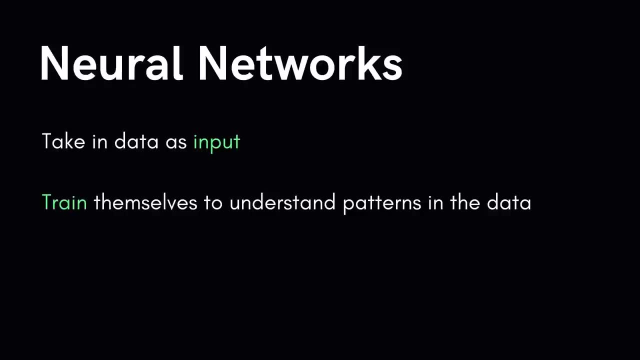 neurons make up the brain. the fundamental building blocks of a neural network is also a neuron. Neural networks take in data. they train themselves to recognize patterns in this data and predict outputs for a new set of data. The new networks take in data. they train themselves to recognize patterns in this data and predict outputs for a new set of data. 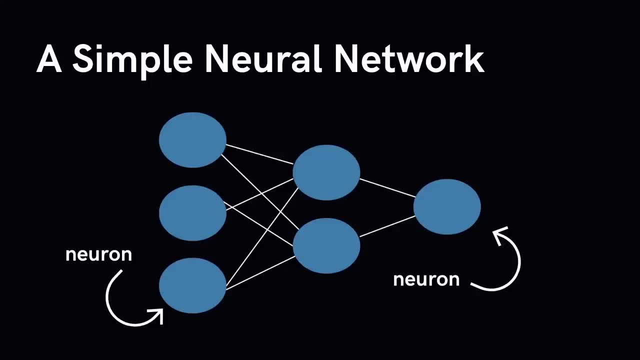 for a new set of similar data. In a neural network, information propagates through three central components that form the basis of every neural network architecture: The input layer, the output layer and several hidden layers between the two. In the next video, we'll go over the learning process of a neural network. 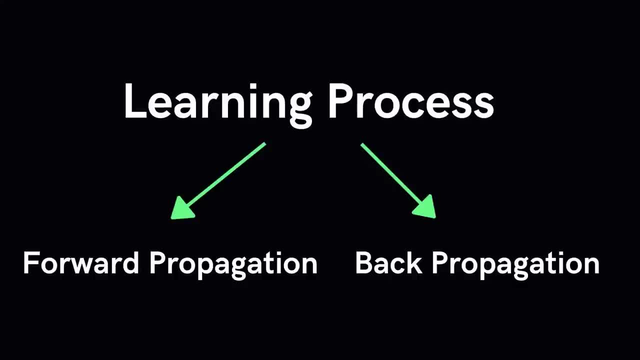 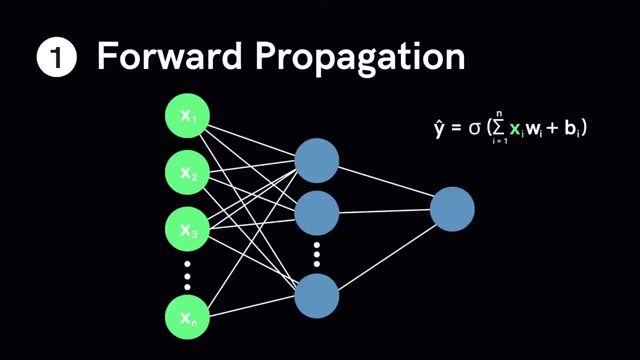 The learning process of a neural network can be broken into two main processes: forward propagation and back propagation. Forward propagation is the propagation of information from the input layer to the output layer. We can define our input layer as several neurons: x1 through xn. 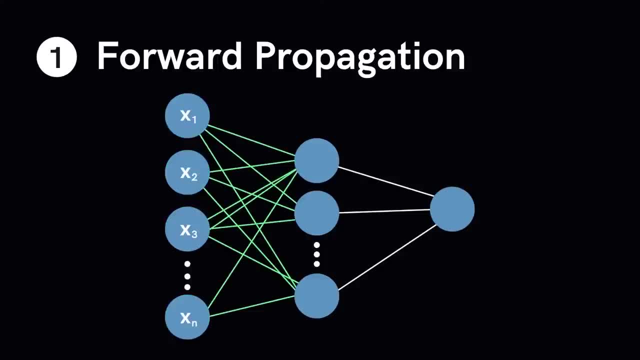 These neurons connect to the neurons of the next layer through channels and they are assigned numerical values called weights. The inputs are multiplied to the weights and their sum is sent as input to the neurons in the hidden layer, where each neuron in turn is associated to a numerical value called. 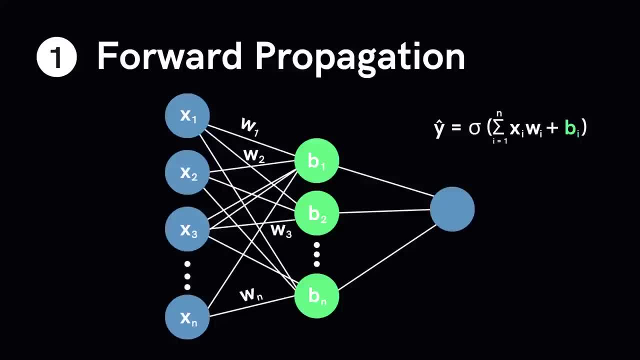 the bias, which is then added to the input sum. So this credited value will then be accumulated between the two neurons. This weighted sum is then passed through a non-linear function called the activation function, which essentially decides if that particular neuron can contribute to the next. 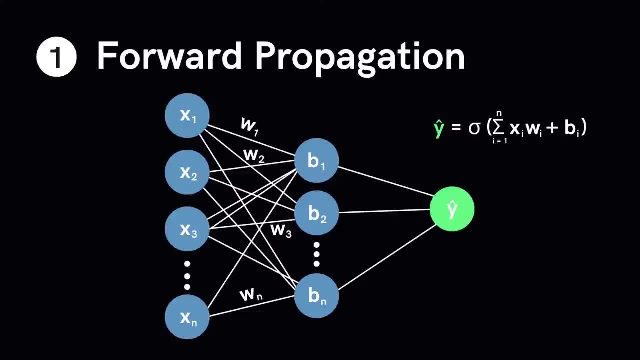 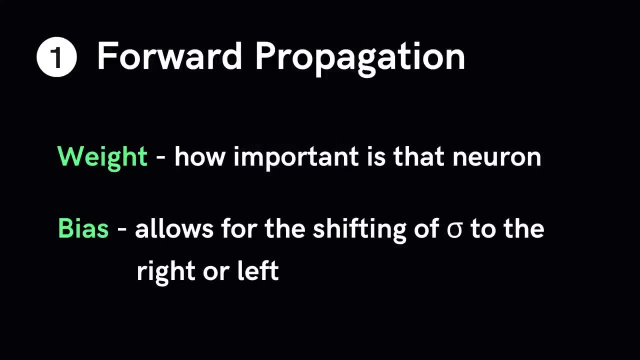 layer In the output layer. it's basically is a form of probability. The neuron with the highest value determines what the output finally is. Let's look at some other sources. The weight of a neuron can tell us how important a neuron is. 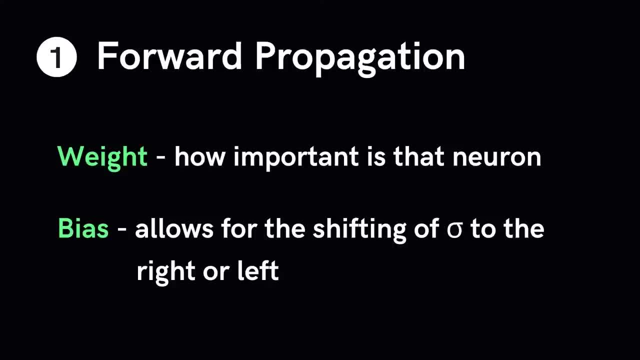 The higher the item, the more important it's. activity: The value of a magnet E to a beacon, E to dy mortal on having an opinion, to the relationship. It serves to shift the activation function to the right or to the left. If you have had some experience with high 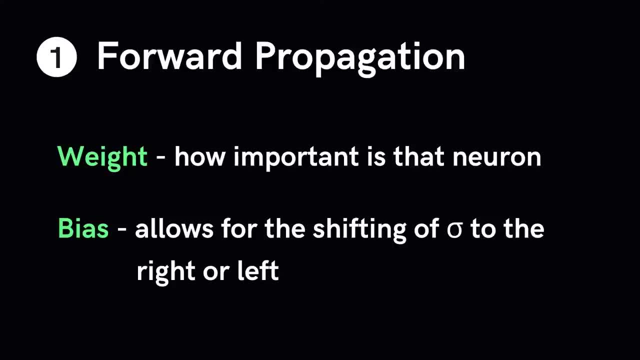 school math. you should know that adding a scalar value to a function shifts the graph either to the left or to the right, and this is exactly what the bias does: It shifts the activation function to the right or to the left. Bad propagation is almost like full propagation, except in the reverse direction. Information here. 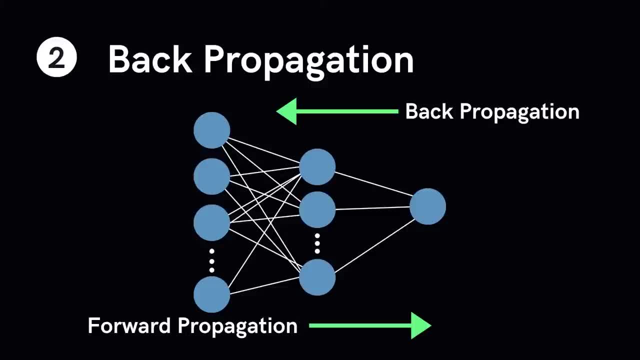 is passed from the output layer to the hidden layers, not the input layer. But what information gets passed on from the output layer? Isn't the output layer supposed to be the final layer where we get the final output? Well, yes, but no. 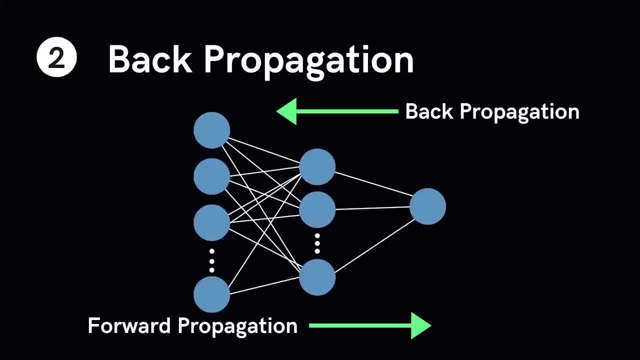 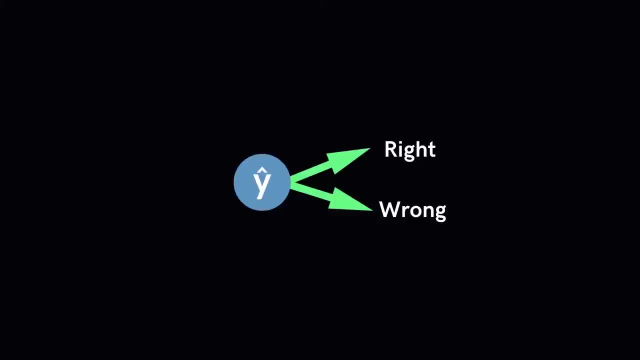 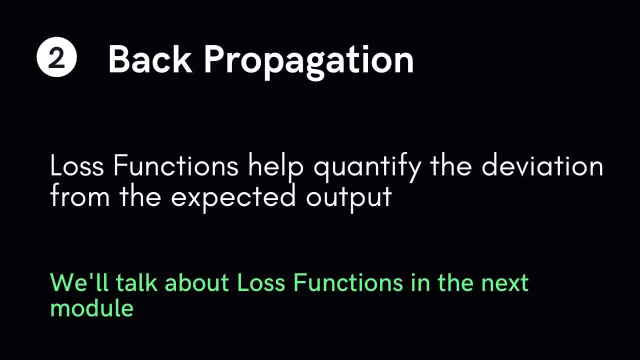 Bad propagation is the reason why neural networks are so powerful. It is the reason why neural networks can learn by themselves. In the last step of all propagation, a neural network spits out a prediction. This prediction could have two possible possibilities: either right or wrong. In bad propagation, the neural network. 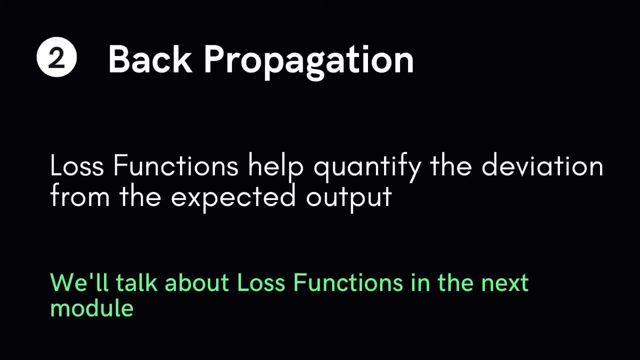 evaluates its own performance and checks if it is right or wrong. If it is wrong, the network uses something called a loss function to quantify the deviation from the expected output, and it is this information that's sent back to the hidden layers for the weight and biases to be adjusted so that the network's 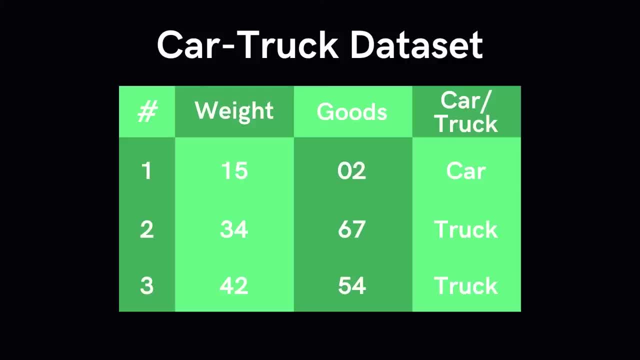 accuracy level increases. Let's visualize the training process with a real example. Let's suppose we have a data set. This data set us the weight of a vehicle and the number of goods carried by that vehicle, and also tells us if those vehicles are cars or trucks. we want to go through this data trade, our neural networks. 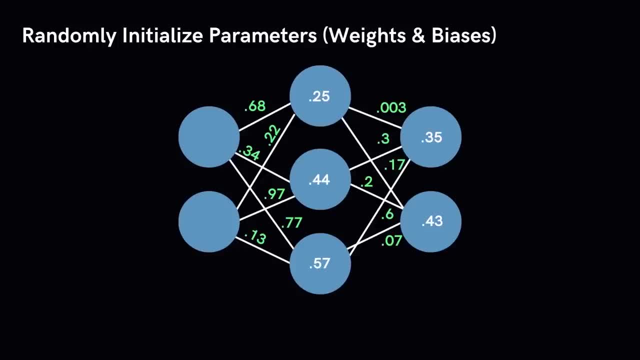 to predict cars or trucks based on their weights and goods. to start off, let's initialize the neural network by giving it random weights and biases. these can be anything. we really don't care what these values are, as long as they're there in the first entry of a data set. we have vehicle weight. 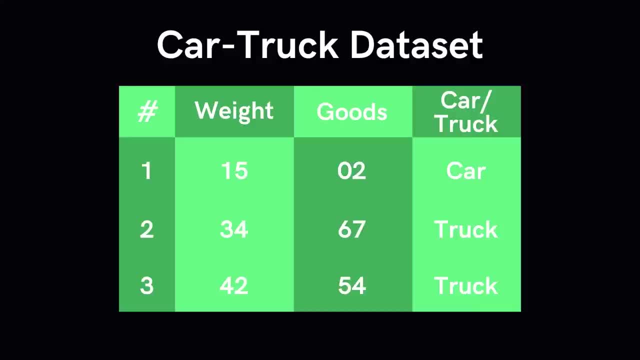 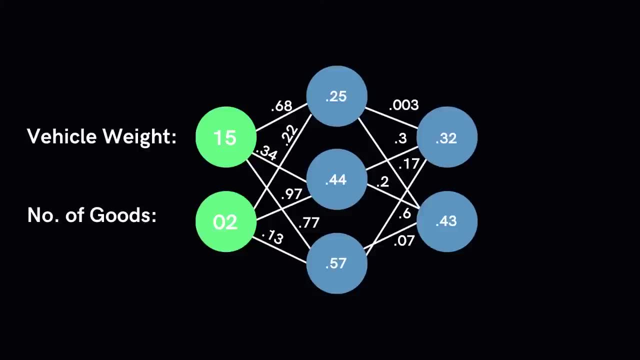 equal to a value, which in this case is 15, and goods as 2.. according to this, it's a car. we now start moving these input dimensions through the neural network. so, basically, what we want to do is take both the inputs, multiply them by their weight and add a bias, and this is where the magic. 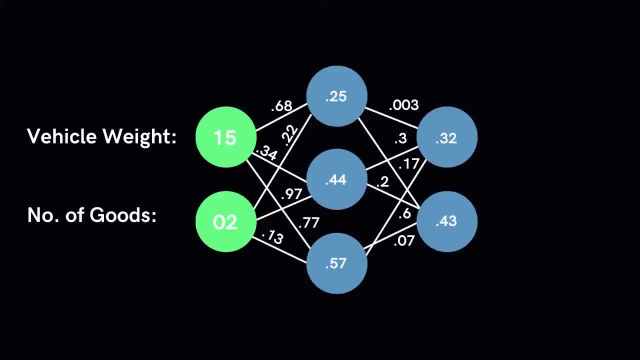 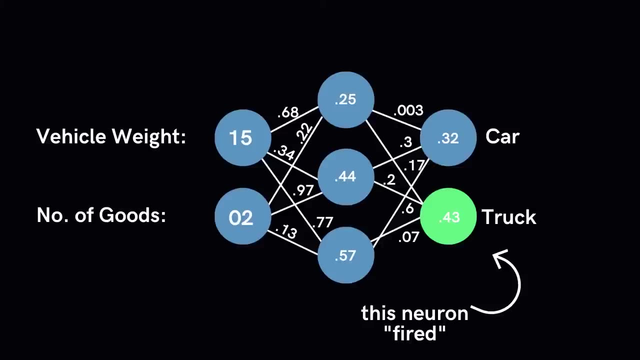 happens, we run this weighted sum through an activation function. okay, now let's say that the output of this activation function is 0.001. this again is multiplied by the weight and add it to the bias and finally, in the output layer, we have a guess. now, according to this neural network, the type of vehicle with weight 15 and goods 2. 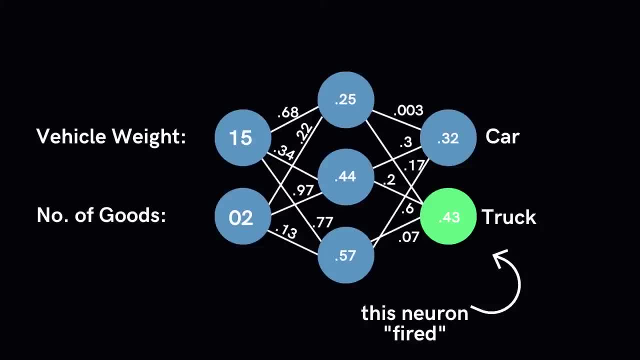 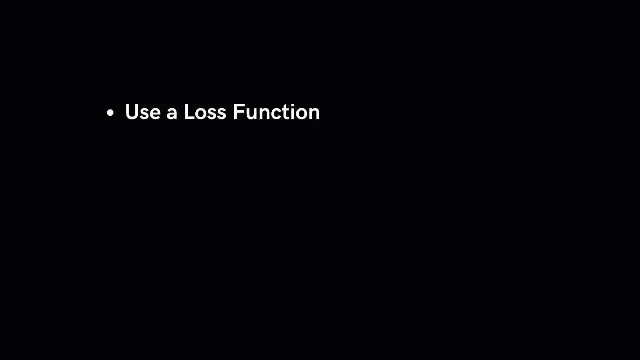 has a greater probability of being a truck. of course this is not true, and a neural network knows this. so we use back propagation. we're going to quantify the difference between the expected result and the predicted output using our most function in back propagation. we're going to go. 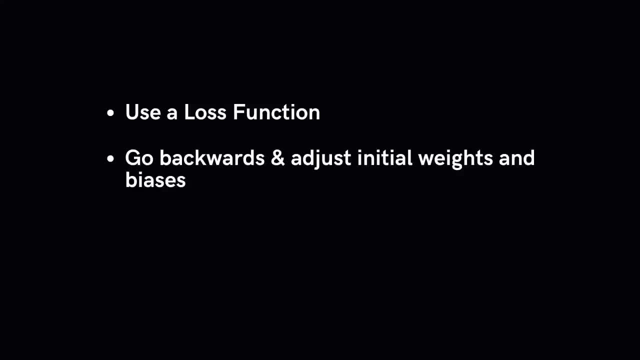 backwards and adjust our initial weights and biases. remember that during the initialization of the completely random weight and biases, Well, during backpropagation, these values will be adjusted to better fit the prediction model. Okay, so that was one iteration. through the first piece of the data set In the second entry we have 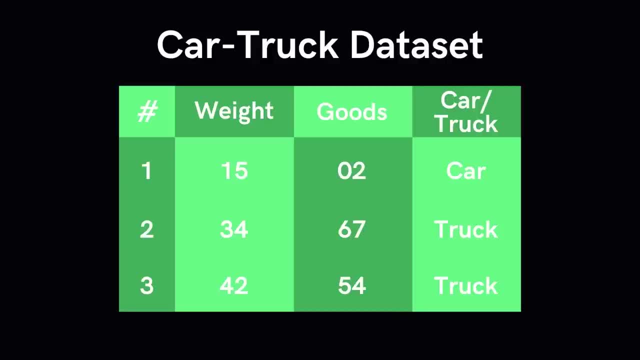 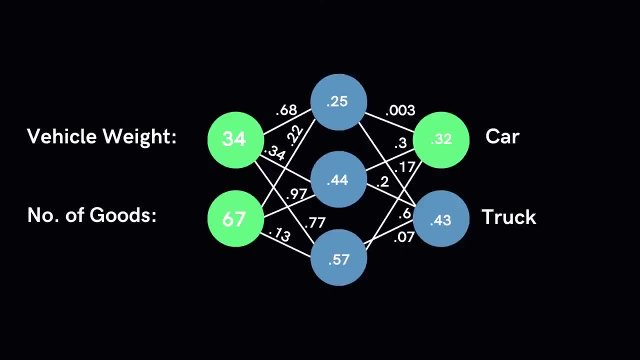 vehicle weight 34 and goods 67.. We're going to use the same process as before: multiply the input with the weight and add a bias. Pass this result into an activation function and repeat till the output layer. Check the error difference and employ backpropagation to adjust the weights and the biases. Your new 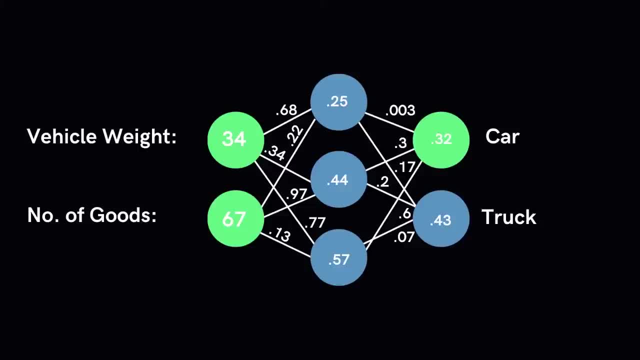 network will continue doing this repeated process of forward propagation, calculating the error and then backpropagation for as many entries there are in this data set. The more data you give the new network, the better it will be at predicting the right output. But there's a trade-off, because too much 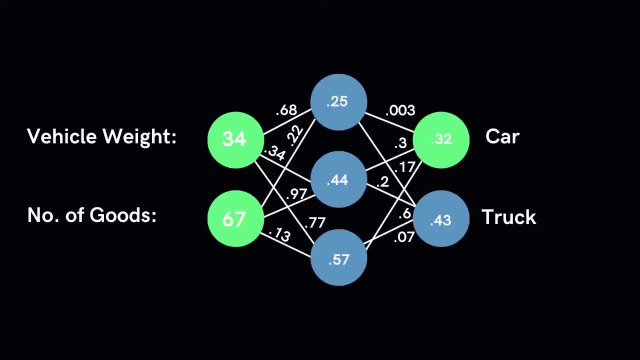 data and you'll end up with a problem like overfitting, which I'll discuss later on this course. But that's essentially how a new network works. You feed, input, the network initializer will treat the error and then the data will be read to the. 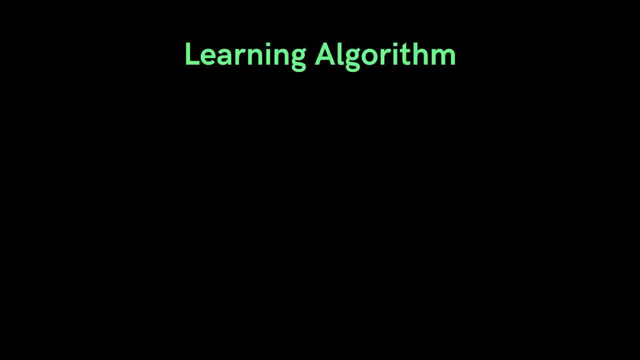 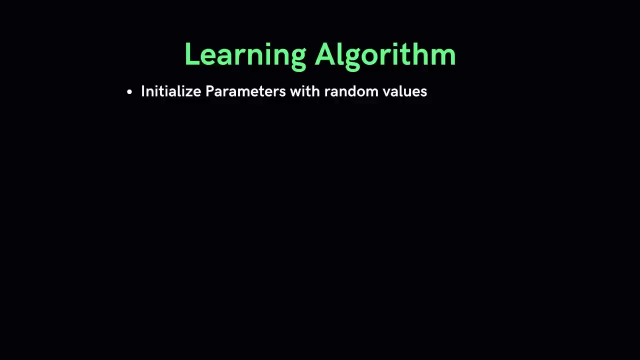 random weights and biases that are adjusted each time during backpropagation until the network has gone through all your data and is now able to make predictions. This learning algorithm can be summarized as follows: First, we initialize the network with random values for the network's parameters, or 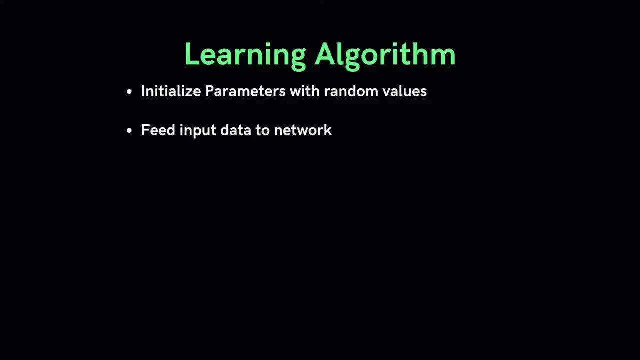 the weights and biases. We take a set of input data and pass them through the network. We compare these predictions obtained with the values of the expected labels and calculate the loss using a loss function. We perform backpropagation in order to propagate this loss to each and every weight and bias. 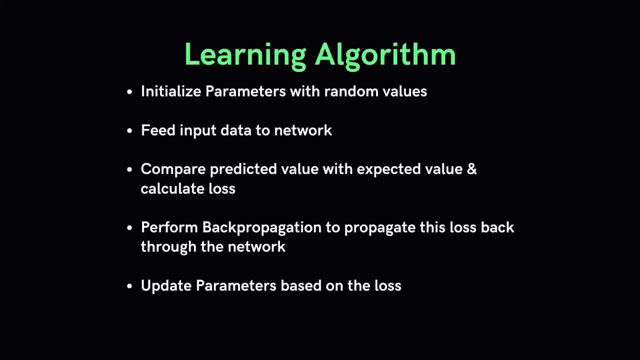 We use this propagated information to update the weights and biases of the new network with the gradient descent algorithm in such a way that the total loss is reduced and a better model is obtained. The last step is to continue iterating the previous steps until we consider that we have 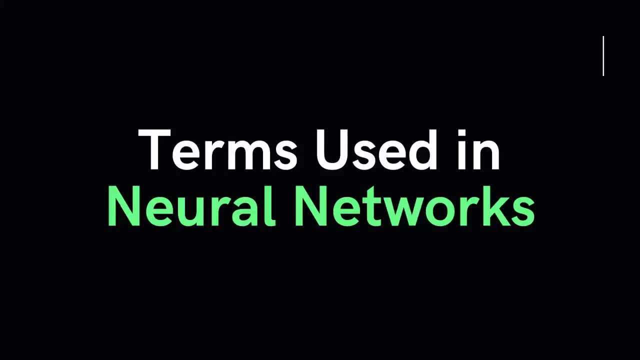 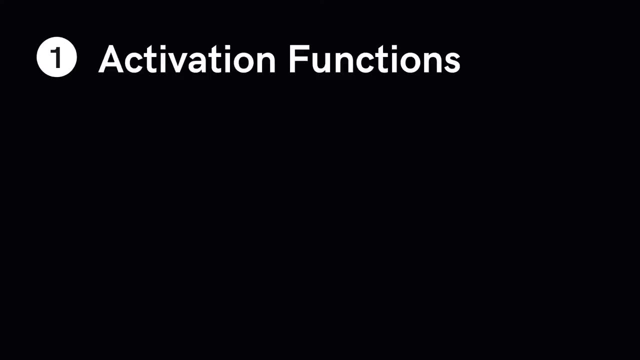 a good enough model. In this section, we're going to look at how to create a new model. We're going to talk about the most common terminologies used in deep learning today. Let's start off with the activation function. The activation function serves to introduce something called non-linearity into the network. 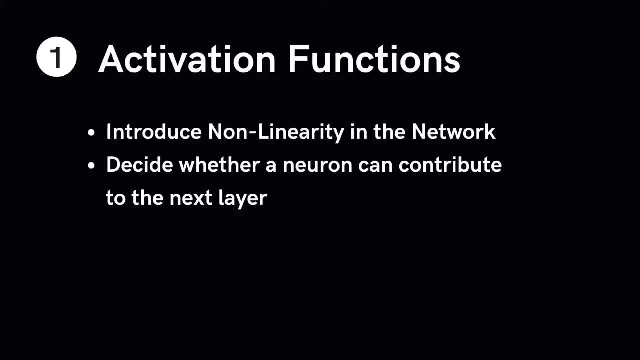 and also decides whether a particular neuron can contribute to the next layer. But how do you decide if the neuron can fire or activate? We had a couple of ideas which led to the creation of different activation functions. The first idea we had is: how about we activate the neuron? 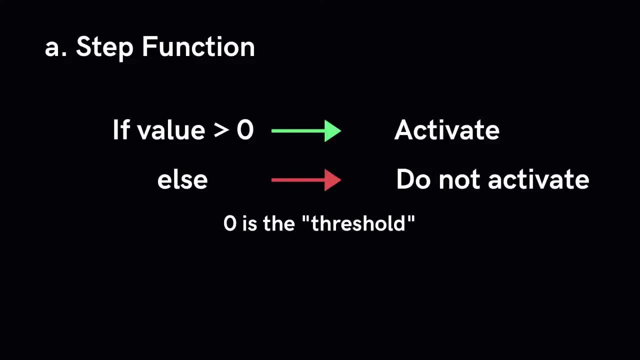 We activate the neuron if it is above a certain value or threshold. If it is less than this threshold, don't activate it. Activation function a is equal to activated if y is greater than some threshold. else it's not. This is essentially a step function. 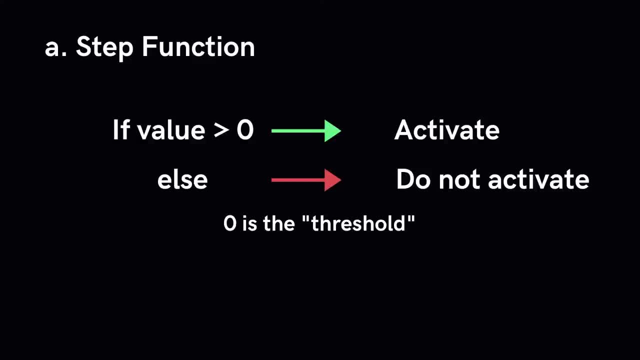 Its output is 1 or activated when value is greater than 0. Its output is activated when value is greater than some threshold and output is not activated otherwise. Great. so this makes an activation function for a neuron. No confusions. The wave is perfect. except there are some drawbacks with this. 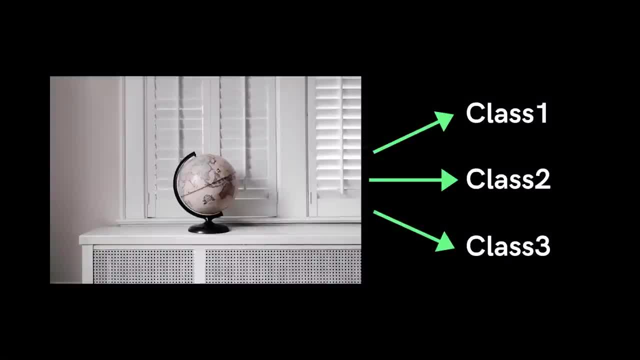 To understand it better, think about the following. Think about a case where you want to classify multiple such neurons into classes, Say class 1, class 2, class 3, etc. What will happen if more than one neuron is activated? All these neurons will output a 1.. 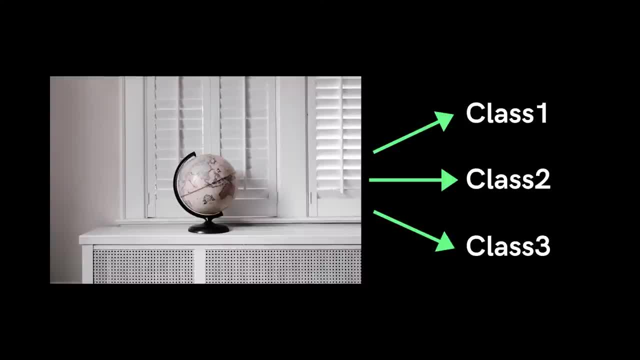 Well, how do you decide which class it belongs to? It's complicated, right. You would want the network to activate only one neuron. This should be 0. Only then you would be able to say it was classified properly. In real practice, however, it is harder to train and converge it this way. 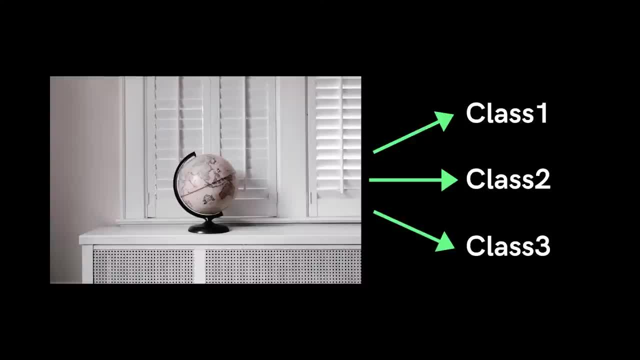 It would be better if the activation was not binary and instead some probable value like 75% activated or 16% activated, there's a 75% chance that it belongs to class 2, etc. Then, if more than one neuron activates, you could find which neuron fires based on which. 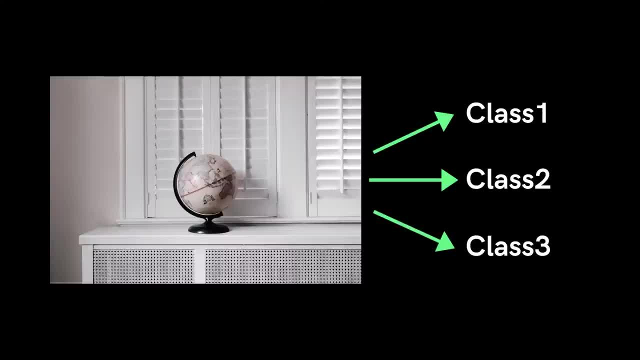 has the highest probability. Okay, Maybe you'll ask yourself: I want something to give me a more analog value, rather than just saying activated or not activated, Something other than in binary. And maybe you would have thought about a linear function, a straight line function, where the 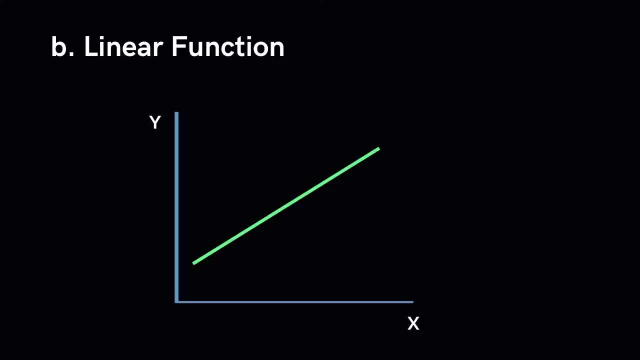 activation is proportional to the input by a value called the slope of the line. This way it gives us a range of activations, so it isn't binary activation. We can definitely connect a few neurons together and if more than one fires we could take. 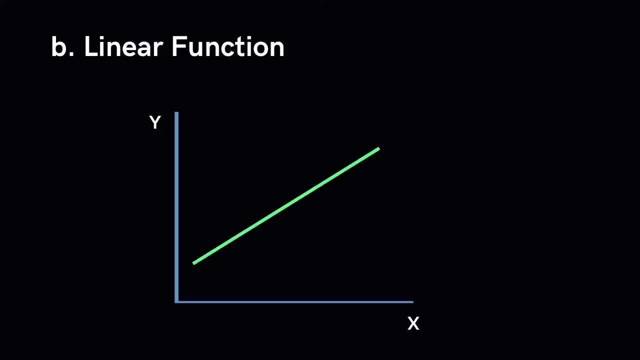 the maximum value and decide based on that. So that is okay too. What's wrong with this? Well, if you are familiar with gradient descent, which I'll come to in just a bit, You'll notice that the derivative of a linear function is a constant. 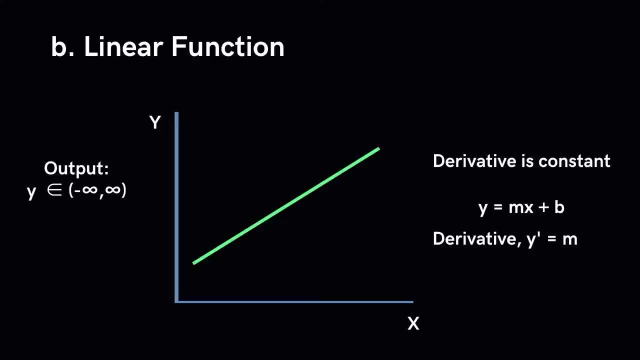 Makes sense, because the slope isn't changing at any point. For a function, f is equal to mx plus c. the derivative is m. This means that the gradient has no relationship whatsoever with x. This also means that during backpropagation, the adjustments made to the weights and the 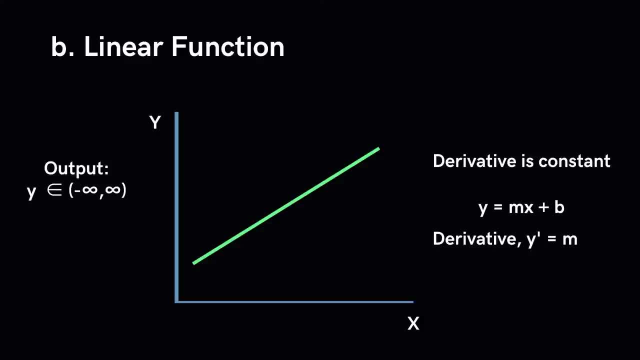 biases aren't dependent on x at all. This is not a good thing. Additionally, think about if you have a gradient descent that has no relationship whatsoever with x. this is not a good thing. For example, if you have a gradient descent that has no relationship. 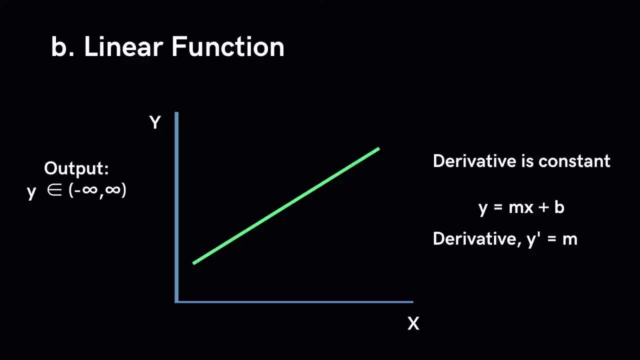 connected layers. No matter how many layers you have, if all of them are linear in nature, the activation function of the final layer is nothing but just a linear function of the input of the first layer. Pause for a bit and think about it. This means that the entire neural network of dozens of layers can be 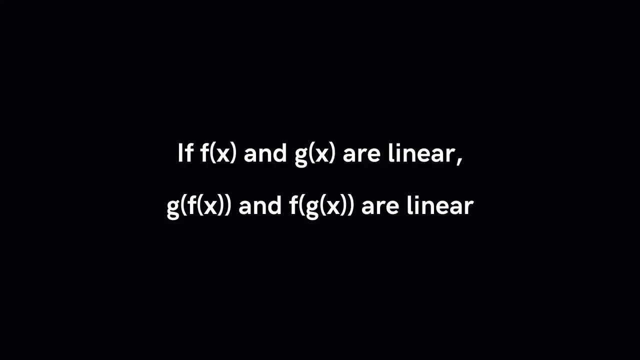 replaced by a single layer. Remember, a combination of linear functions in the linear manner is still another linear function, And this is terrible because we've just lost the ability to stack layers. this way, No matter how much we stack, the whole network is still equivalent to a single layer with single 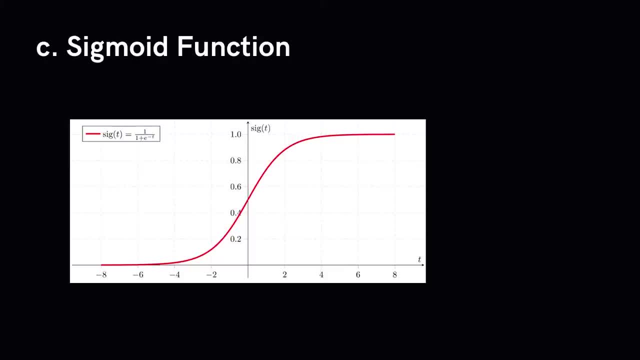 activation. Next we have a sigmoid function, and if you've ever watched a video on activation functions, this is the kind of function used in the examples. A sigmoid function is defined as a of x is equal to 1 over 1 plus e to the negative x. Well, this looks smooth and kind of like a step function. What? 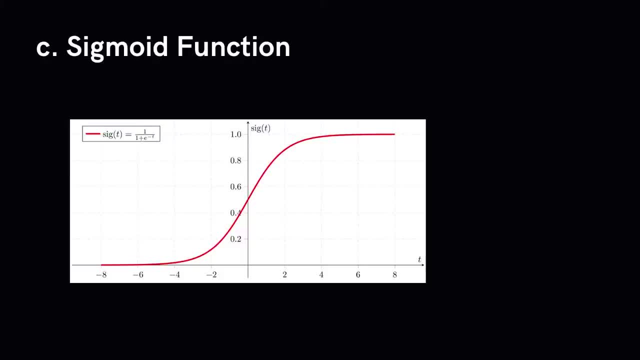 are its benefits? Think about it for a moment. Well, first things first, it has nonlinear nature. Combinations of this function are also nonlinear. Great, so now we can stack layers. What about non-binary activations? Yes, that too, This function outputs an. 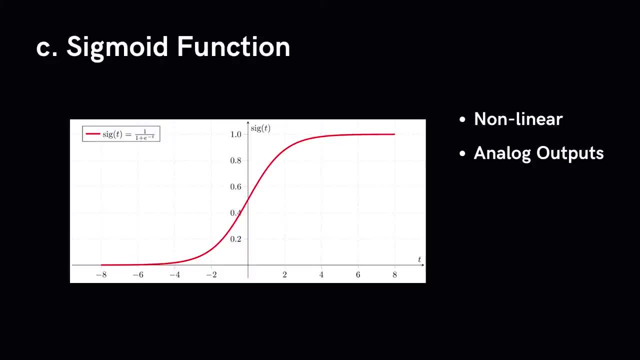 analog activation, unlike the step function and also has a smooth gradient. An advantage of this activation function is that, unlike the linear function, the output of this function is going to be in the range 0 to 1 inclusive, compared to the negative infinity to infinity of the latter. So we have our activations. 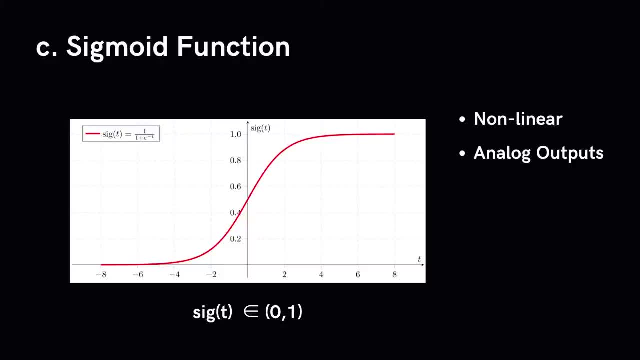 bound in the range and this won't blow up. So we have a combination of nonlinear and non-binary activations, And this is great. and sigmoid functions are one of the most widely used activation functions today. But life isn't always rosy and sigmoids. 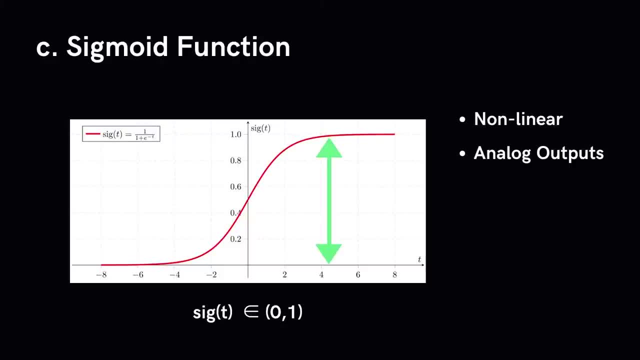 too, tend to have their share of disadvantages. If you look closely, between x is equal to negative 2 and x is equal to 2, the y values are very steep. Any small changes in the values of x in that region will cause values of y to change drastically. 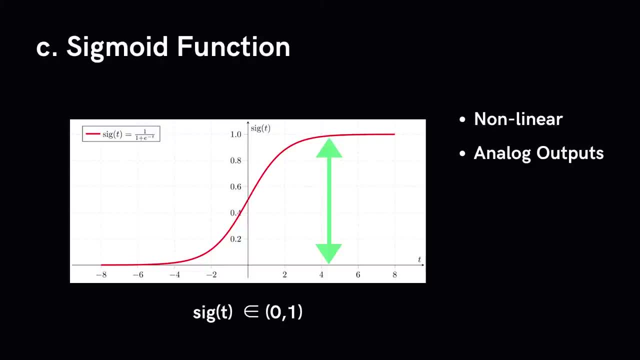 Also towards either end of the function. the y values tend to respond very less to changes in x. The gradient at those regions is going to be really, really small, Almost zero, And it gives rise to the vanishing gradient problem, Which just says that if the input to the activation 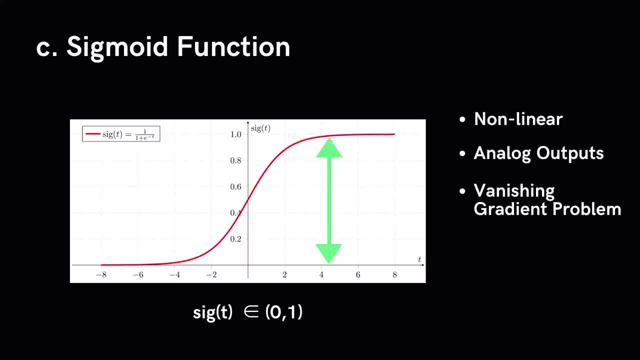 function is either large or small. the sigmoid is going to squish that down to a value between 0 and 1. And the gradient of this function becomes really small. And you will see why, when we talk about gradient descent, this is a huge problem. 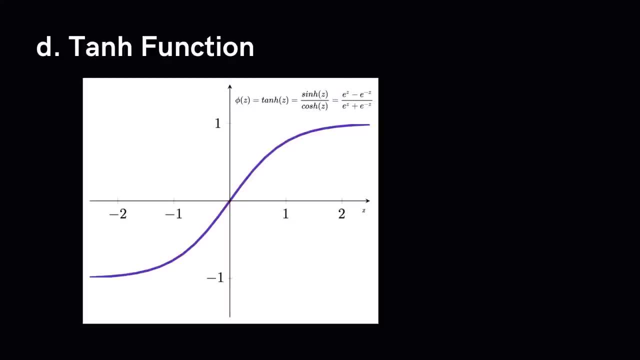 Another activation function that is used is the tanh function. This looks very similar to the sigmoid. In fact, mathematically this is what's known as a shifted sigmoid function. So, like the sigmoid, it has characteristics that we discussed above: It is non-linear. 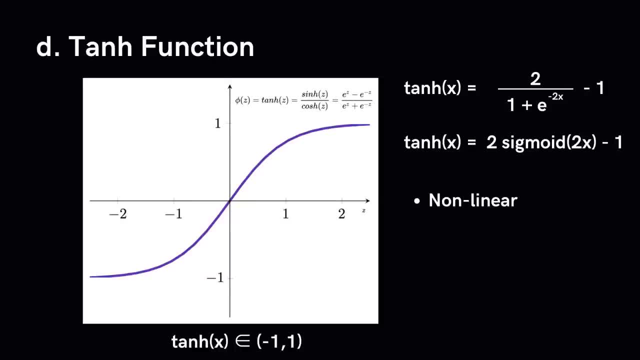 in nature so we can stack layers. It is bound to a range from negative 1 to 1, so there is no worrying about the activations blowing up. The derivative of the tanh function, however, is steeper than that of the sigmoid, So deciding. 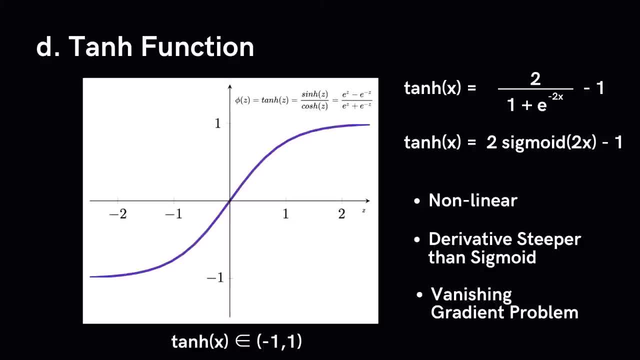 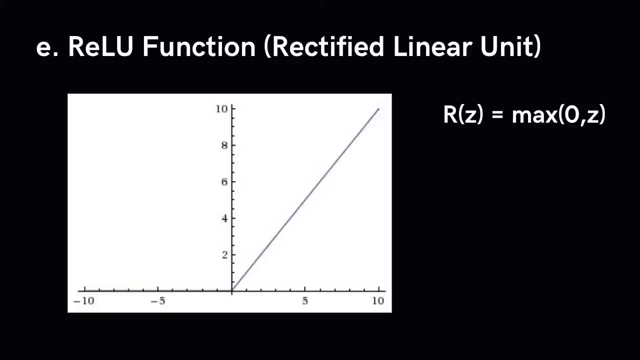 between the sigmoid and the tanh will really depend on your requirement of the gradient strength. Like sigmoid, tanh is also a very popular and widely used activation function and, yes, like the sigmoid tanh, does have the vanishing gradient problem. The rectified linear unit, or the ReLU function, is defined as a if x is equal to the max from. 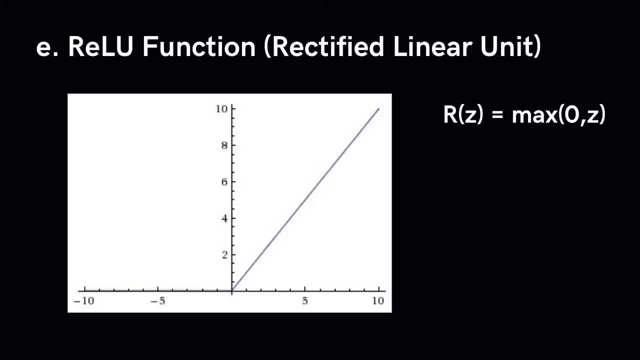 0 to x. At first look, this would look like a linear function. right, The graph is linear in the positive axis. Let me tell you, ReLU is in fact, non-linear in nature and combinations of ReLU are also non-linear- Great. so this means that we can stack layers. 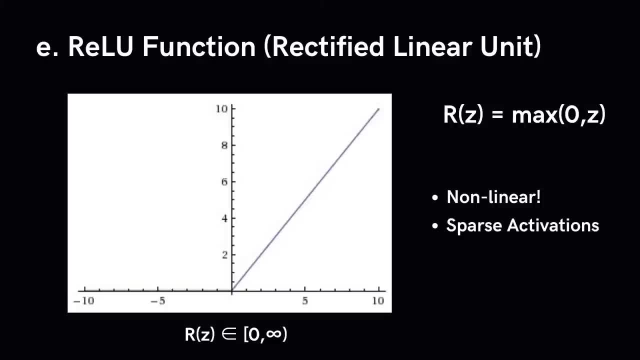 However, unlike the previous two functions that we discussed, it is not bounded. The range of the ReLU is from 0 to infinity. This means there is a chance of blowing up the activation. Another point that I would like to discuss here is the sparsity of an activation. Imagine. 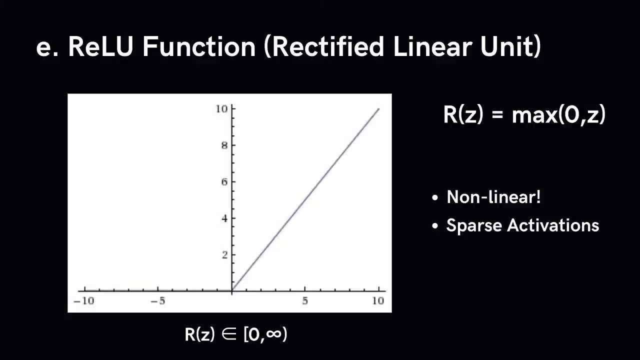 a big neural network with lots of neurons. Using a sigmoid or a tanh will cause almost all the neurons to fire in an analog way. This means that almost all activations will be processed to describe the networks output. This means that almost all activations will 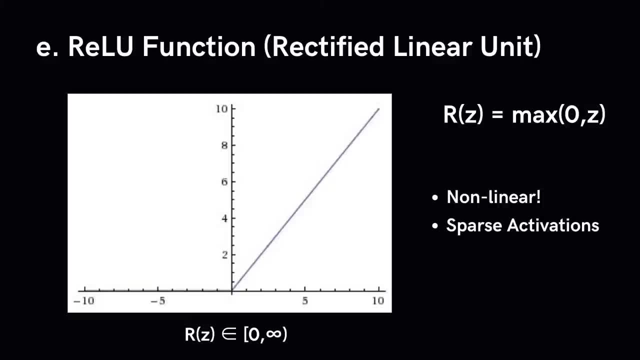 be processed to describe the networks output. In other words, the activation would be dense, And this is costly. Ideally, we want only a few neurons in the network to activate and thereby making the activation sparse and efficient. Here's where the ReLU comes in. 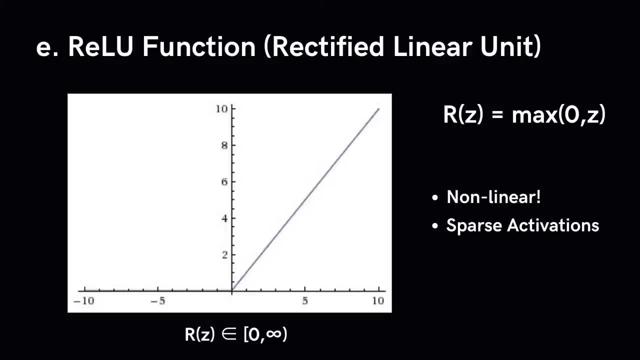 Imagine a network with randomly initialized weights and almost 50% of the network yields zero activation. Because of the characteristic of ReLU, it outputs zero for negative values of x. This means that only 50% of the neurons fire sparse activation, making the network lighter. 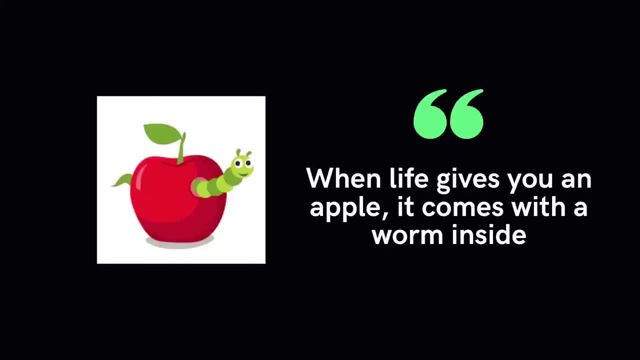 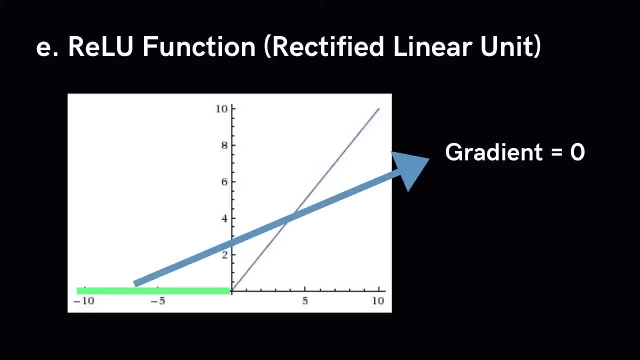 But when life gives you an apple, it comes with a little worm inside. Because of that horizontal line in ReLU for negative values of x the gradient is zero in that region, Which means that during backpropagation the weights will not get adjusted during descent. 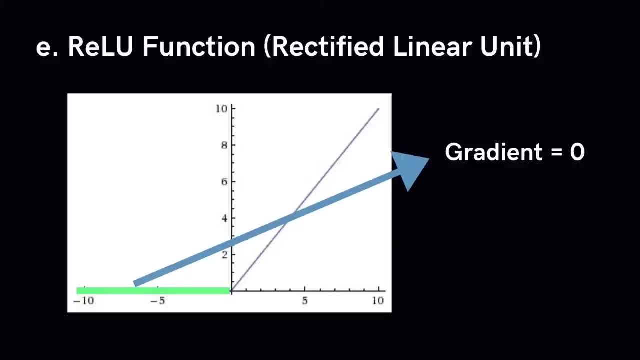 This means that those neurons which go into that state will stop responding to variations in the error. simply because the gradient is zero, nothing changes. This is called the dying ReLU problem. This problem can cause several neurons to just die and not respond, thus making a substantial 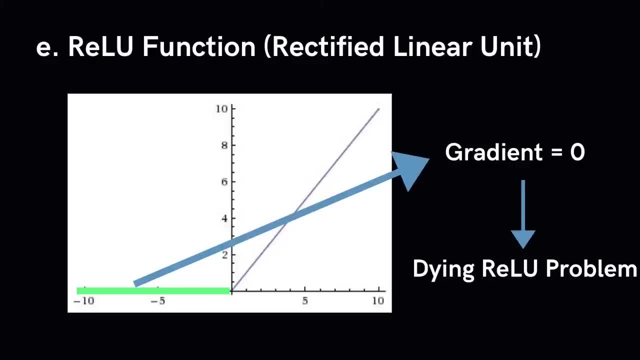 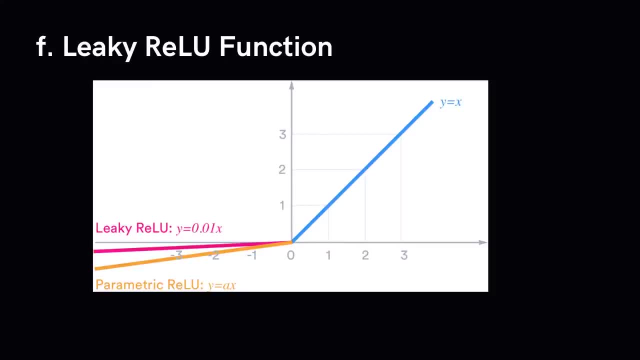 part of the network passive rather than what we want, active. There are workarounds for this. one way, especially, is to simply make the horizontal line into a non-horizontal component by adding a slope. Usually, the slope is around 0.001.. 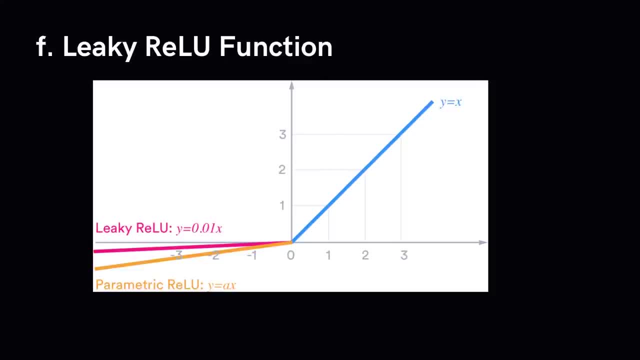 And this new version of the ReLU is called the leaky ReLU. The main idea is that the gradient should never be zero. One major advantage of the ReLU is the fact that it's less computationally expensive than functions like tanh and sigmoid, because it involves simpler mathematical operations. 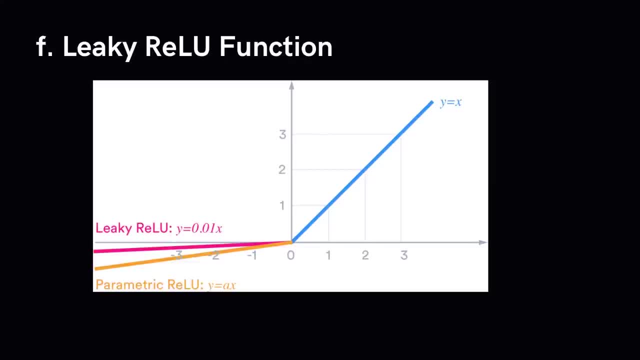 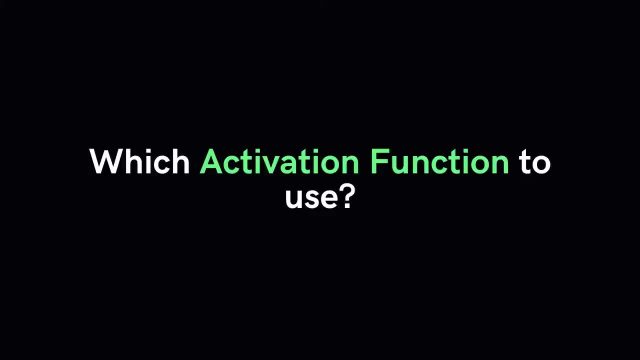 This is a really good point to consider when you are designing your own deep neural networks. Great, so now the question is which activation function to use Because of the advantages that ReLU offers. does this mean that you should use ReLU for everything you do? 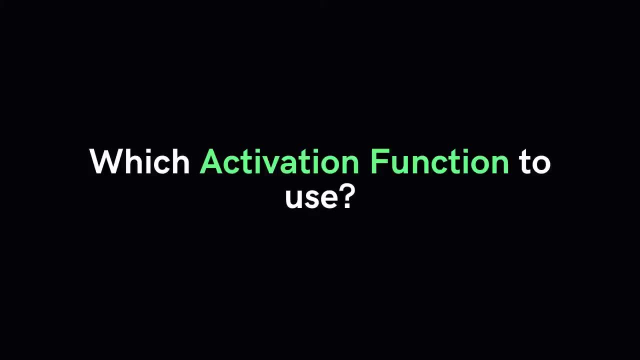 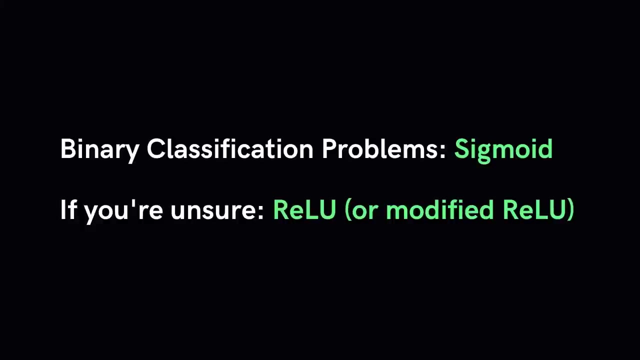 Or could you consider sigmoid and tanh Well, both. When you know the function that you're trying to approximate has certain characteristics, you should choose an activation function which will approximate the function faster, leading to faster training processes. For example, a sigmoid function works well for binary classification problems because 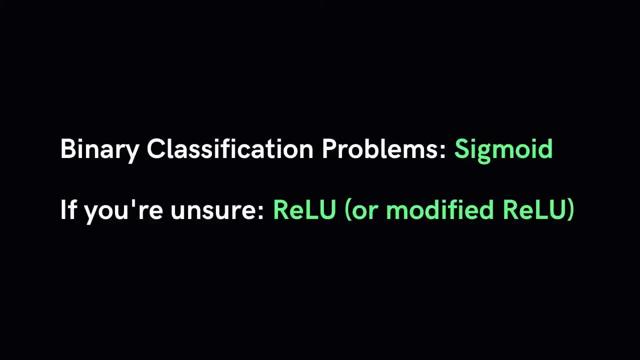 approximating or classifying functions as combinations of the sigmoid is easier than maybe the ReLU. This will lead to faster training processes and larger convergence. You can use your own custom functions too. if you don't know the nature of the function you're trying to learn, I would suggest you start with ReLU and then work backwards. 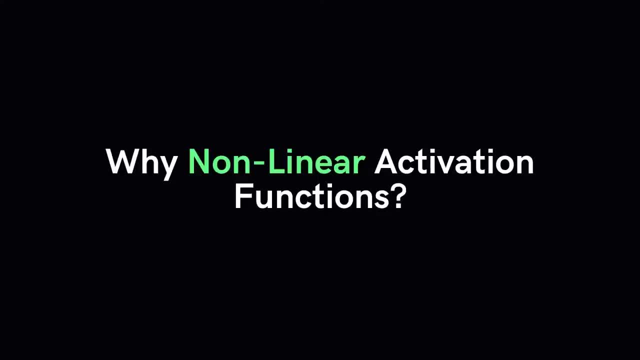 from there. Before we move on to the next section, I want to talk about why we use non-linear activation functions as opposed to linear ones. If you recall, in my definition of activation functions I mentioned that activation functions serve to introduce something called non-linearity in the network. 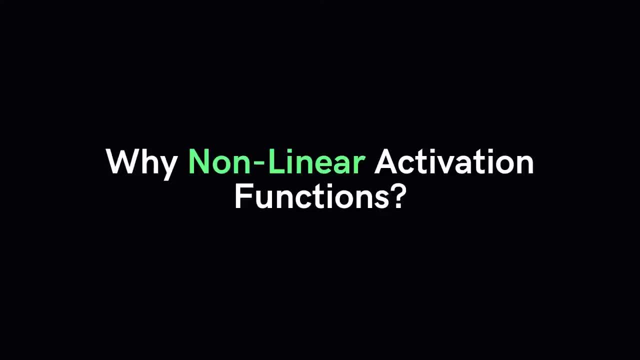 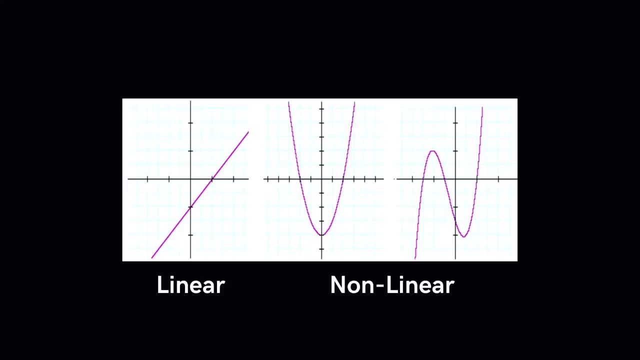 For all intents and purposes, introducing non-linearity simply means that your activation function must be non-linear. That is not a straight line. Mathematically linear functions are polynomials of degree 1, that, when graphed in the xy-plane. 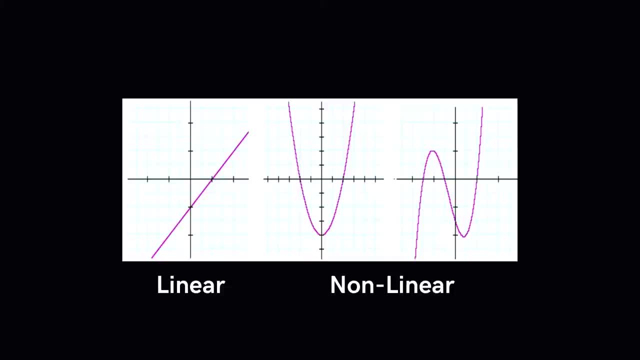 are straight lines inclined to the x-axis at a certain value. We call this the slope of the line. Non-linear functions are polynomials of degree greater than 1, and when graphed they don't form straight lines, rather they're more curved. 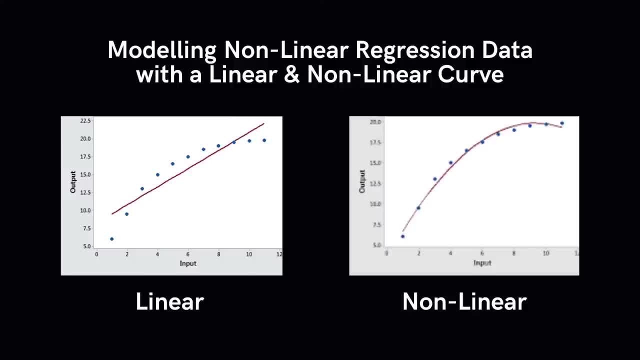 If we use linear activation functions to model our data, then no matter how many hidden layers our network has, it will always become equivalent to having a single-layer network. In deep learning, we want to be able to model every type of data without being restricted. 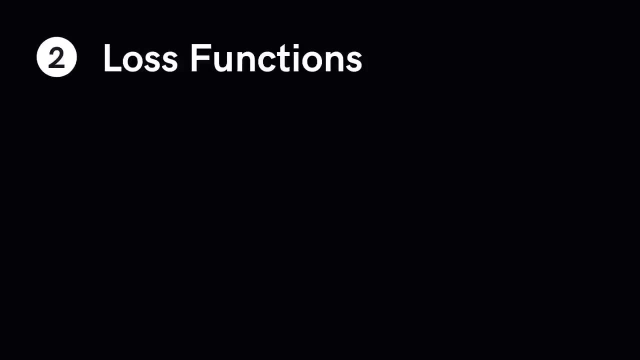 as would be the case should we use linear functions? We've discussed previously in the learning process of neural networks that we started with random weights and biases. The neural network makes a prediction. this prediction is compared against the expected output and the weights and biases are adjusted accordingly. 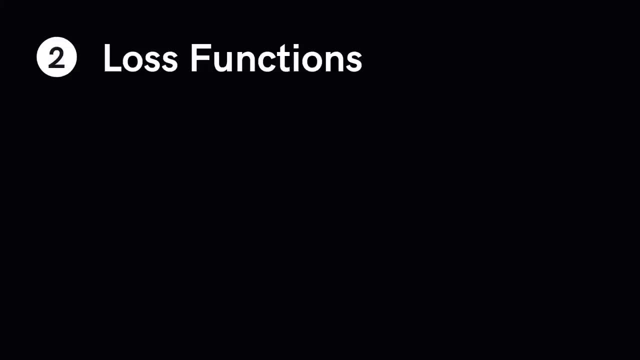 Well, loss functions are the reason that we're able to calculate that difference Really simply. A loss function is a way to quantify the deviation of the predicted output by the neural network to the expected output. It's as simple as that. nothing more, nothing less. 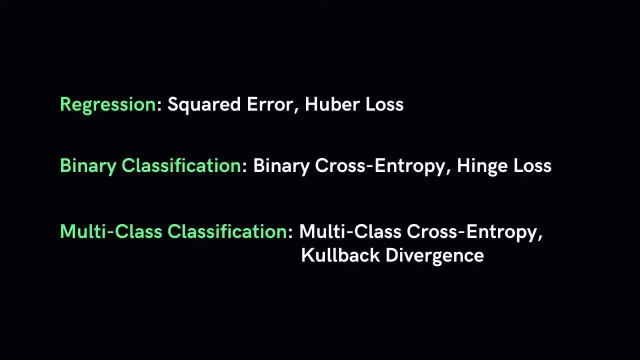 There are plenty of loss functions out there. for example, under regression we have squared error loss, absolute error loss and Huber loss. In binary classification we have binary cross entropy and hinge loss. In multiclass classification problems we have the multiclass cross entropy and the 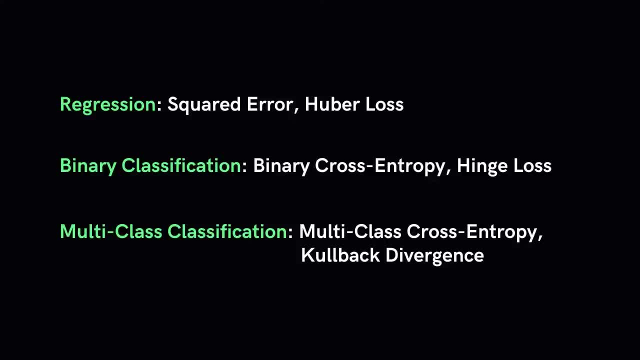 callback-liable, divergence loss and so on. The choice of the best function really depends on what kind of project you're working on. Different projects require different loss functions. Now I don't want to talk any further on loss functions right now. we'll do this under the 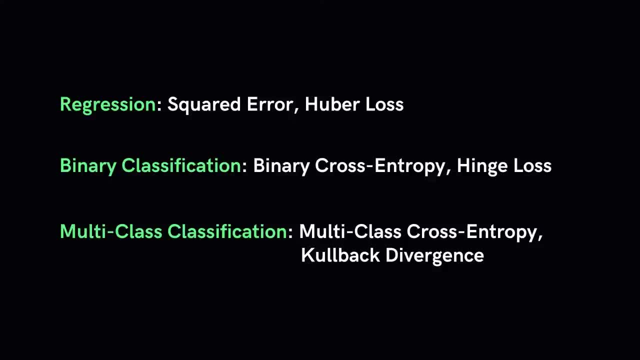 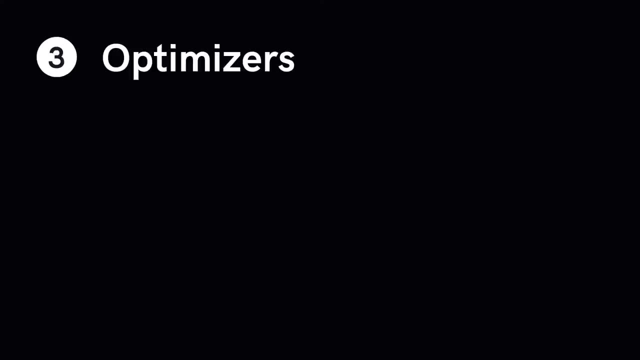 optimization section, because that's really where loss functions are utilized. In the previous section we dealt with loss functions, which are mathematical ways of measuring how wrong predictions made by a neural network are. During the training process, we tweak and change the parameters of the weights of the 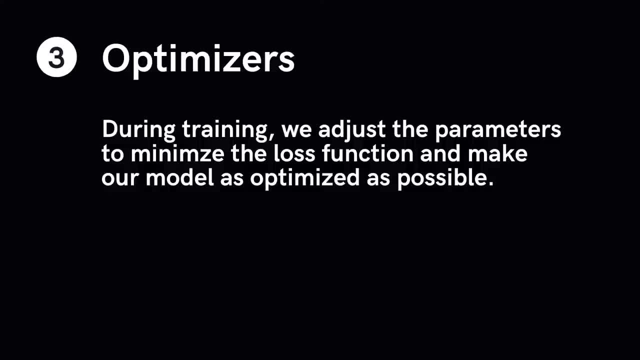 model to try and minimize the loss function and make our predictions as correct and optimized as possible. But how exactly do you do that? How do you change the parameters of your model? by how much and when? We have the ingredients, how do we make the cake? 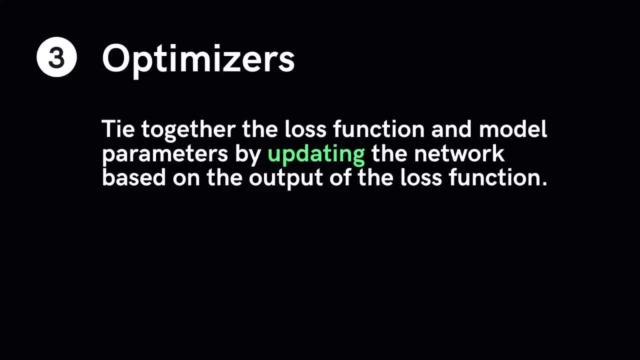 This is where optimizers come in. They tie together the loss function and the model parameters, or the weights and biases, by updating the network in response to the output of the loss function. In simpler terms, and mold your model into more accurate models by adjusting the weights and the 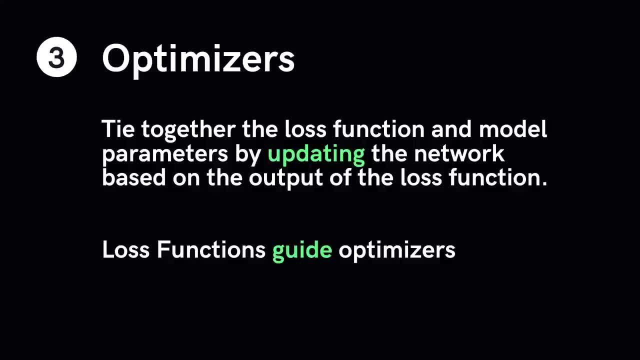 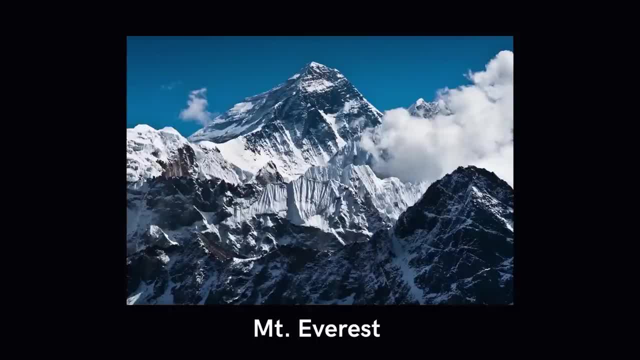 biases. The loss function is its guide. It tells the optimizer whether it's moving the right or the wrong direction. To understand this better, imagine that you have just scaled Mount Everest and now you decide to descend the mountain blindfolded. It's impossible to know which direction to go in. You could 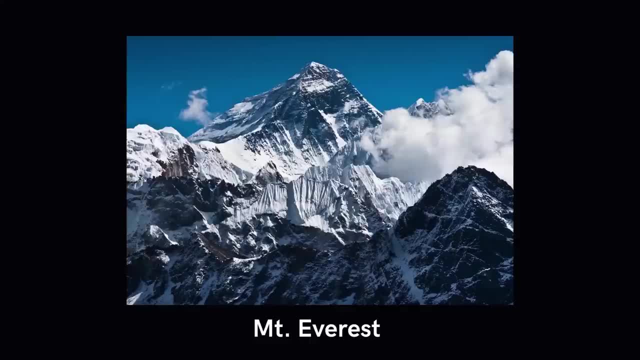 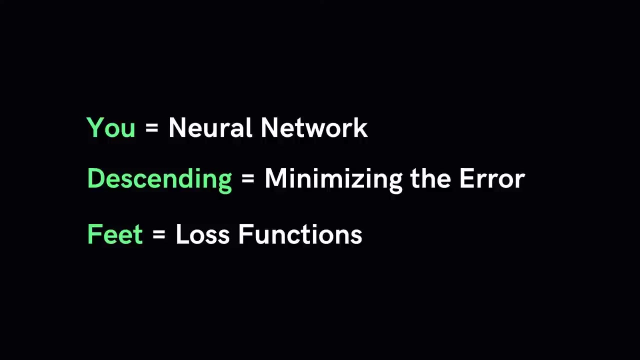 either go up, which is away from your goal, or go down, which is towards your goal. But to begin, you would start taking steps. Using your feet, you'll be able to gauge whether you're going up or down. In this analogy, you resemble the neural network. Going down your goal is trying to minimize the error and your 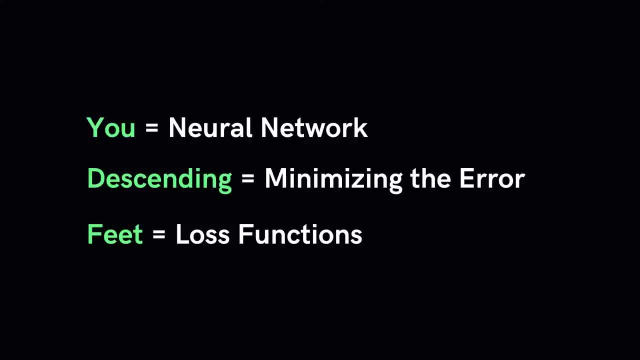 feet are resemblant of the loss functions. They measure whether you're going in the right way or the wrong way. Similarly, it's impossible to know what your model's weights should be right from the start. But with some trial and error based on the loss function, you could end up. 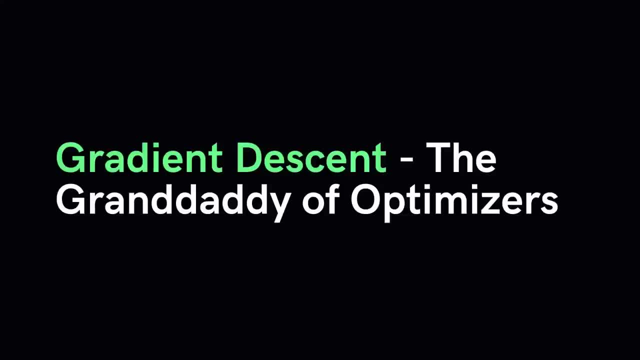 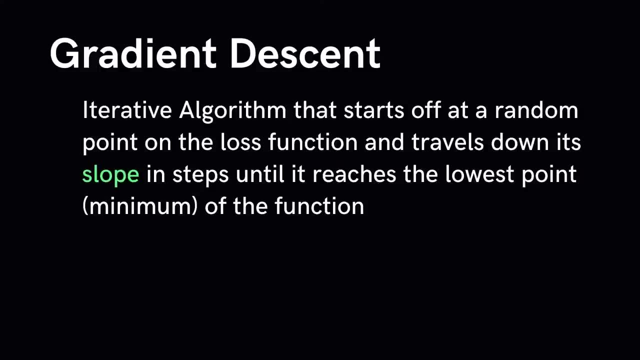 getting there eventually. We now come to gradient descent, often called the granddaddy of optimizers. Gradient descent is an iterative algorithm that starts off at a random point in the loss function and travels down its slope in steps until it reaches the lowest point or the minimum of the function. It is the. 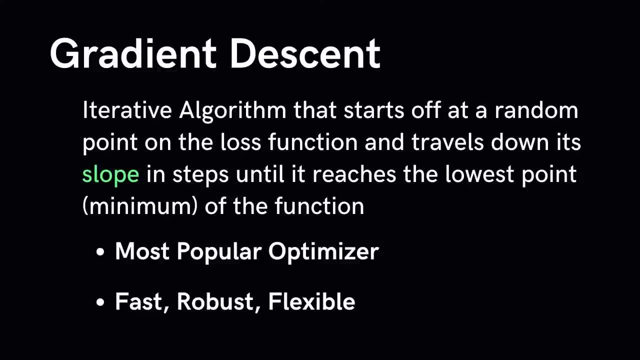 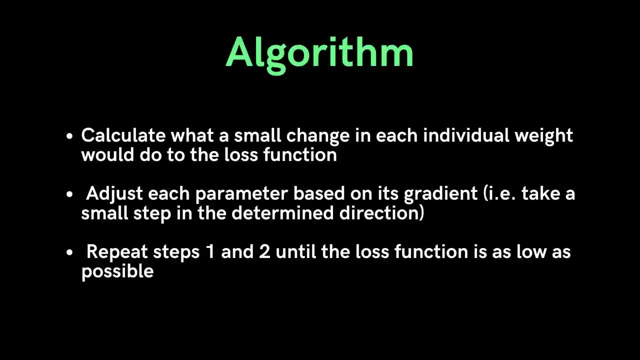 most popular optimizer we use nowadays. It's fast, robust and flexible. And here's how it works. First we calculated what a small change in each individual weight would do to the loss function. We then calculated the weight of the loss function. We adjust each individual weight based on its gradient. that is, take a small. 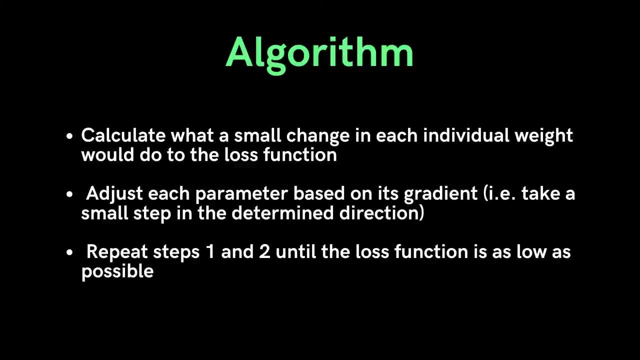 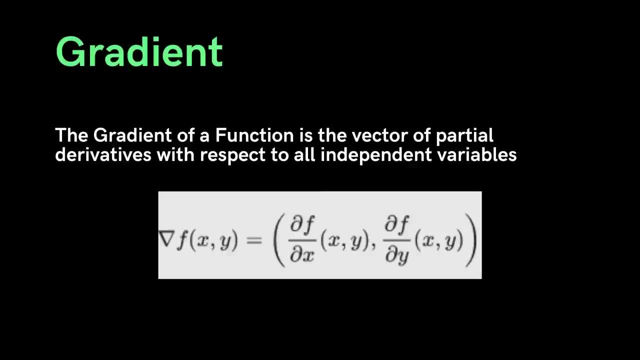 step in the determined direction. The last step is to repeat the first and the second step until the loss function gets as low as possible. I want to talk about this notion of a gradient. The gradient of a function is the vector of the partial derivatives with respect to all independent 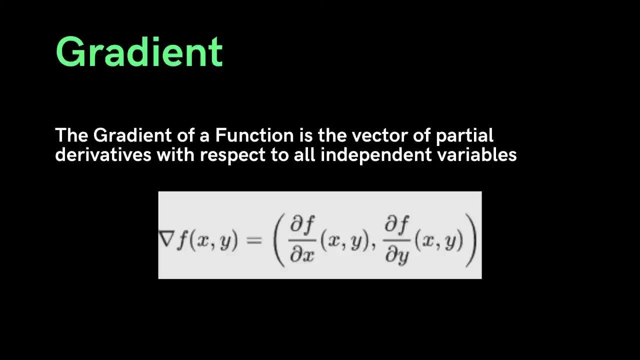 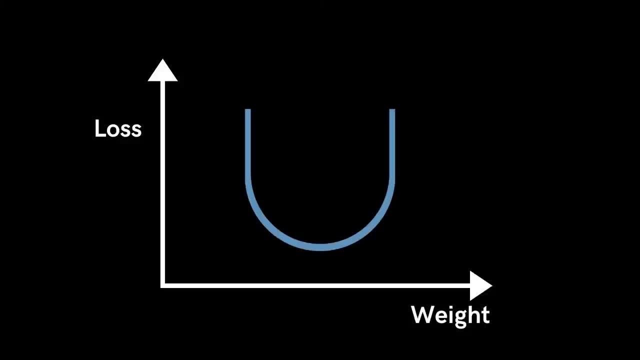 variables. The gradient always points in the direction of the steepest increase in the function. Suppose we have a graph like so, with loss on the y-axis and the value of the weight on the x-axis. We have a little data point here that 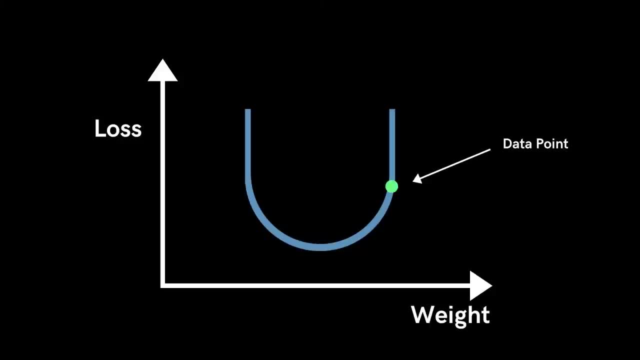 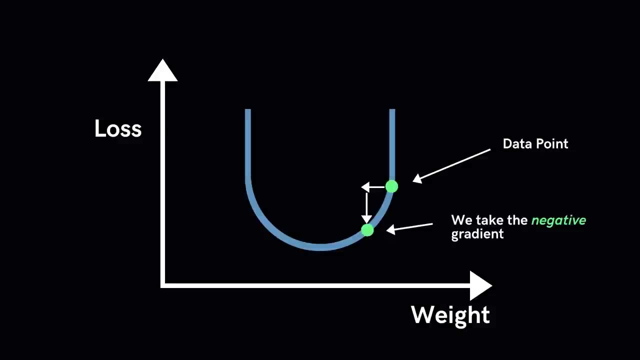 corresponds to the randomly initialized weight. To minimize this loss, that is, to get this data point to the minimum of the function, we need to take the negative gradient, since we want to find the steepest decrease in the function. This process happens iteratively. 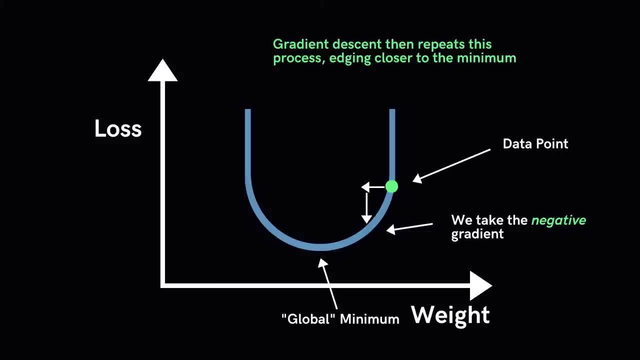 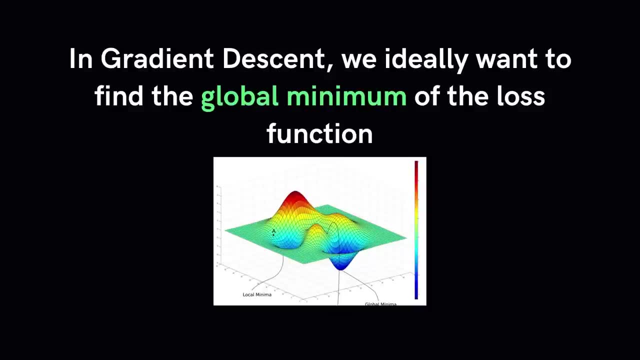 till, the loss is as minimized as possible. That's gradient descent in a nutshell. When dealing with high dimensional datasets, that is lots of variables- it's possible you'll find yourself in an area where it seems like you've reached the lowest possible value for your loss function, but in reality it's just a local minimum To avoid getting 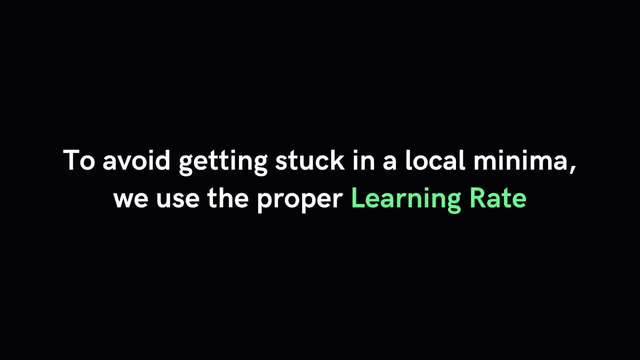 stuck in a local minimum. we make sure we use a proper learning rate. Changing our weights too fast by adding or subtracting too much- that is, taking steps that are too large or too small- can hinder your ability to minimize the loss function We don't want to make. 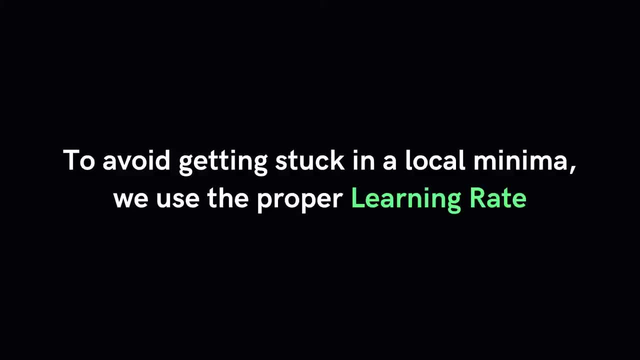 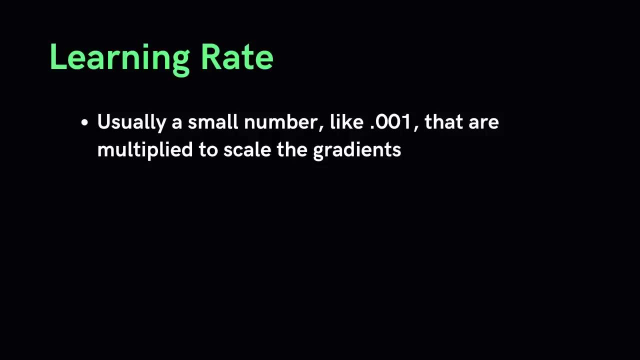 a jump so large that we skip over the optimal value for a given weight. To make sure this doesn't happen, we use a variable called the learning rate. This thing is usually just a small number like .001, that we multiply the gradient by to. 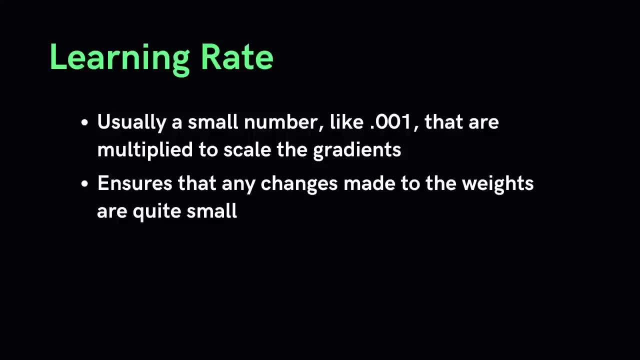 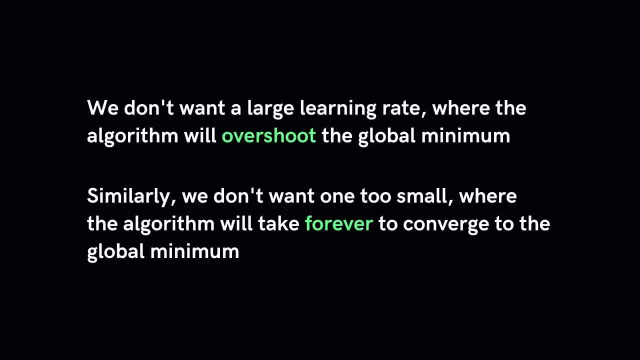 scale them. This ensures that any changes we make to our weights are pretty small. In math talk, taking steps that are too large can mean that the algorithm will never converge to an optimum. At the same time, we don't want to take steps that are too small because 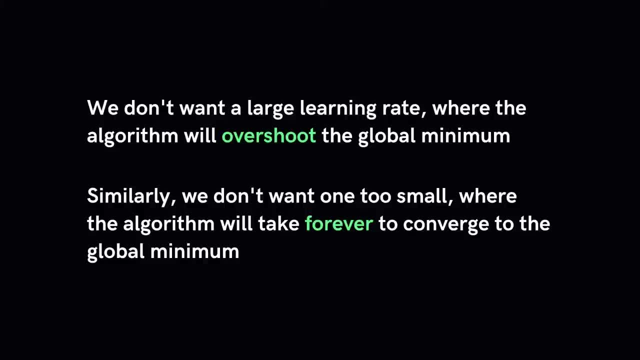 then we might never end up with the right values for our weights. In math talk, steps that are too small might lead to our optimizer converging on a local minimum for the loss function whenever the absolute minimum. For a simple summary, just remember that the learning 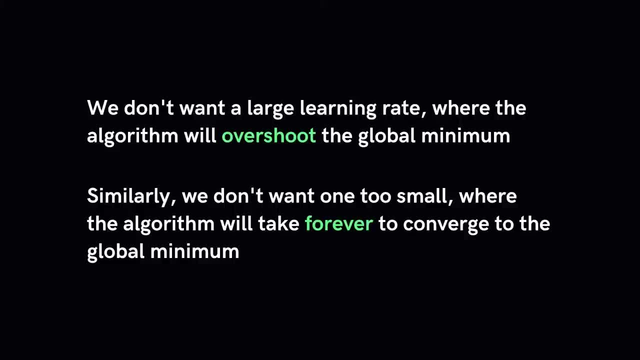 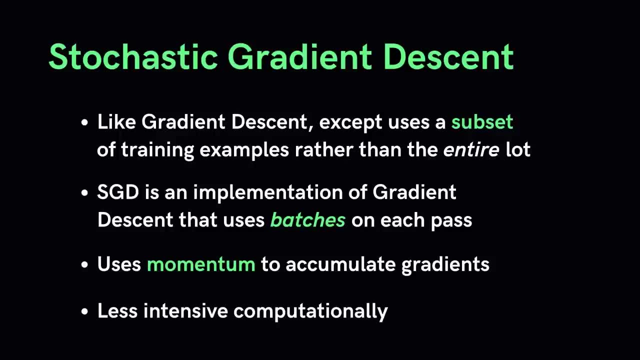 rate ensures that we change our weights at the right pace, not making any changes that are too big or too small. Instead of calculating the gradients for all your training examples on every pass of the gradient descent, it's sometimes more efficient to only use a subset. 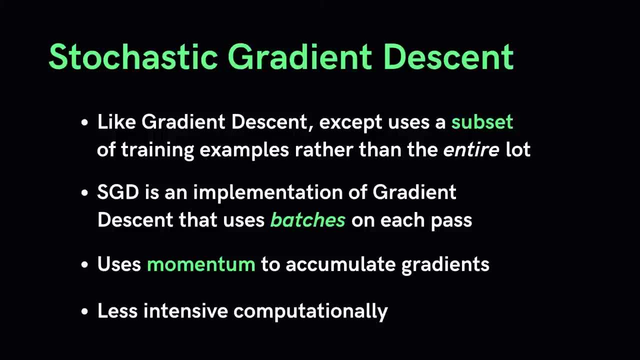 of the training examples each time. Stochastic gradient descent is an implementation that either uses batches of examples at a time or random examples on each pass. Stochastic gradient descent uses the concept of momentum. Momentum accumulates the gradients of the past steps to dictate what might happen in the next steps. Also, because we don't include 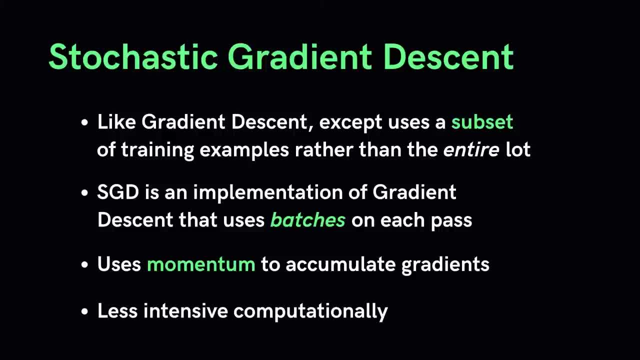 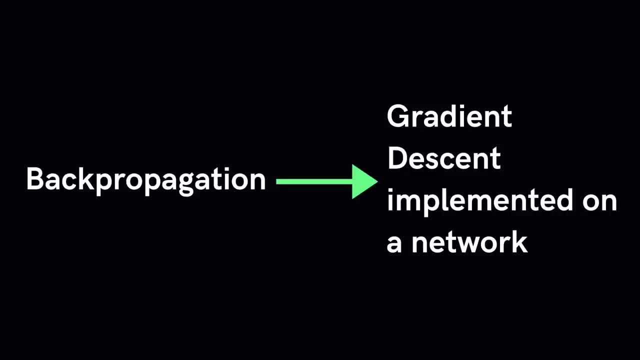 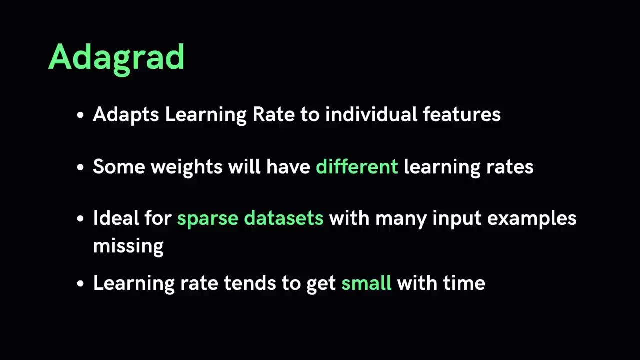 the entire training set. SGD is less computationally expensive. It's difficult to overstate how popular gradient descent really is. Backpropagation is basically gradient descent implemented on a network. Adagrad adapts the learning rate specifically to individual features. That means that some 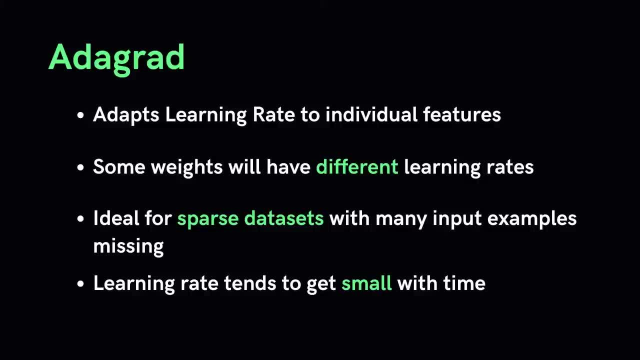 of the weights in your dataset will have different learning rates than others. This works really well for sparse datasets where a lot of input examples are missing. Adagrad has a major issue, though. The adaptive learning rate tends to get really, really small over time. 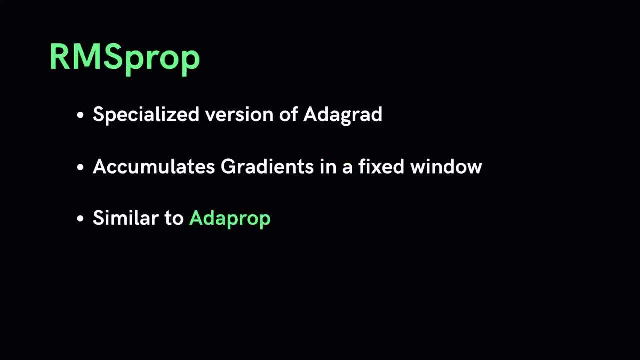 RMSProp is a special version of Adagrad developed by Professor Geoffrey Hinton. Instead of letting all the gradients of the gradient descent be the same, you can use it to calculate the gradients of the previous gradients. If the gradients accumulate for momentum, it accumulates gradients in a fixed window. 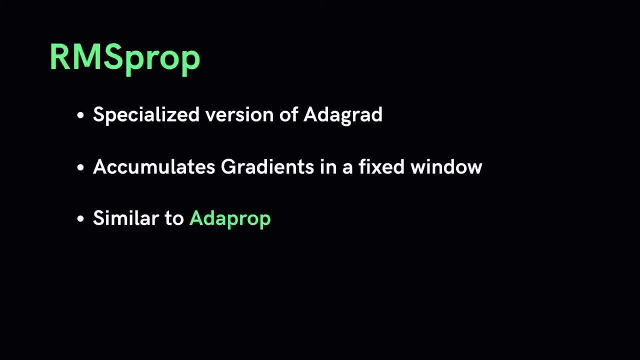 RMSProp is similar to Adaprop, which is another optimizer that seeks to solve some of the issues that Adagrad leaves open. ADAM stands for Adaptive Moment Estimation and is another way of using past gradients to calculate the current gradient. 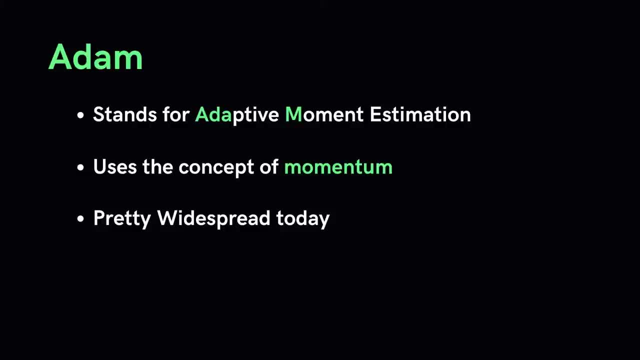 ADAM also utilizes the concept of momentum, which is basically our way of telling the neural network whether we want past changes to affect the new change by adding fractions of the previous gradients to the current one. This optimizer has become pretty widespread and is practically accepted for use in training. 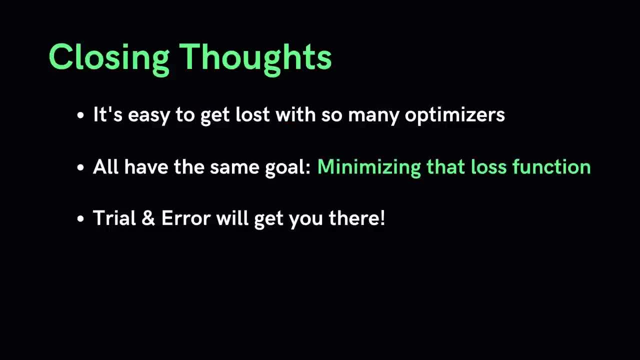 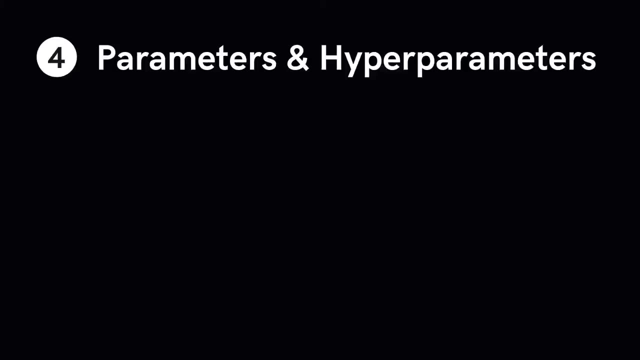 neural networks. It's easy to get lost in the complexity of some of these new optimizers. Just remember that they all have the same goal: minimizing the loss function, And trial and error will get you there. You may have heard me referring to the word parameters quite a bit, and often this word 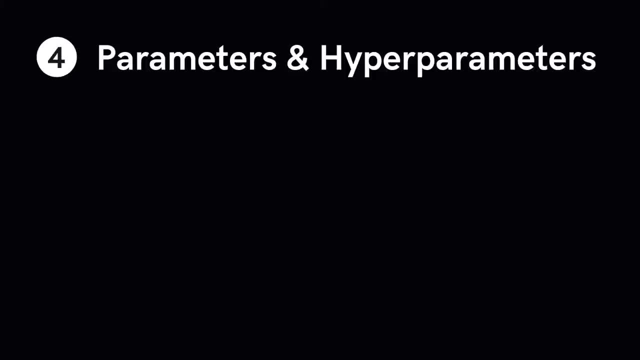 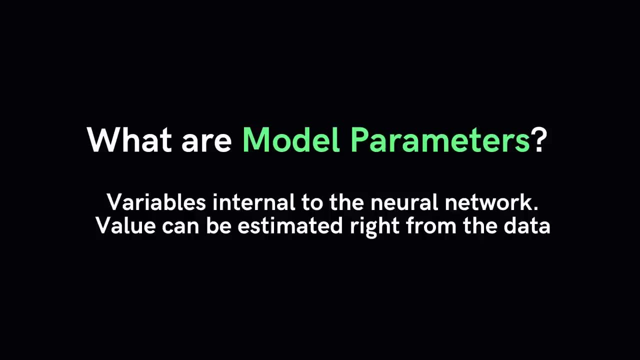 is confused with the term hyperparameters. In this video, I'm going to talk about hyperparameters. Let's get started. In this video, I'm going to outline the basic difference between the two. A model parameter is a variable that is internal to the neural network and whose values can 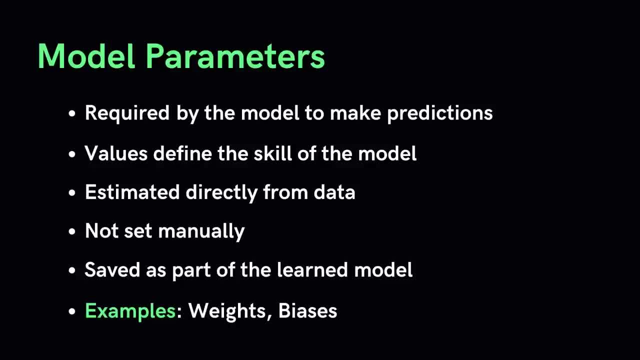 be estimated from the data itself. They are required by the model when making predictions. These values define the skill of the model on your problem. They can be estimated directly from the data and are often not manually set by the practitioner And often times when you save your model, you are essentially saving your model. 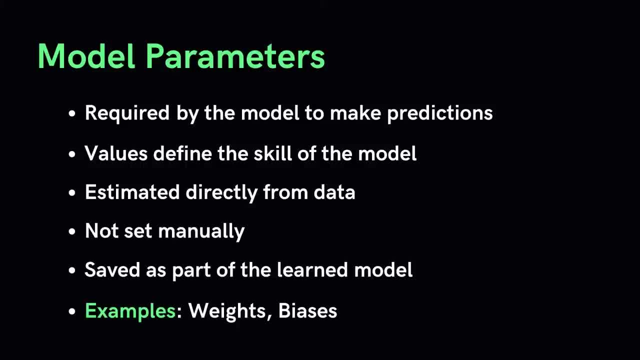 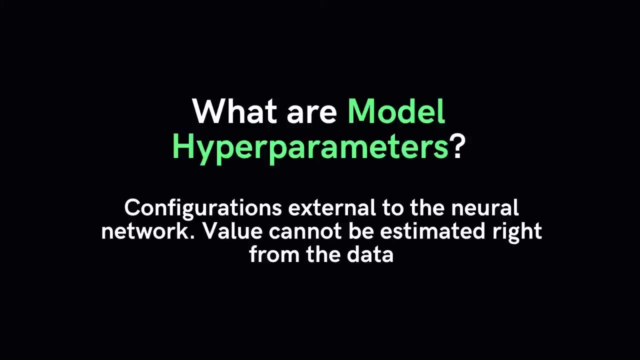 So let's get started. In this video, I'm going to outline the basic difference between the two. A hyperparameter is a configuration that is external to the model and whose value cannot be estimated from data. There is no way that we can find the best value for a model hyperparameter on a given 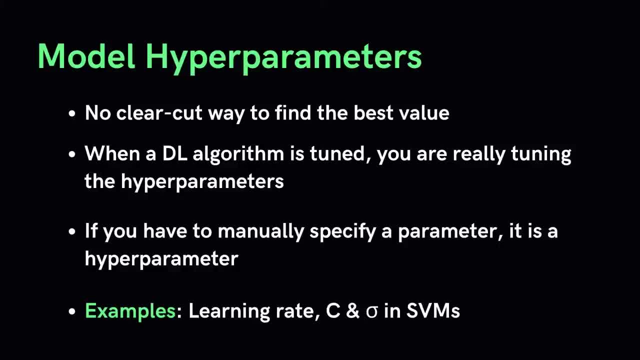 problem. We may use rules of thumb, copy values used in other problems or search for the best value by trial and error. In this video, I'm going to outline the basic difference between the two. When a machine learning algorithm is tuned for a specific problem, such as when you're. 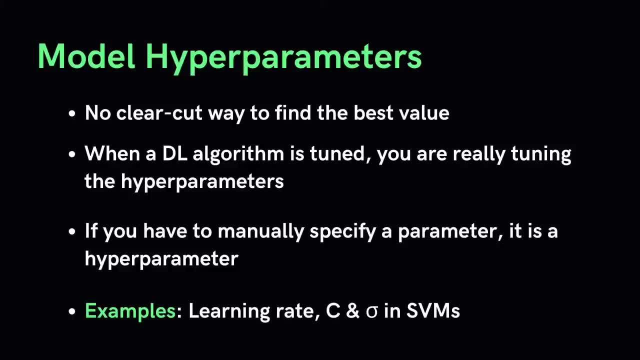 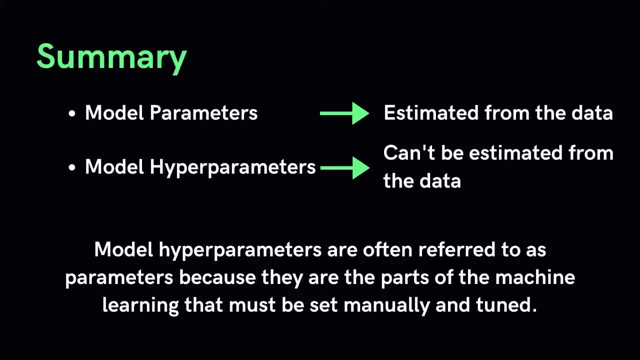 using grid search or random search, then you are in fact tuning the hyperparameters of the model in order to discover the parameters that result in more skillful predictions. Model hyperparameters are often referred to as parameters, which can make things confusing, So a good rule of thumb to overcome this confusion is as follows. 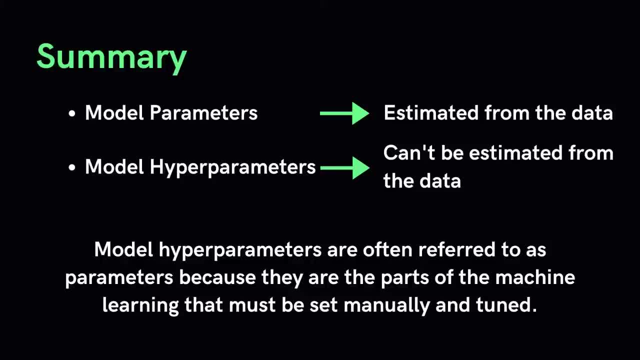 If you have to specify a parameter manually, then it is probably a hyperparameter. The parameters are inherent to the model itself. Some examples of hyperparameters include the learning rate for training a neural network, the C and sigma hyperparameters for support vector machines and the k and k-nearest neighbors. 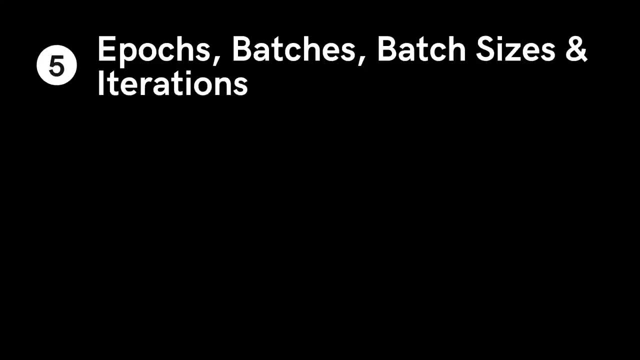 We need terminologies like epochs, batch size and iterations only when the data is too big, which happens all the time in machine learning, and when we can't pass all this data to the computer at once. So to overcome this problem, we need to use a machine learning algorithm. 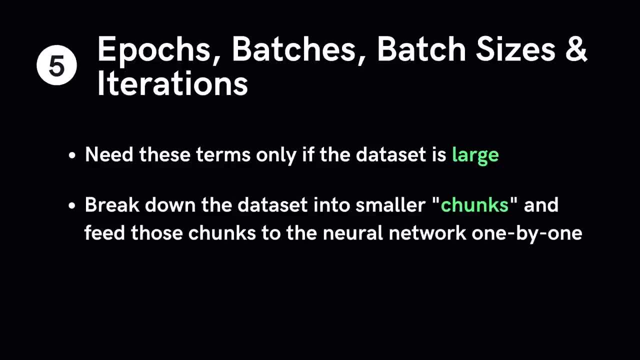 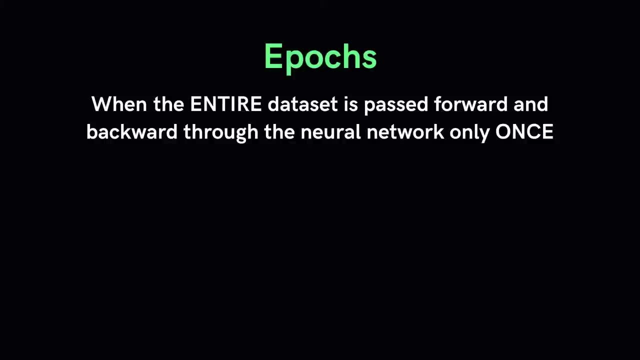 To overcome this problem, we need to divide the dataset into smaller chunks, give it to our computer one by one and update the weights of the neural network at the end of every step to fit it into the data given. One epoch is when an entire dataset is passed forward and backward through the network once. 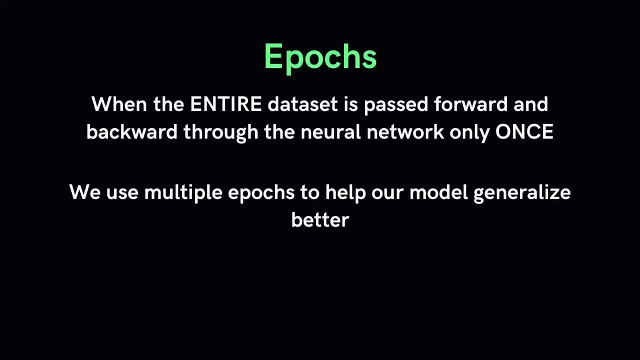 In a majority of deep learning models we use more than one epoch. I know it does make sense in the beginning. why do we need to pass the entire dataset many times through the same neural network? It's not enough to pass the entire dataset through the network only once it's trying. 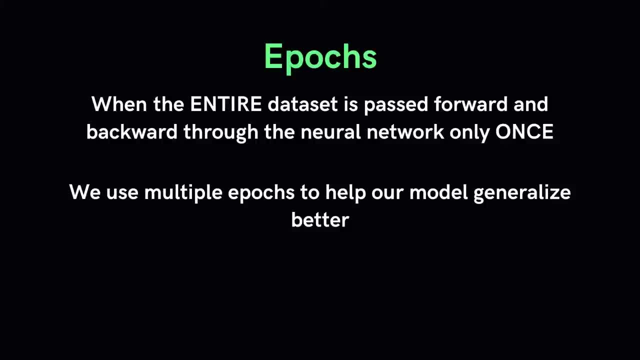 to read the entire lyrics of a song. once You won't be able to remember the entire song immediately, you'd have to re-read the lyrics a couple more times before you can say you know the song by memory. The same is true with the neural network. 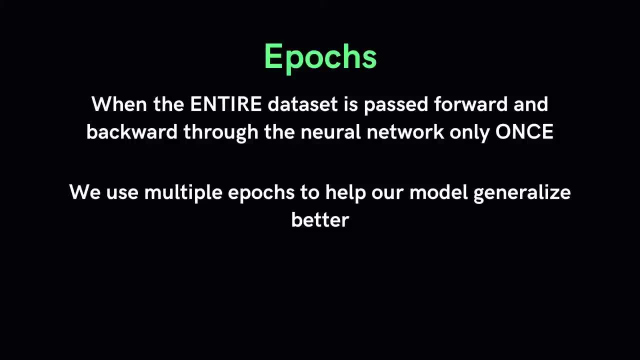 We pass the dataset multiple times through the neural network so it's able to generalize better. Gradient descent is an iterative process, and updating the parameters and backpropagation in a single pass or one epoch is not enough. The more epochs increases, the more the parameters are adjusted, leading to a better performing. 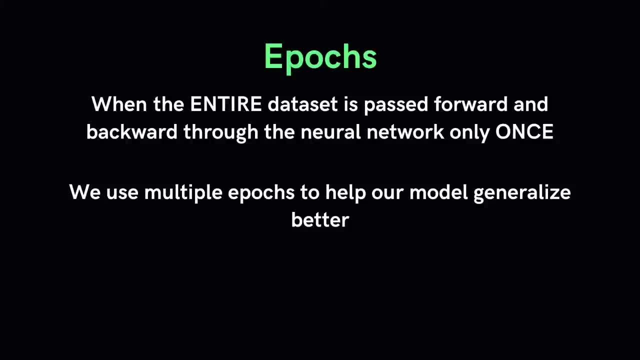 model. But too many epochs could spell disaster and lead to something called overfitting, where a model has essentially memorized the patterns in the training data and performs terribly on data it's never seen before. So what is the right number of epochs? 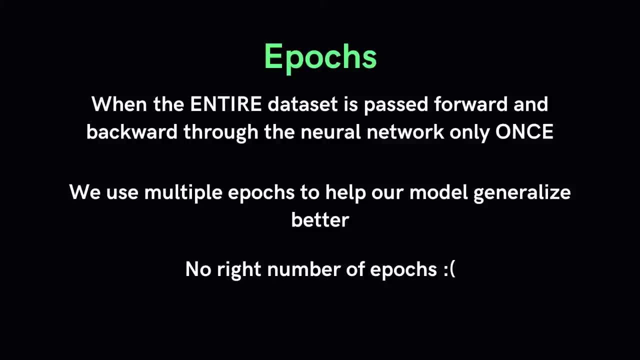 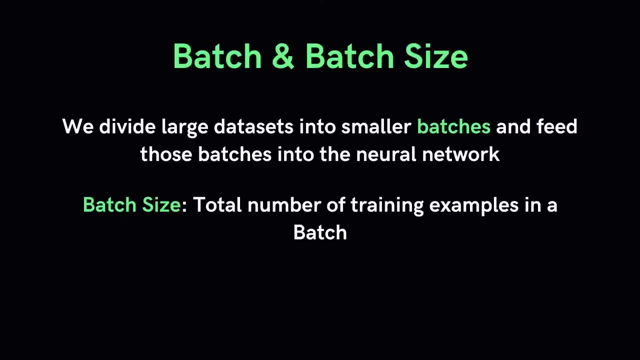 Unfortunately, there is no right answer. The answer is different for different datasets. Sometimes your dataset can include millions of examples. Passing this entire dataset at once becomes extremely difficult, so what we do instead is divide the dataset into a number of batches, rather than passing the entire dataset once. 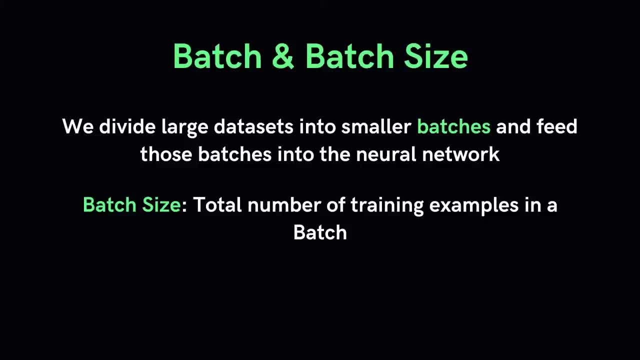 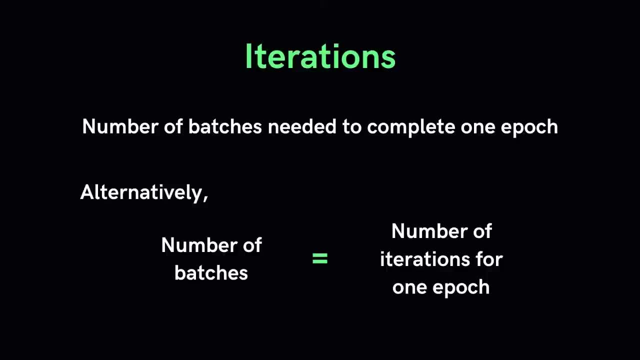 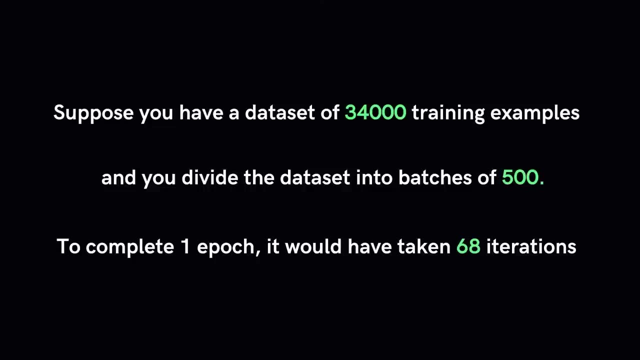 The total number of training examples present in a single batch is called a batch size. Iterations is the number of batches needed to complete one epoch. Note: the number of batches is equal to the number of iterations for one epoch. Let's say that we have a dataset of 34,000 training examples. 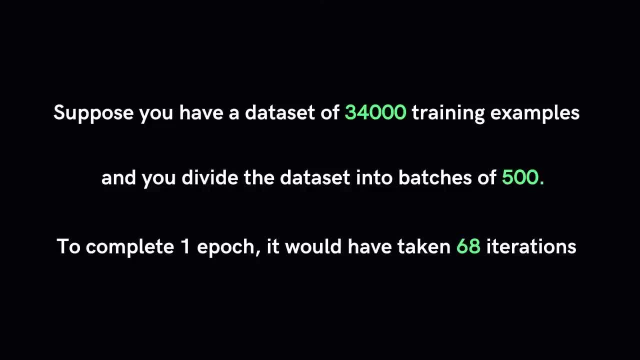 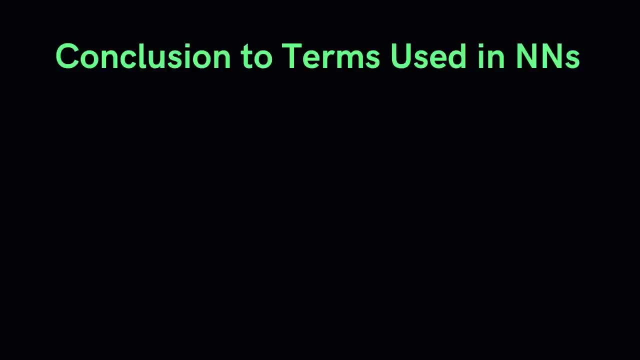 The number of batches is equal to the number of iterations for one epoch. If we divide the dataset into batches of 500, then it will take 68 iterations to complete one epoch. Well, I hope that gives you some kind of sense about the very basic terminologies used in. 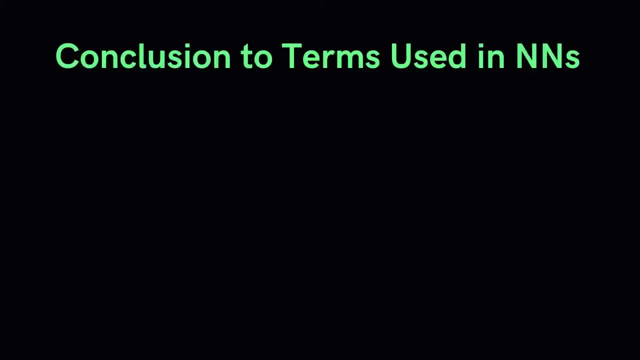 deep learning. Before we move on, I do want to mention this, and you will see this a lot in deep learning- You will often have a bunch of different choices to make. How many hidden layers should I choose, or which activation function must I use and where? 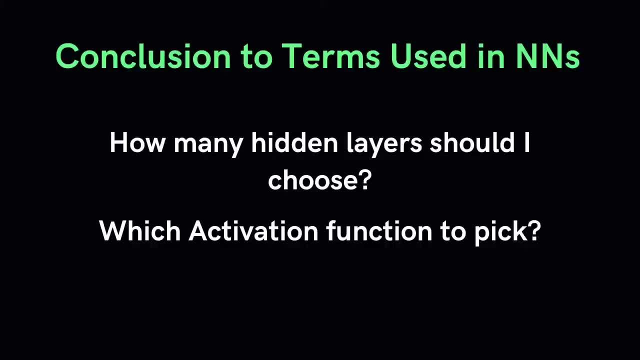 This is a fun part about deep learning. it's extremely difficult to know in the beginning what's the right combination to use for your project. What works for me might not work for you, And a suggestion from my end would be that you dabble along with the material shown. 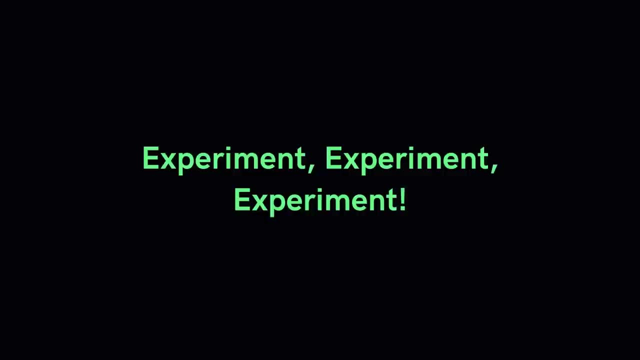 Try various combinations and see what works for you best. Ultimately, that's the learning process pun intended. Throughout this course, I'll give you quite a bit of intuition as to what's popular, so that, when it comes to building a deep learning project, you'll be able to get the most out. 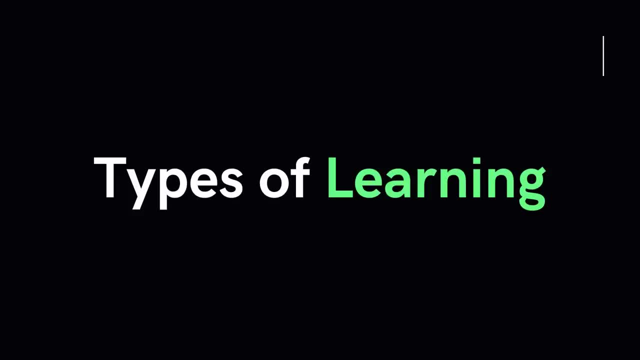 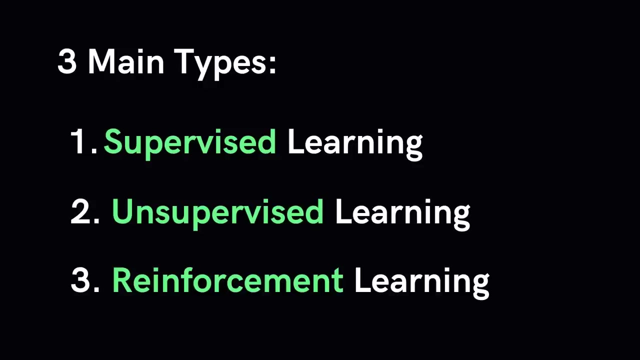 of it, You won't find yourself lost. In this section we're going to talk about the different types of learning, which are machine learning concepts but are extended to deep learning as well. In this course, we'll go over supervised learning, unsupervised learning and reinforcement. 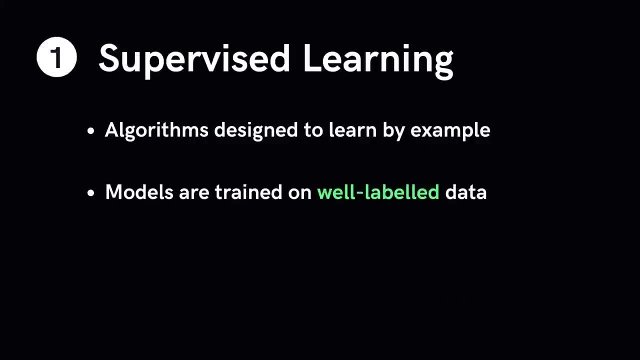 learning. Supervised learning is the most common sub-branch of machine learning today. Typically, if you're new to machine learning, your journey will begin with supervised learning algorithms. Let's explore why Supervised machine learning algorithms are designed to learn by example. 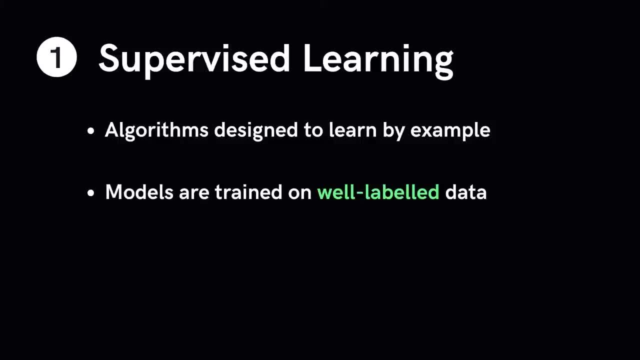 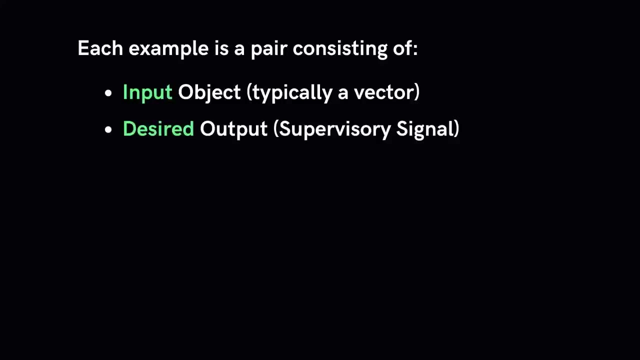 The name supervised learning originates from the idea that training this type of algorithm is almost like there's a human supervising the whole process. In supervised learning, we train our models on well-labeled data. Each example is a pair consisting of an input object, which is typically a vector, and a 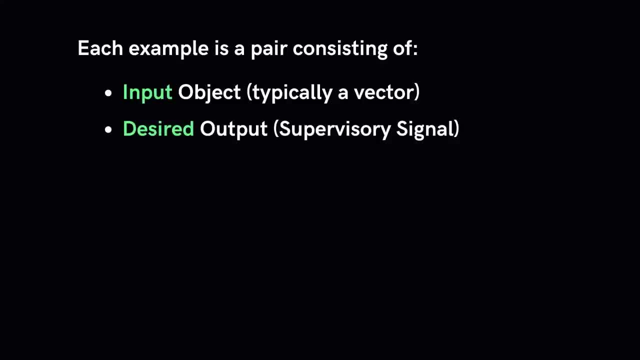 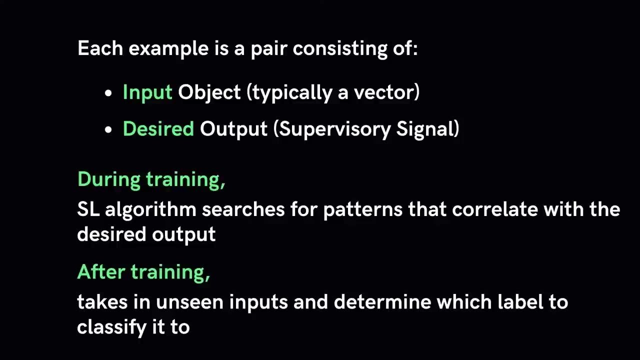 desired output value, also called a supervisory signal. During training, A supervised learning algorithm will search for patterns in the data that correlate with the desired outputs. After training, it will take in new unseen inputs and will determine which label the new inputs will be classified as, based on prior training data. 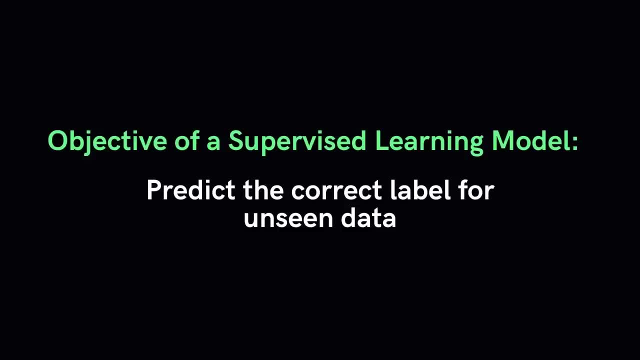 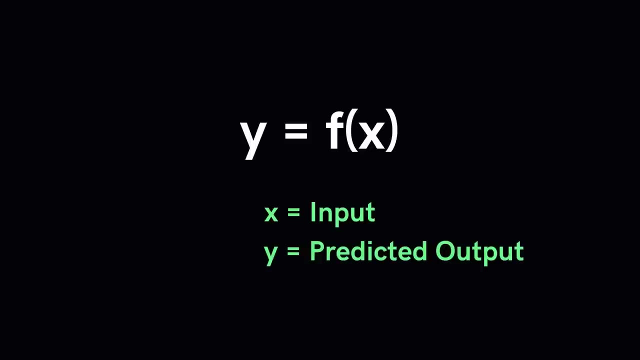 The objective of a supervised learning model is to predict the correct label for newly presented input data. At its most basic form, a supervised learning algorithm can simply be written: as: y is equal to fx, Where y is the predicted output That is determined by a mapping function that assigns a class to an input value, x. 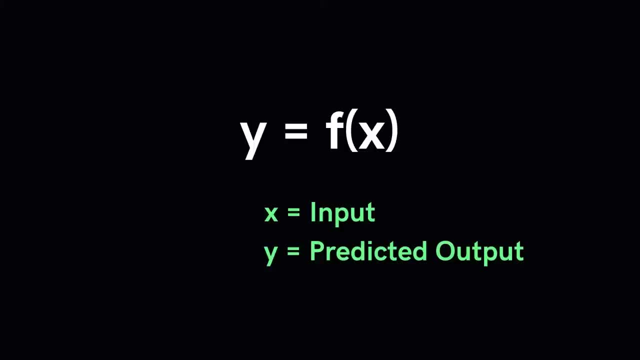 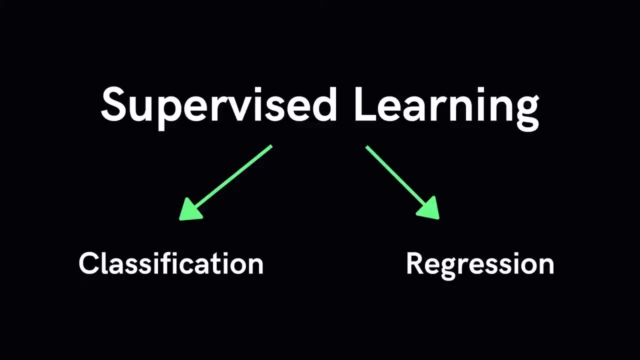 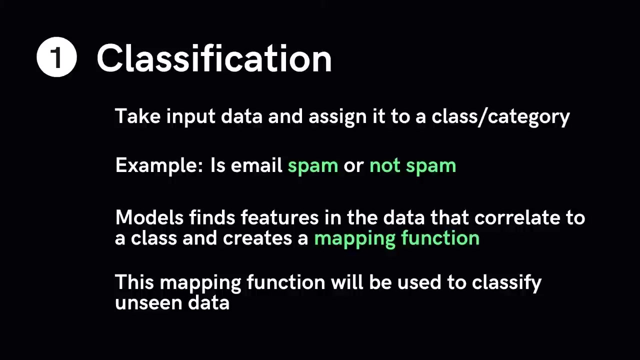 The function used to connect input features to a predicted output is created by the machine learning model during training. Supervised learning can be split into two subcategories: classification and regression. During training, a classification algorithm will be given data points with an assigned category. 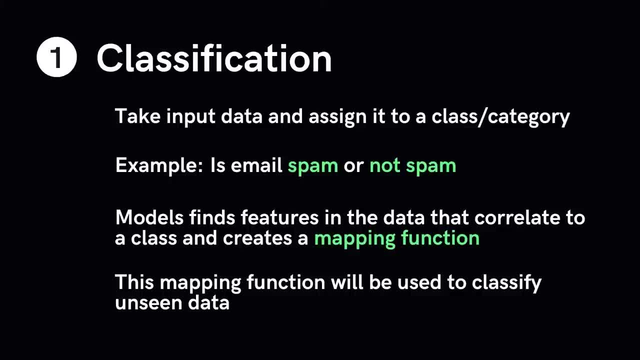 The job of a classification algorithm is then to take this input value and assign it to a class of category that it fits into, Based on the training data provided. The most common example of classification is determining if an email is spam or not With two classes. you choose from spam or not spam. this problem is called a binary. 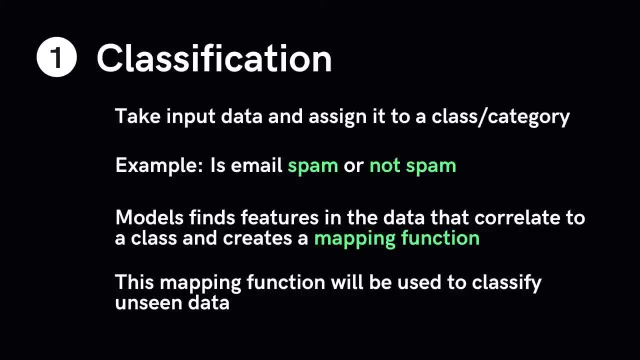 classification problem. The algorithm will be given training data with emails that are both spam and not spam and the model will find the features within the data that correlate to either class and create a mapping function. Then, when provided with an unseen email, The model will use this function to determine whether or not the email is spam. 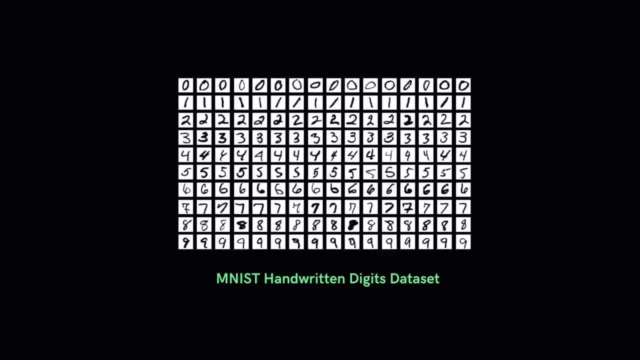 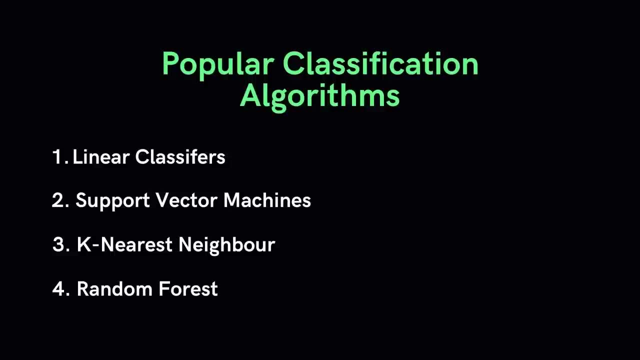 An example of a classification problem would be the MNIST handwritten digits dataset, where the inputs are images of handwritten digits or pixel data and the output is a class label for what digit the image represents, that is, numbers 0 to 9.. There are numerous algorithms to solve classification problems, each which depends on the data and 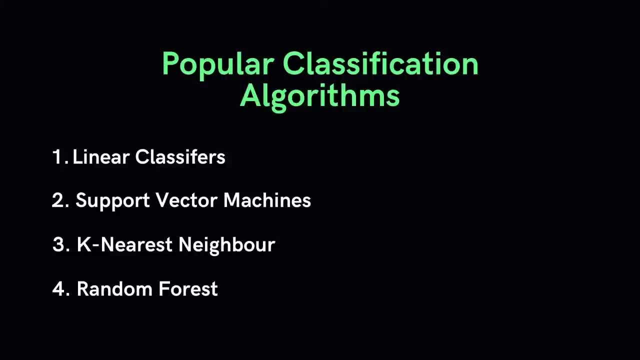 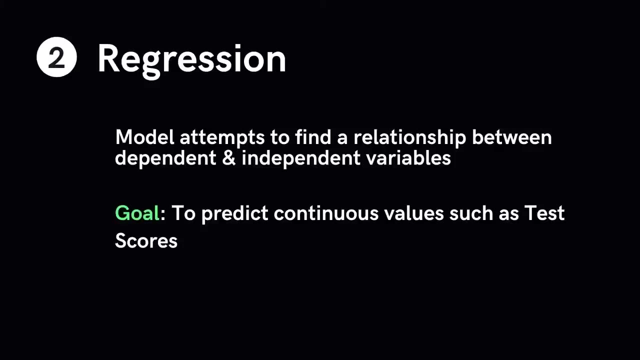 the situation. Here are a few popular classification algorithms: Linear classifiers, Support vector machines, decision trees, k-nearest neighbors and random forest. Regression is a predictive statistical process where the model attempts to find the important relationship between dependent and independent variables. 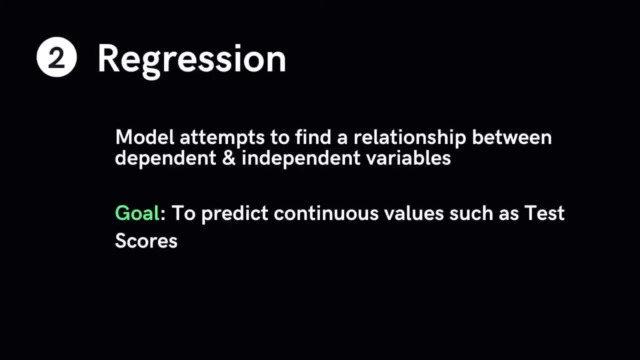 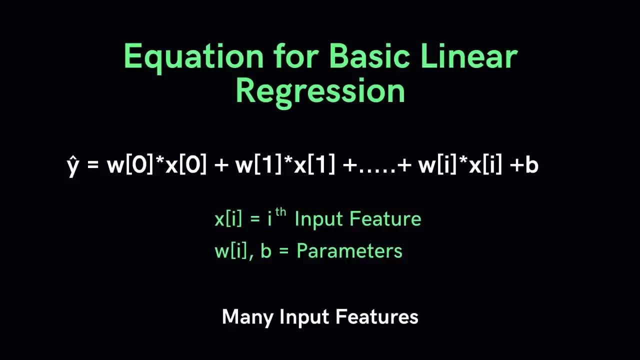 The goal of a regression algorithm is to predict a continuous number, such as sales income and tax cost. The equation for a basic linear regression can be written as follows: where x represents the features of the data. For simple linear regression models with only one feature in the data, the formula: 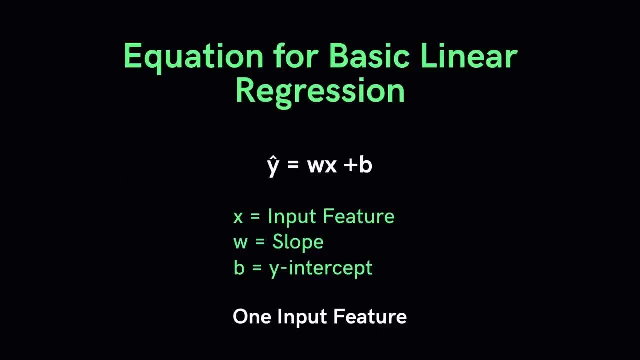 looks like this: where w is the slope, x is the single feature and b is the y-intercept. Familiar For simple regression problems such as this, the model's predictions are represented by the line of best fit. For models using two features, a plane is used. 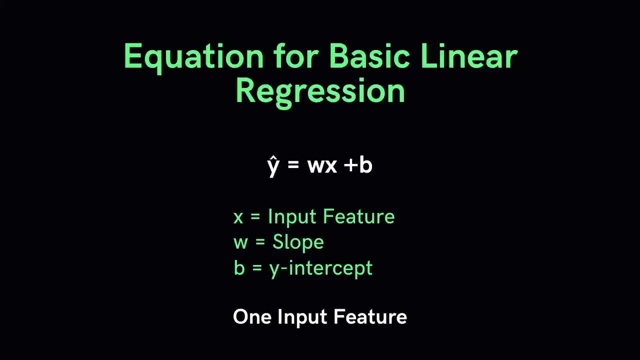 And for models with more than two features, a hyperplane is used. Imagine we want to determine a student's test grade, For example. we want to determine a student's test grade. For example: we want to determine a student's test grade. 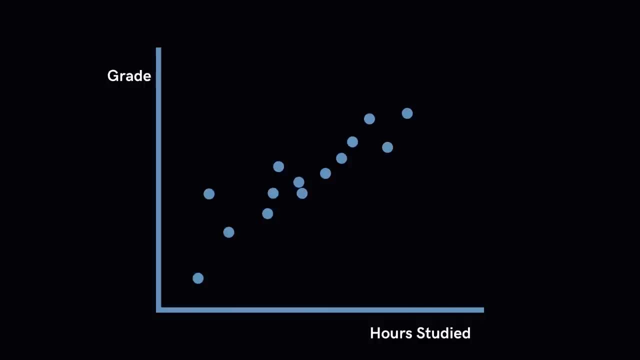 We can use the line of best fit to predict the test score based on how many hours they study the week of the test. Let's say, the plot data with the line of best fit looks like this: There is a clear positive correlation between r studied, the independent variable and the. 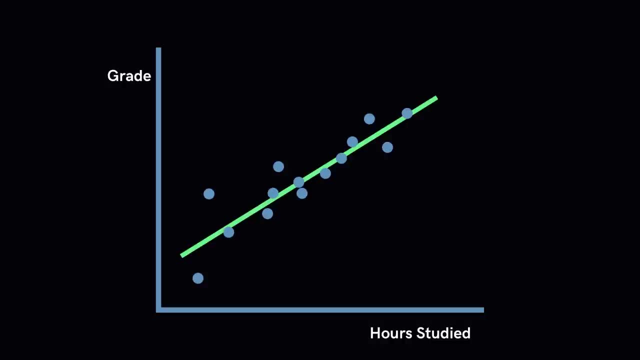 student's final test score. the dependent variable, A line of best fit, can be drawn through the data points to show the model's predictions when given a new input. Say, we wanted to know how well a student would do with five hours of studying. 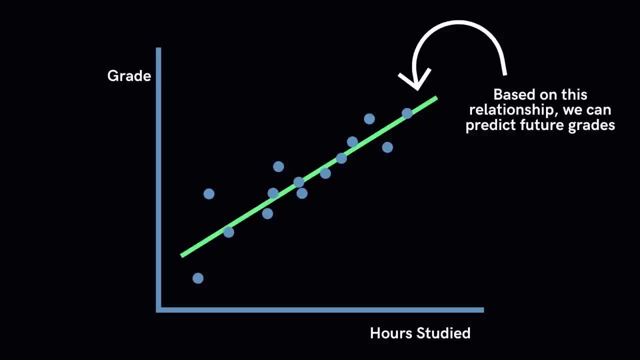 We can use the line of best fit to predict the test score based on the number of hours they study. We can use the line of best fit to predict the test score based on the number of hours they study. We can use the line of best fit to predict the test score based on the number of hours. 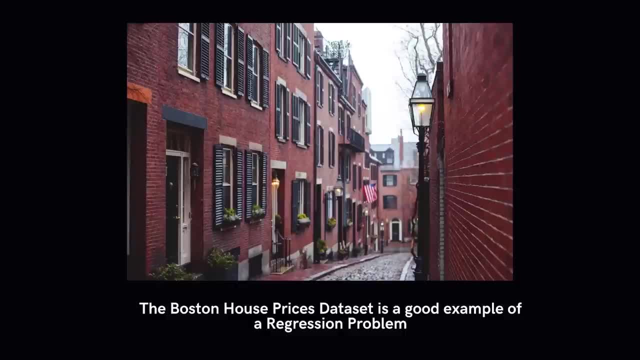 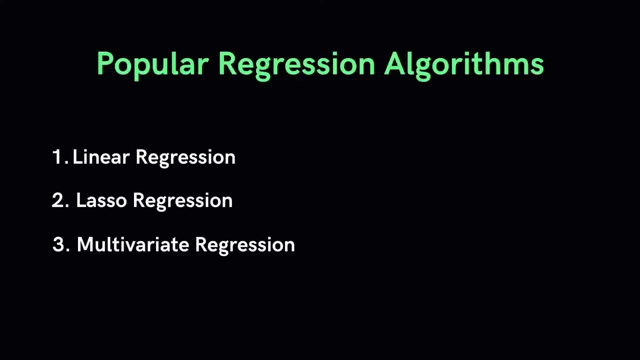 they study. Another example of regression problem would be the Boston House prices data set, where the input of variables that describe a neighborhood and the output is a house price in dollars. There are many different types of regression algorithms. Three most common are linear regression, Lasser regression and multivariate regression. 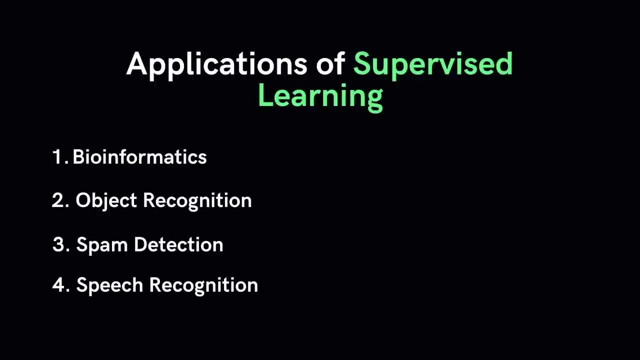 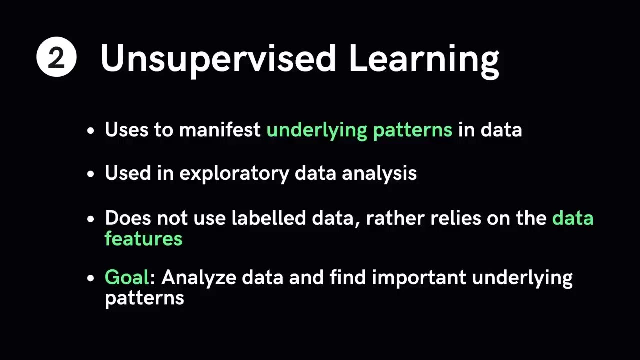 Supervised learning finds applications in classification and regression problems like bioinformatics, Such as fingerprints, Fingerprint iris and face recognition in smartphones, Object recognition, spam detection and speech recognition. Unsupervised learning is a branch of machine learning that is used to manifest underlying 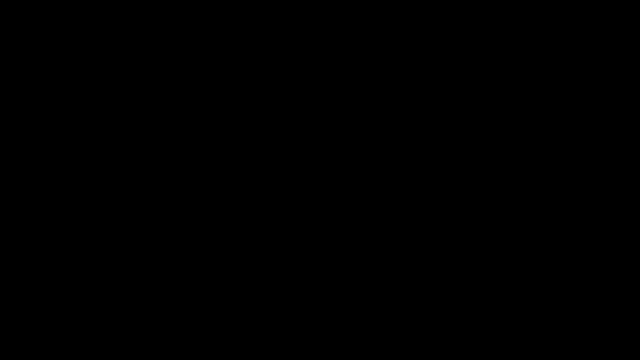 patterns in data and is often used in exploratory data analysis. Unlike supervised learning, unsupervised learning does not use label data, but instead focuses on the data's features. Digital training data has a corresponding output for each input. The goal of an unsupervised learning algorithm is to analyze data and find important features. 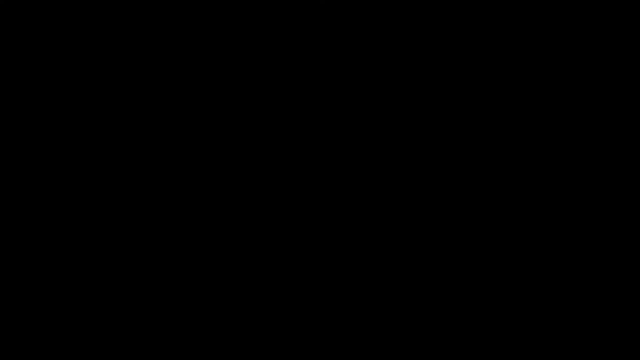 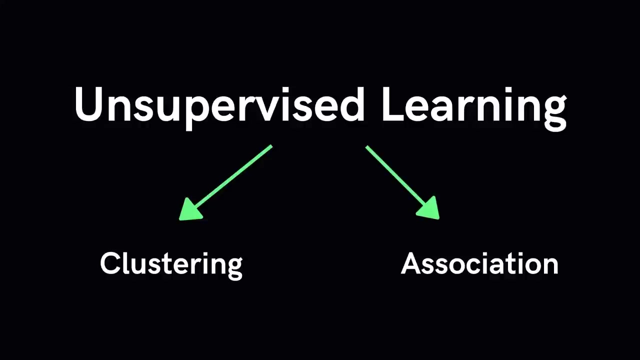 in that data. Unsupervised learning will often find subgroups or hidden patterns within the dataset that a human observer might not pick up on, And this is extremely useful. as we'll soon find out, Unsupervised learning can be of two types: clustering and association. 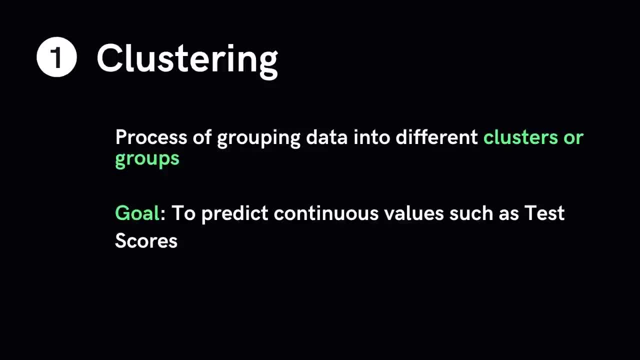 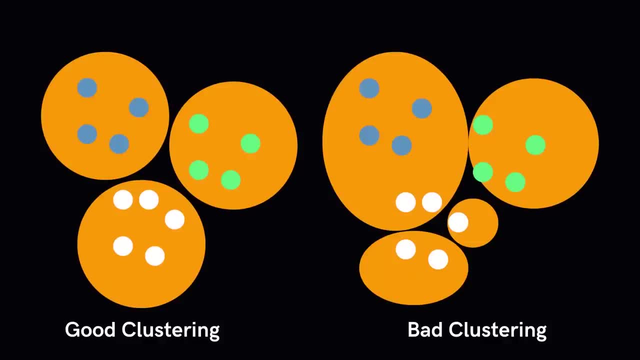 Clustering is the simplest And among the most common Applications of unsupervised learning. It is the process of grouping the given data into different clusters or groups. Clusters will contain data points that are as similar as possible to each other and as 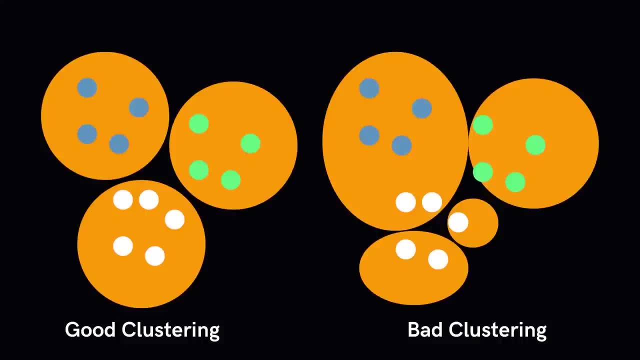 dissimilar as possible to data points in other clusters. Clustering helps find underlying patterns within the data that may not be noticeable to a human observer. It can be broken down into Partitional clustering and Hierarchical clustering. Partitional clustering refers to a set of clustering applications. 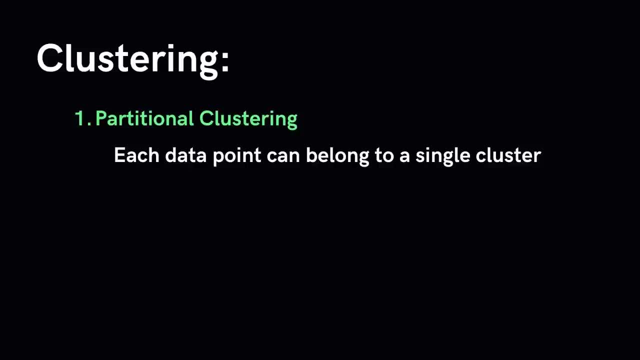 Partitional clustering refers to a set of clustering applications that can be used to classify data points. Hierarchical clustering is a set of clustering algorithms where each data point in a dataset can belong to only one cluster. Hierarchical clustering finds clusters by a system of hierarchies. 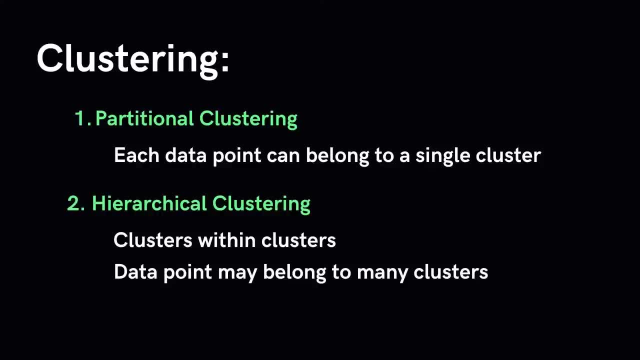 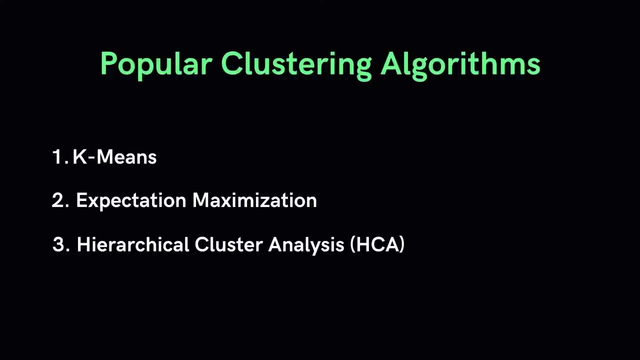 Every data point can belong to multiple clusters. Some clusters will contain smaller clusters within it. This hierarchy system can be organized as a tree diagram. Some of the more commonly used clustering algorithms are the k-means, expectation maximization, the hierarchical cluster analysis or the ECA. 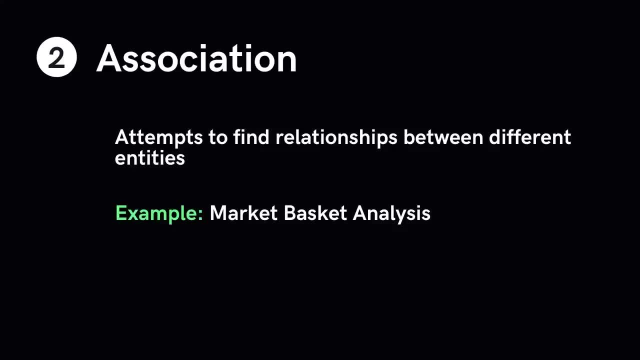 Here are some of the most commonly used clustering algorithms. Association, on the other hand, attempts to find relationships between different entities. The classic example of association rules is market basket analysis. This means using a database of transactions in a supermarket to find items that are frequently. 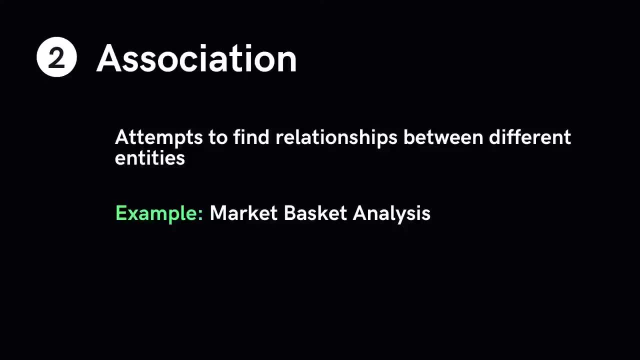 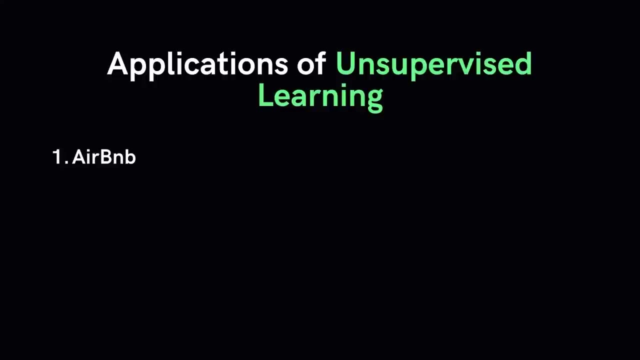 bought together. For example, a person who buys potatoes and burgers usually buys beer. For example, a person who buys tomatoes and pizza cheese might want to bring pizza bread, and so on. Unsupervised learning finds applications almost everywhere, For example, Airbnb, which helps host stays and experiences and connect people all over. 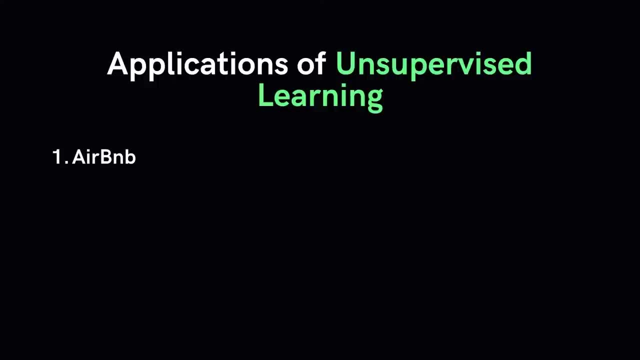 the world. This application uses unsupervised learning algorithms where a potential client queries their requirements, and Airbnb learns these patterns and recommends stays and experiences which fall under the same group or cluster. For example, a person looking for houses in San Francisco might not be interested in finding. 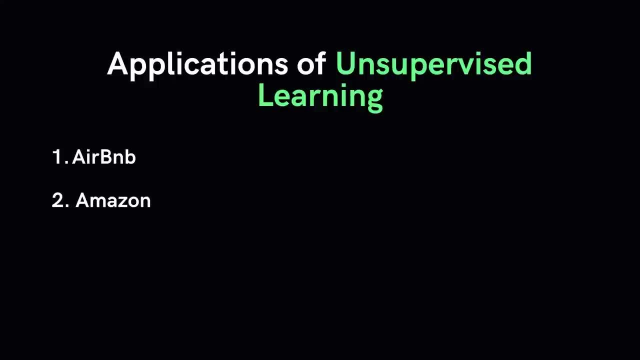 houses in Boston. Amazon also uses unsupervised learning. It's a great way to build relationships. It's a great way to learn the customers' purchases and recommend products which are frequently bought together, which is an example of association rule mining. Credit card fraud detection is another unsupervised learning algorithm that learns the various 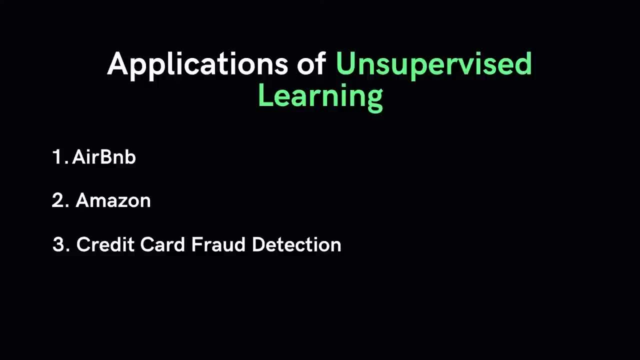 patterns of a user and their usage of a credit card. If the card is used in parts that do not match the behavior, an alarm is generated which could possibly be marked as fraud And in some cases, your bank might call you to confirm whether it was you using the card. 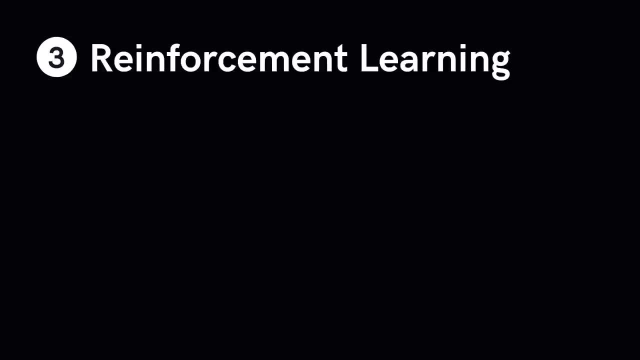 or not. Reinforcement learning is a type of machine learning technique that enables an agent to learn in an interactive environment by trial and error, using feedback from its own actions and experiences. Like supervised learning, it uses mapping between the input and the output. 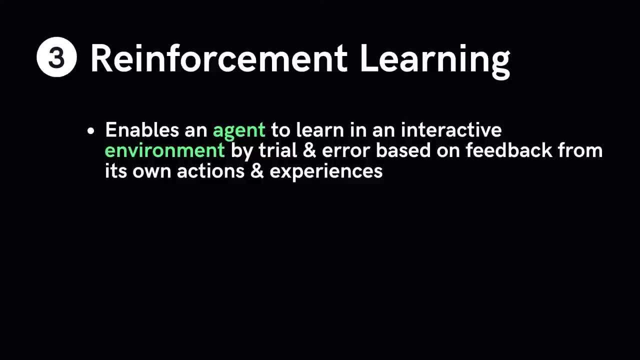 But unlike supervised learning, where feedback provided to the agent is a correct set of actions for performing a task, reinforcement learning uses rewards and punishments as signals for positive and negative behavior. So what is reinforcement learning? When you compare it with unsupervised learning, reinforcement learning is different in terms. 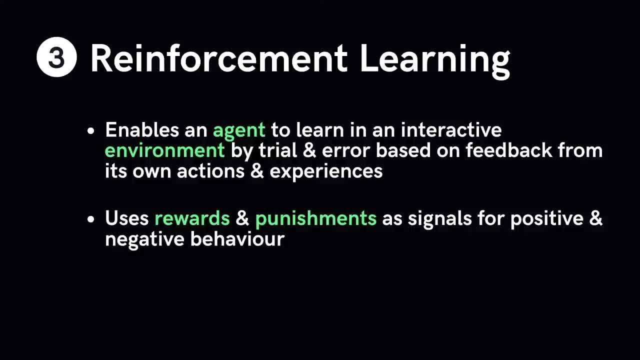 of its goals. While the goal in unsupervised learning is to find similarities and differences between data points, in reinforcement learning, the goal is to find a suitable action model that would maximize the total cumulative reward of the agent. Reinforcement learning refers to goal-oriented algorithms which learn how to attain a complex 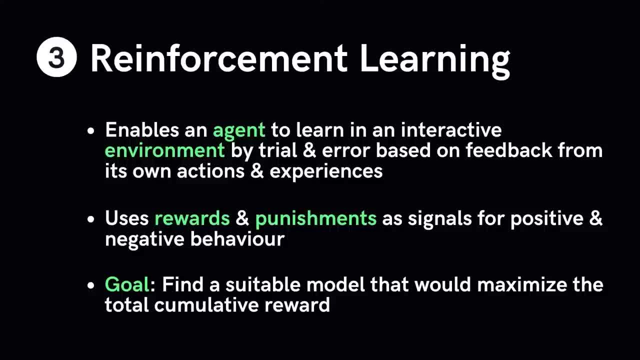 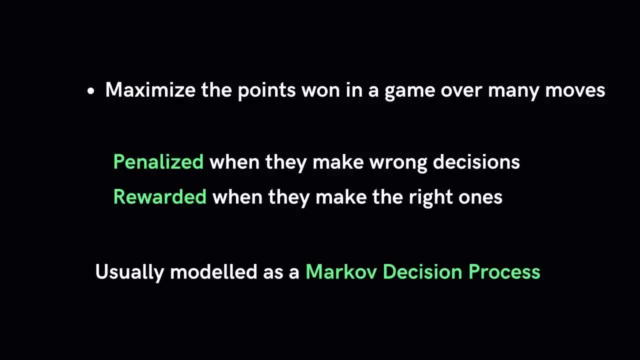 objective or goal or how to maximize along a particular dimension or goal. For example, they can maximize the points won in a game over many moves. Reinforcement learning algorithms can start from a blank slate and, under the right conditions, achieve superhuman performance. 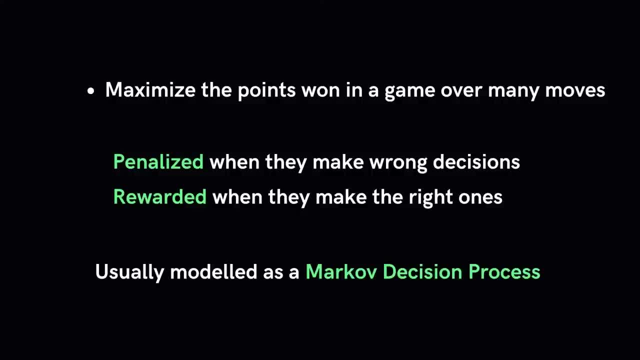 Like a pet, incentivized by scolding and treats. these algorithms are penalized when they make the wrong decisions and rewarded when they make the right ones. This is reinforcement. Reinforcement learning is usually model, as a Markov decision. In the past, reinforcement learning has been a model for countermeasures. 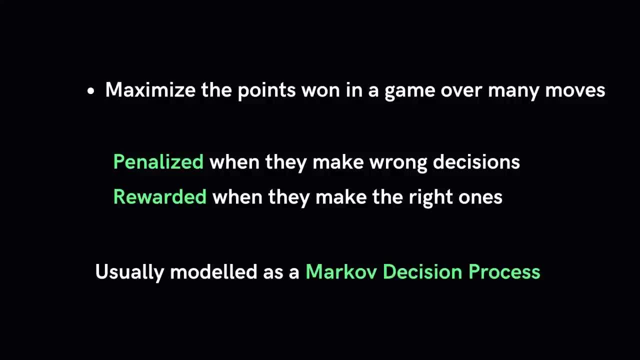 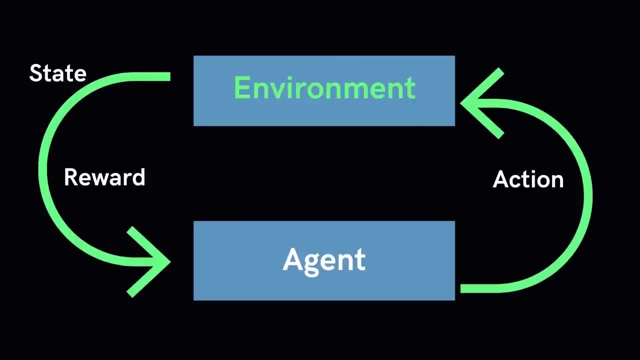 decision process, although other frameworks, like Q-learning, are used. Some key terms that describe the elements of a reinforcement learning problem are: the environment, which is the physical world in which the agent operates. The state represents the current situation of the agent. Reward is the feedback received from the environment. 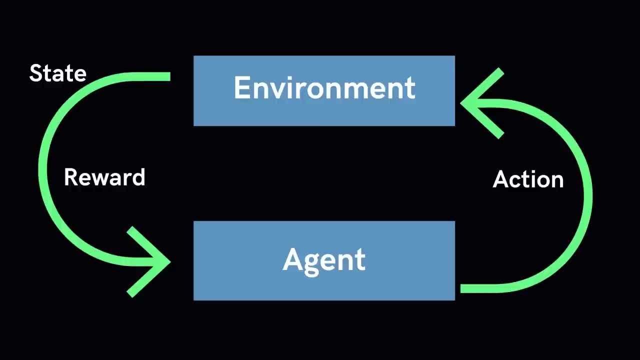 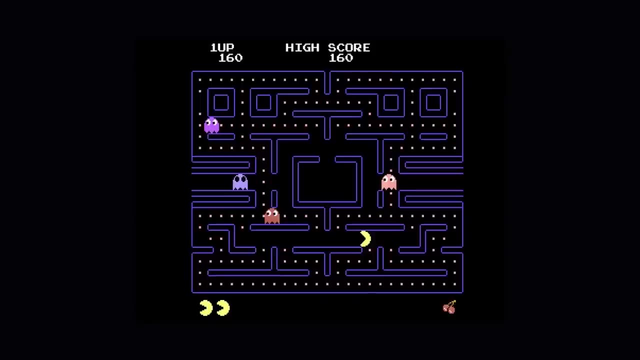 Policy sometimes is the method to map the agent's state to the agent's actions. And finally, value is the future reward that an agent will receive by taking an action in a particular state. A reinforcement learning problem can be best explained through games. Let's take the game of Pac-Man, where the goal of the agent or Pac-Man is to eat the. 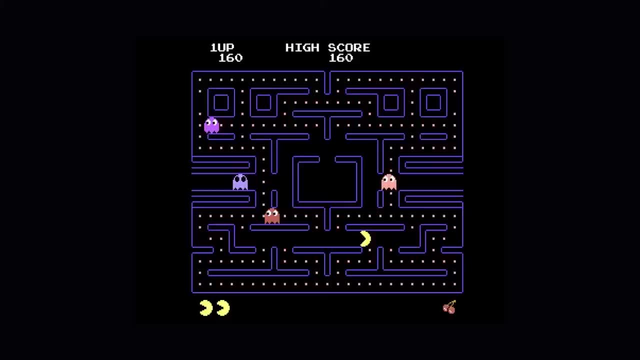 food in the grid while avoiding the ghost on its way. The grid world is the interactive environment for the agent. Pac-Man receives a reward for eating food and punishment if it gets killed by the ghost, That is, it loses the game. 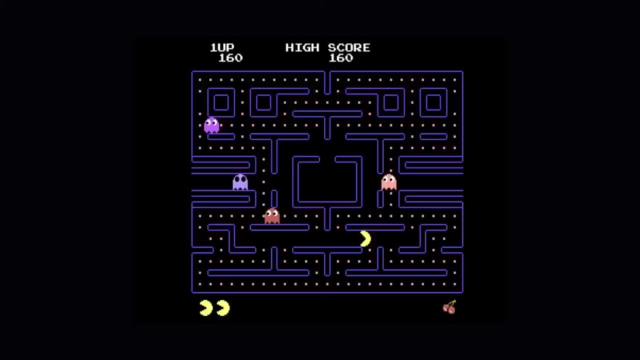 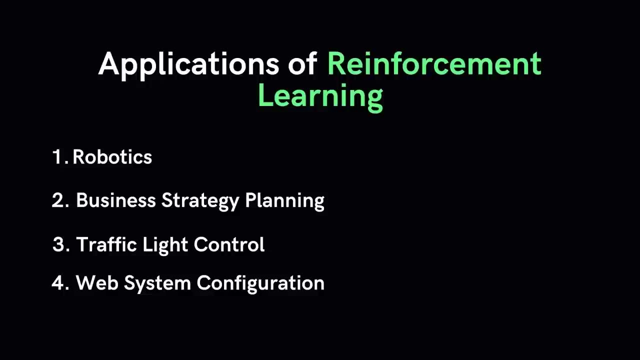 The states are the location of Pac-Man in the grid world, and the total cumulative reward is Pac-Man winning the game. Reinforcement learning finds applications in robotics, business strategy planning, traffic light control, web system configuration and aircraft and robot motion control. 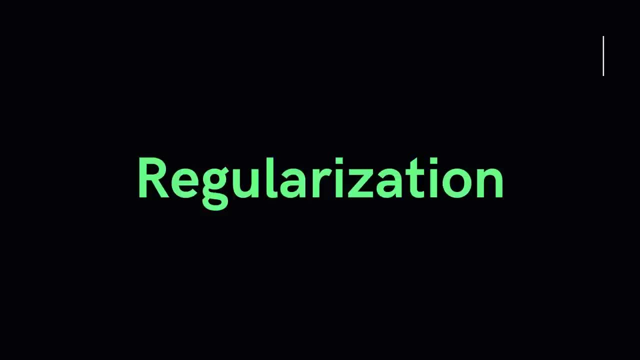 A central problem in deep learning is how to make an algorithm that will perform well not just in training data, but also in learning. A central problem in deep learning is how to make an algorithm that will perform well not just in training data, but also in learning. 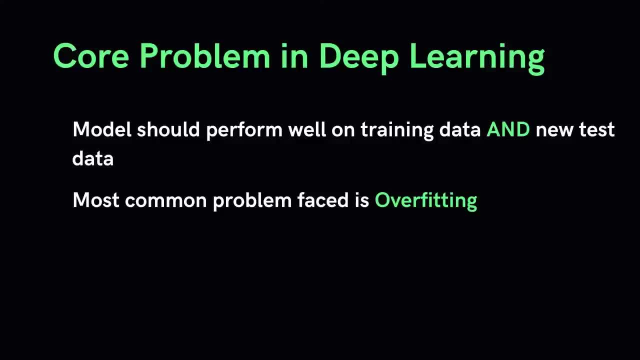 A central problem in deep learning is how to make an algorithm that will perform well, not just in learning. One of the most common challenges you will face when training models is the problem of overfitting a situation where your model performs exceptionally well on training data. 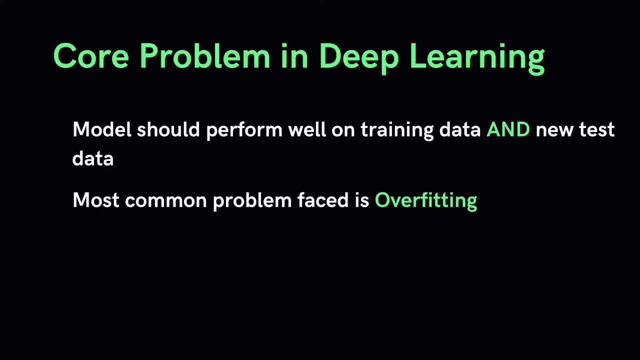 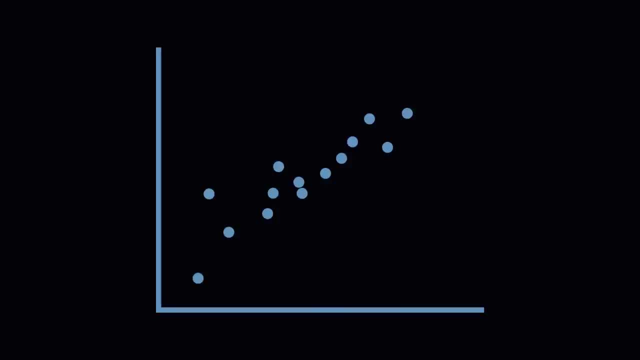 but not on testing data. Say, I have a data set graphed on the xy plane like: so now I want to construct a model that would best fit the data set. What I can do is draw a line of some random slope and intercept. 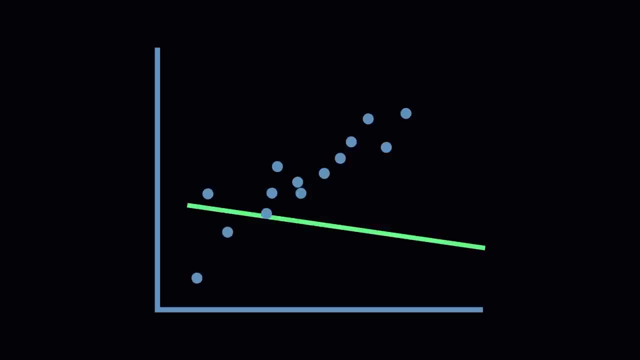 Now, evidently this isn't the best model, And in fact, this is called underfitting, because it doesn't fit the model well. In fact, it underestimates the dataset. Instead, what we could do is draw a line that looks something like this: 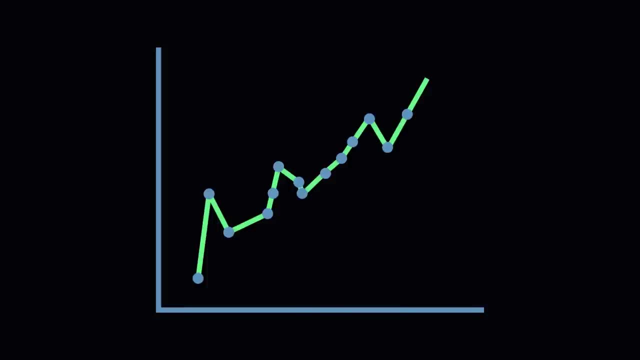 Now this really fits our model the best, but this is overfitting. Remember that while training, we show our network some training data, and once that's done, we'd expect it to be almost close to perfect. The problem with this graph is that, although it is probably the best line of fit for this graph, 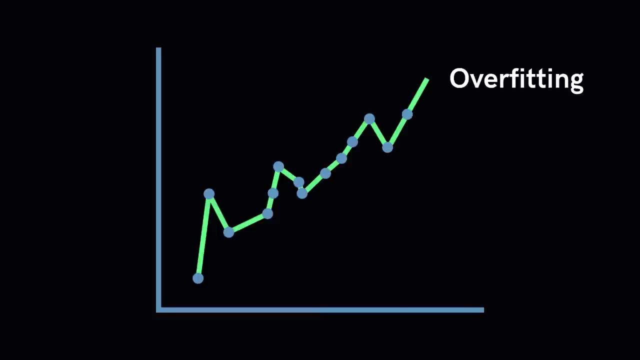 it is the best line of fit only if you're considering your training data. What your network has done in this graph is memorize the patterns between the training data and won't give accurate predictions at all on data it's never seen before. And this makes sense because, instead of memorizing patterns generally, 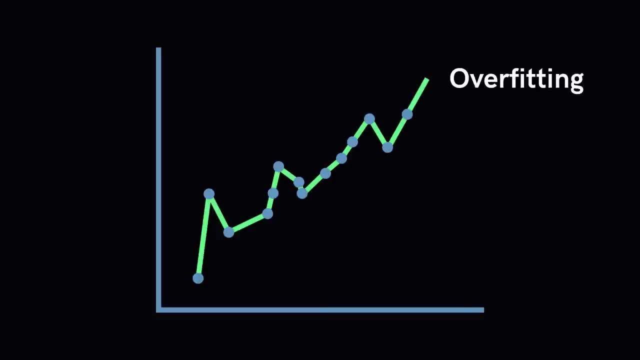 to perform well on both training as well as new testing data. our network, in fact, has memorized the patterns only on the training data, so it obviously won't perform well on new data. This is the problem of overfitting: It fitted too much. 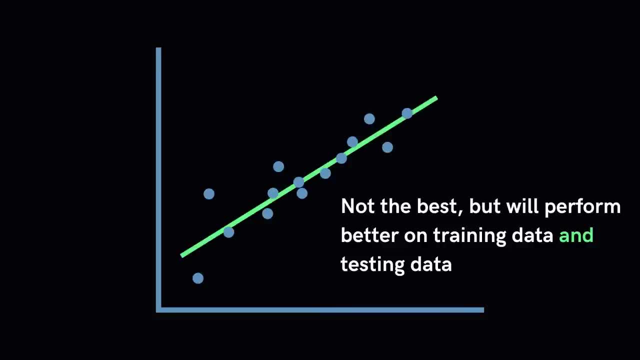 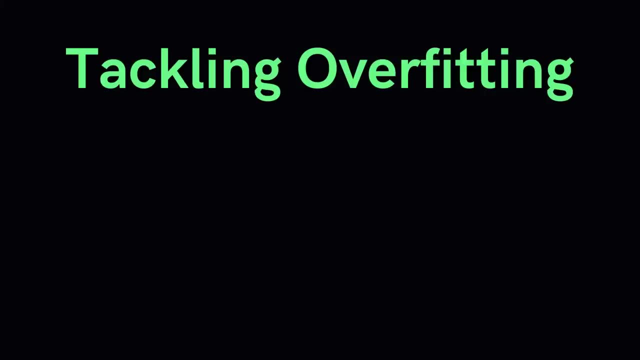 And, by the way, this would be the more accurate kind of fitting. It's not perfect, but it'll do well on both training as well as new testing data with sizeable accuracy. There are a couple of ways to tackle overfitting. 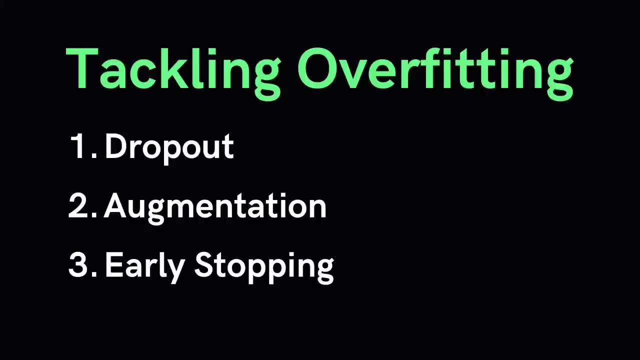 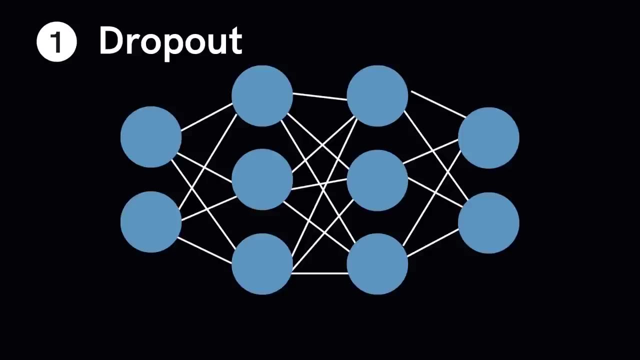 The most interesting type of regularization is dropout. It produces very good results and is consequently the most frequently used regularization technique in the field of deep learning. To understand dropout, let's say that we have a neural network with two hidden layers. What dropout does is that at every iteration it randomly selects some nodes. 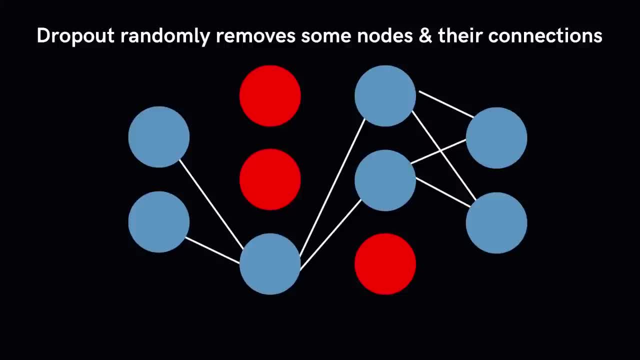 and removes them, along with their incoming and outgoing connections, as shown. So each iteration has a different set of nodes, and this results in a different set of outputs. So why do these models perform better? These models usually perform better than a single model, as they capture more randomness. 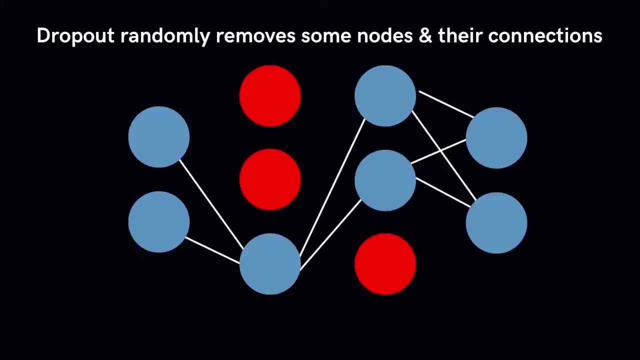 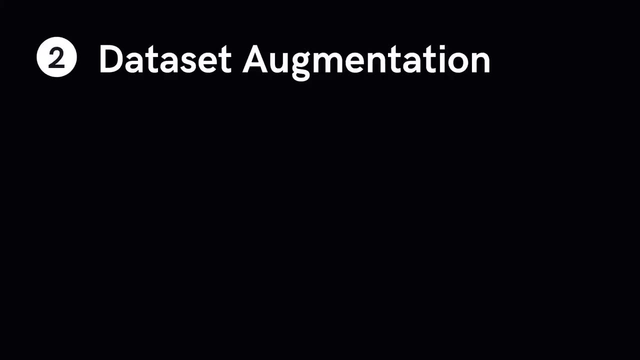 and it memorizes less of the training data and hence will be forced to generalize better and build a more robust predictive model. Sometimes the best way to make a deep learning model generalize better is to train it on more data. In practice, the amount of data we have is limited. 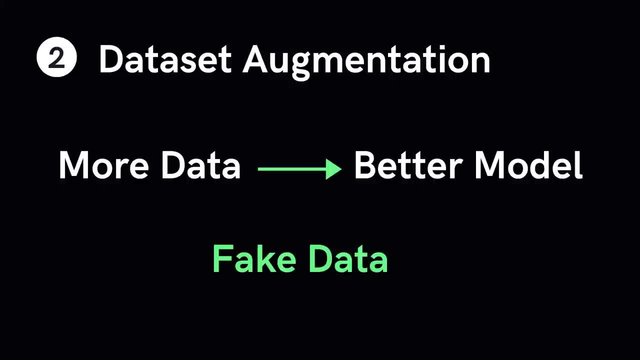 and one way to get around this problem is to create fake data and add it to the training set. For some deep learning tasks it is reasonably straightforward to create new fake data. This approach is easiest for classification. A classifier needs to take a complicated high. 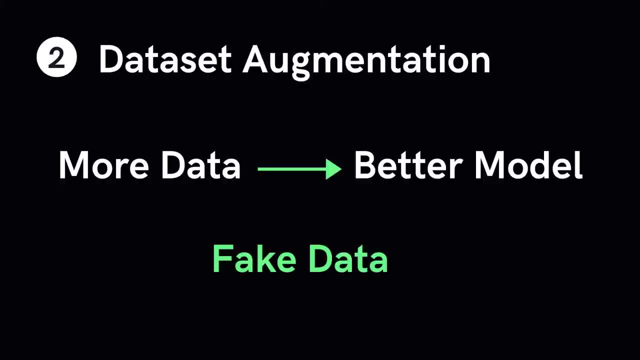 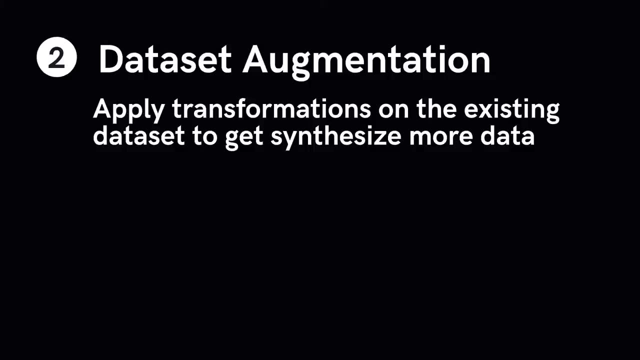 dimensional input x and summarize it with the category identity y. This means that the main task facing our classifier is to be invariant to a wide variety of transformations. We can generate new xy pairs easily just by applying transformations on the xy inputs in our training set. 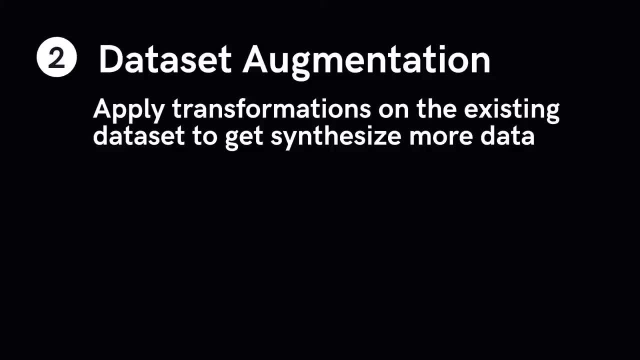 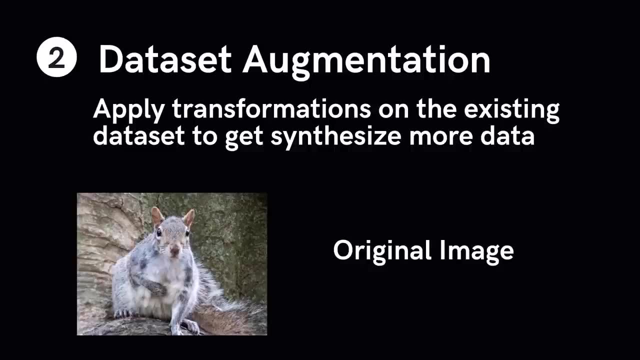 Dataset augmentation has been a particularly effective technique for a specific classification problem. Object recognition Images are high dimensional and include an enormous range of factors of variation, many of which can easily be simulated. Operations like translating the training images- a few pixels in each direction- can often greatly improve generalization. Many other operations- 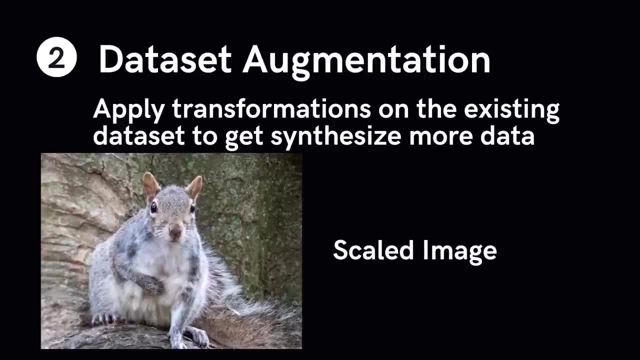 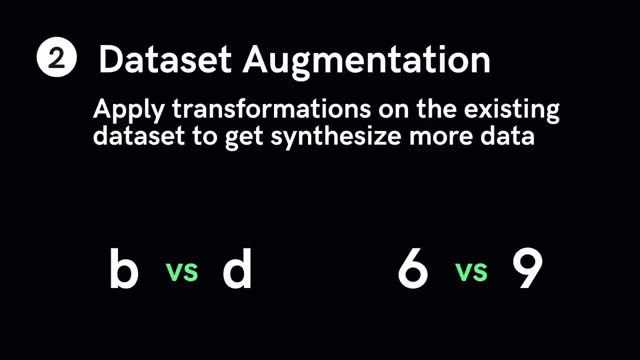 such as rotating the image or scaling the image have also proved quite effective. You must be careful not to apply transformations that would change the correct class, For example, an optical character recognition task that required recognizing the difference between a, b and a, d and the. 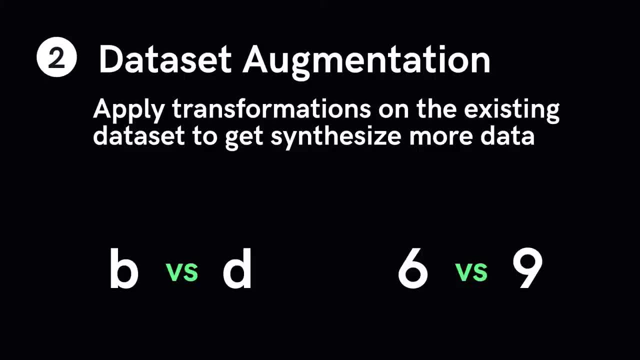 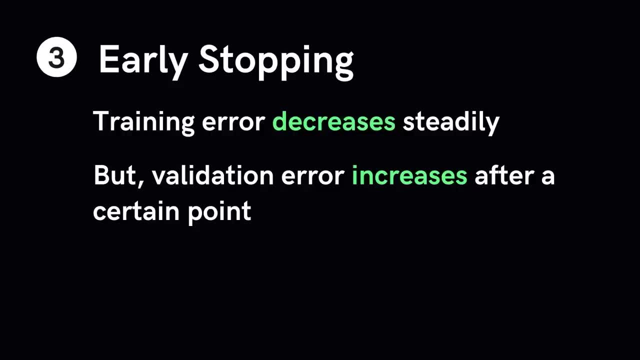 difference between a 6 and a 9.. Horizontal flips and 180 degree rotations are not appropriate ways of augmenting datasets for these tasks. When training large models with sufficient representational capacity to overfit the task, we often observe that the training error decreases steadily over time. 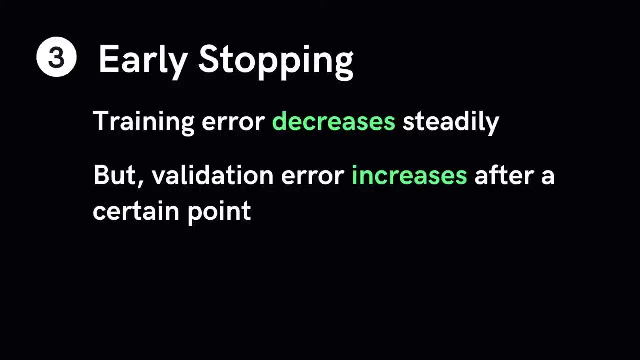 but the error validation set begins to rise again. This means we can obtain a model with the better validation set error, and thus hopefully better test set error, by stopping training at the point where the error in the validation set starts to increase. This strategy is known as. 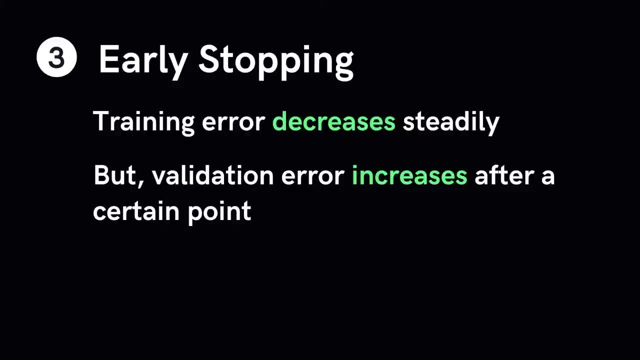 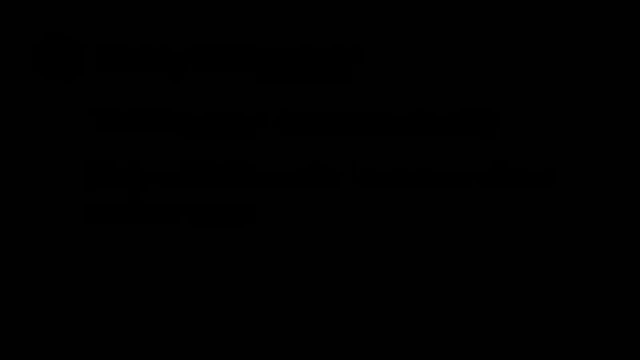 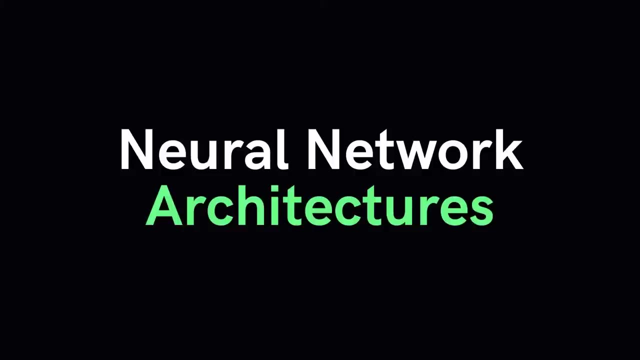 early stopping. It is probably the most commonly used form of regularization in deep learning today. Its popularity is due to both its effectiveness and its simplicity. In this section, I am going to introduce the three most common types of neural network architectures today: Fully connected- v4- renewal network. 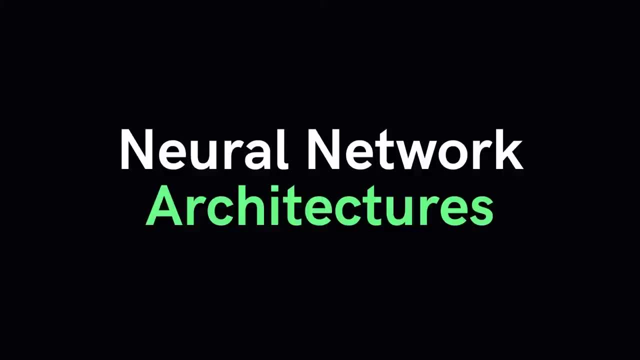 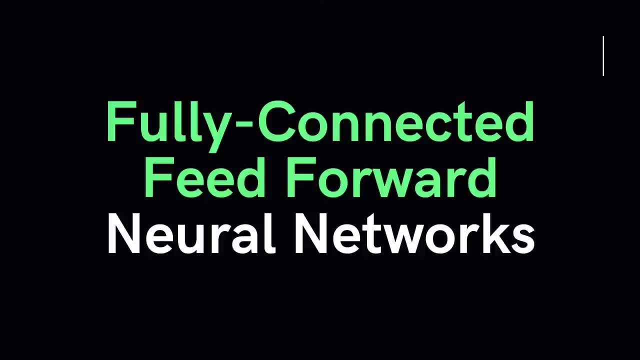 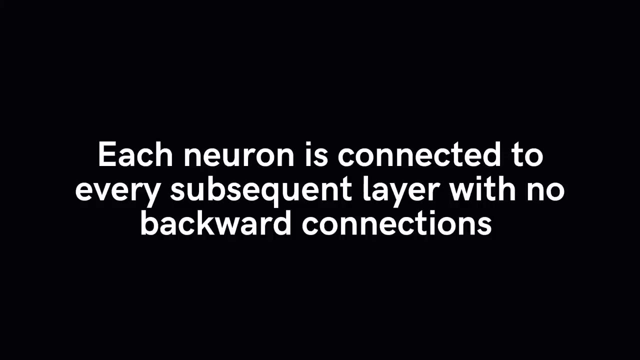 recurrent neural networks and convolutional neural networks. The first type of neural network architecture we are going to discuss is a fully connected v4 neural network. By fully connected I mean that each neuron in the preceding layer is connected to every neuron in the subsequent layer without any connection. 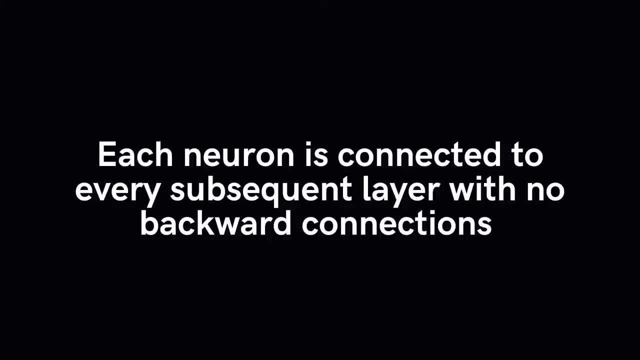 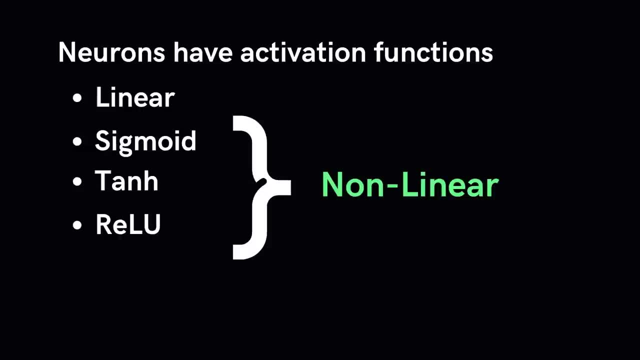 backwards. There are no cycles or loops in the connections in the network. As I mentioned previously, each neuron in a neural network can have its own function called activation function, which is the activation function of a neuron when given its input. There are several types of activation functions that can change. 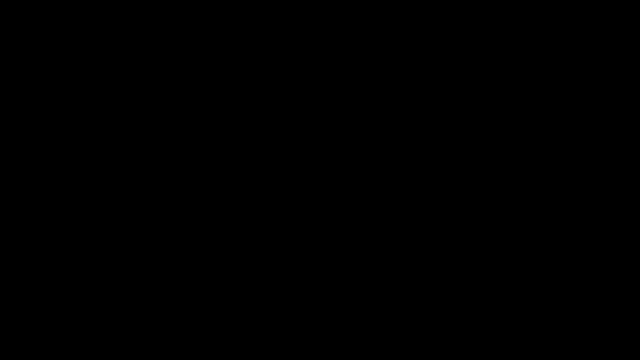 this input-to-output relationship to make a neuron behave in a variety of ways. Some of the most well-known activation functions are the linear function, which is a straight line that essentially multiplies the input by a constant value. the sigmoid function that ranges from 0 to 1, the hyperbolic tangent or the tanh function, ranging. 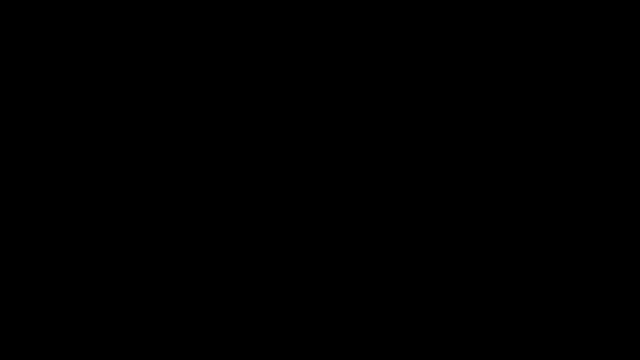 from negative 1 to positive 1, and the linear function that essentially multiplies the input to a constant value. The hyperbolic tangent, or the tangent function, ranges from negative 1 to positive one, and the rectified linear unit, or the ReLU function, which is a piecewise function that 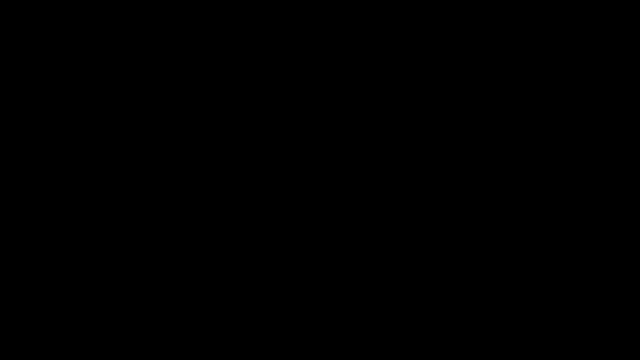 outputs: a zero if the input is less than a certain value, or a linear multiple if the input is greater than a certain value. Each type of activation function has its pros and cons, so we use them in various layers in the Deep Neural Network, based on the problem each is designed to. 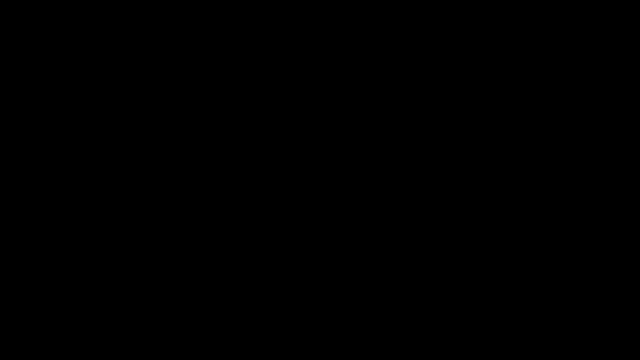 solve, In addition, the last three activation functions we refer to as non-linear functions because the output is not a linear multiple of the input. Non-linearity is what allows Deep Neural Networks to model complex functions. Using everything we've learned so far, we can create. 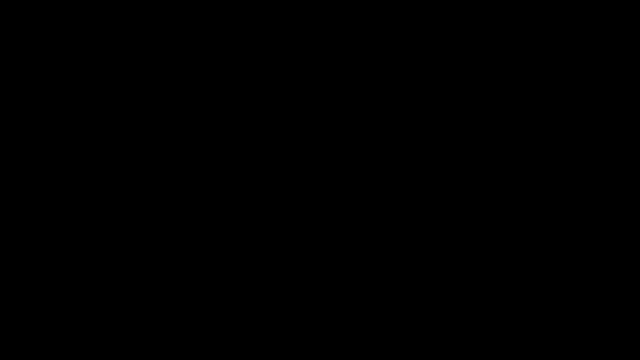 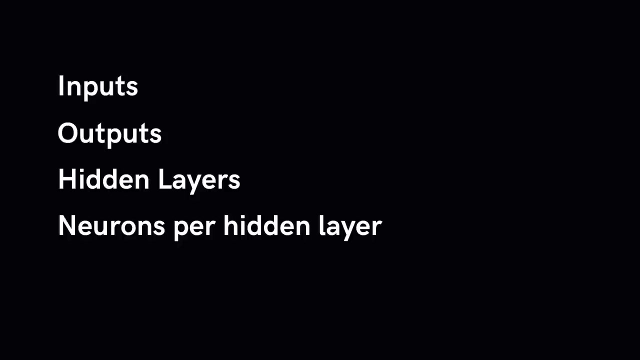 a wide variety of fully connected feedforward neural networks. We can create networks with various inputs, various outputs, various hidden layers, neurons per hidden layer and a variety of activation functions. These numerous combinations allow us to create a variety of powerful Deep Neural Networks. 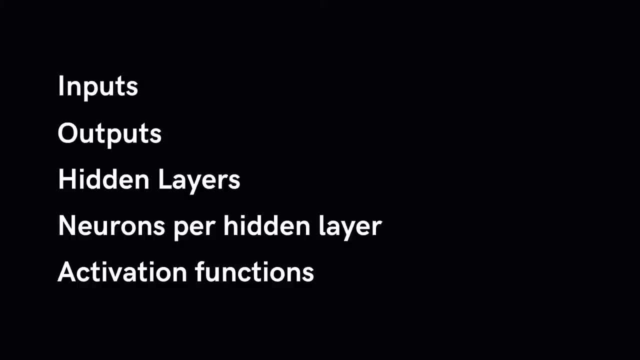 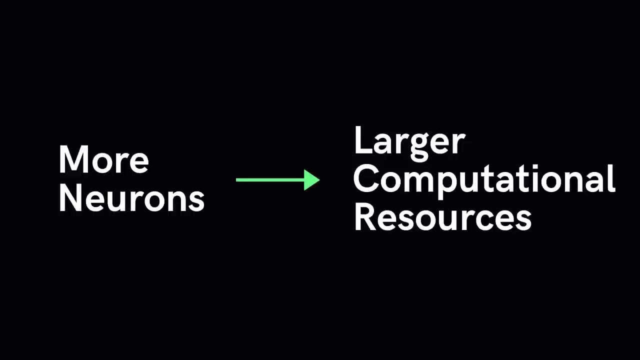 That can solve the wide array of problems. The more neurons we add to each hidden layer, the wider the network becomes. In addition, the more hidden layers we add, the deeper the network becomes. However, each neuron we add increases the complexity and thus the computational resource. 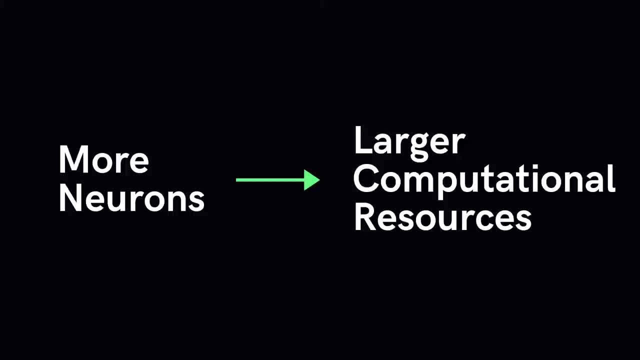 necessary to train the neural network increases. This increase in complexity isn't linear in the number of neurons we add, so it leads to an explosion in complexity and training time for large neural networks. That's a trade-off you need to consider when you are building Deep Neural. 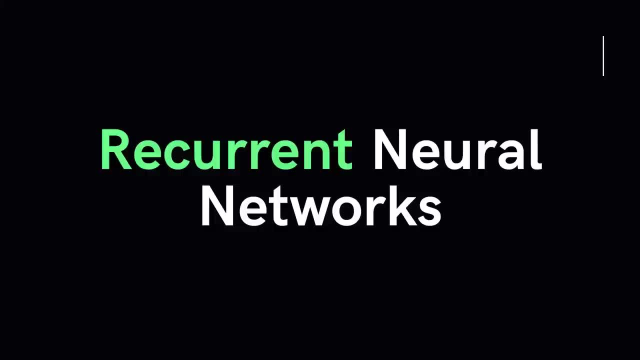 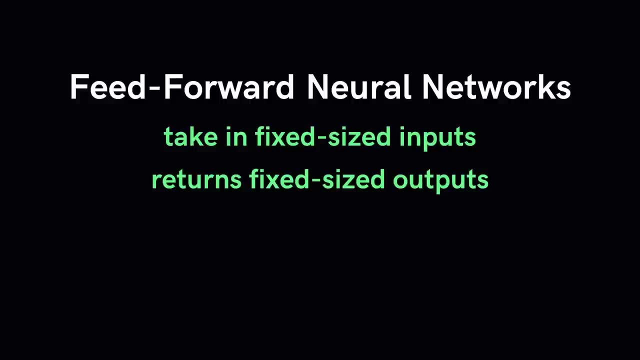 Networks. All the neural networks we've discussed so far are known as feedforward neural networks. They take in a fixed sized input and give you a fixed size output. That's all it does And that's what we expect neural networks to do: Take in an input and give a sizable output. 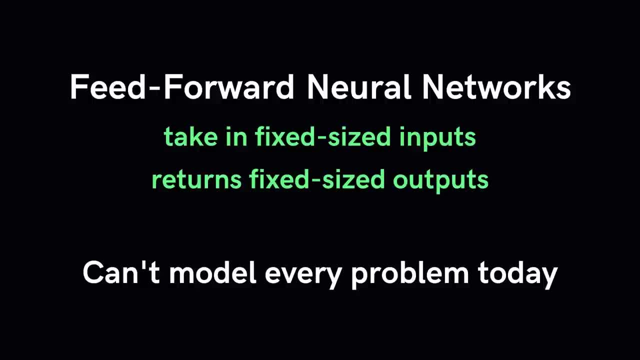 But, as it turns out, these plain or vanilla neural networks aren't able to model every single problem that we have today. This is because they don't have a fixed size input. They don't have a fixed size output. To better understand this, use this analogy. Suppose I show you the picture of a ball. 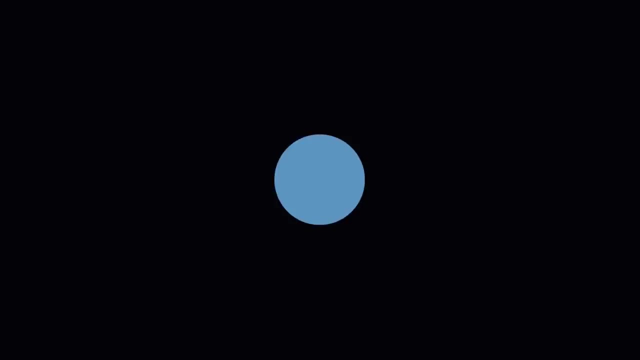 a round spherical ball that was moving in space in some direction. I've just taken a photo of the ball, or a snapshot of the ball at some time t Now I want you to predict the next position of the ball in, say, two or three seconds. You're probably not going to give me an accurate answer. 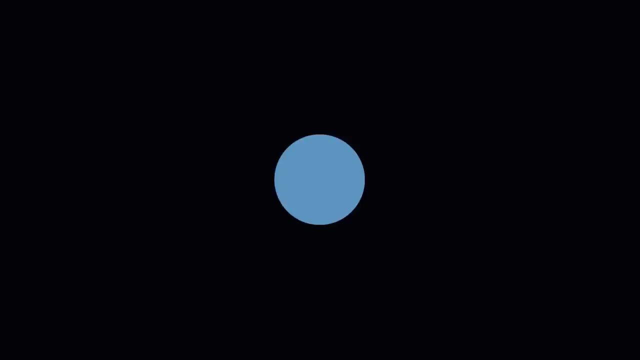 Now let's look at another example. Suppose I walk up to you and say the word dog, You will never understand my statement because, well, it doesn't make sense. There are trilling combinations solely using the word dog, and among these trilling combinations, I'm expecting you to now guess what I'm trying to tell you. 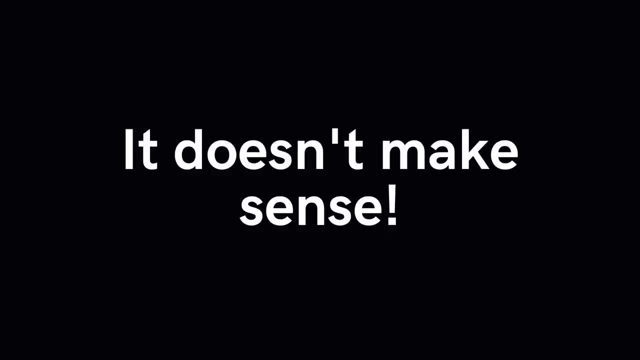 What these two examples have in common is that it doesn't make sense. It doesn't In the first case. I'm expecting you to predict the next position in time, and in the second, I'm expecting you to understand what I mean by dog. These two examples cannot be understood and interpreted unless some 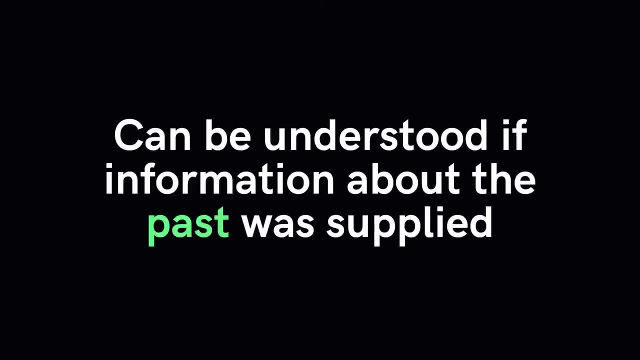 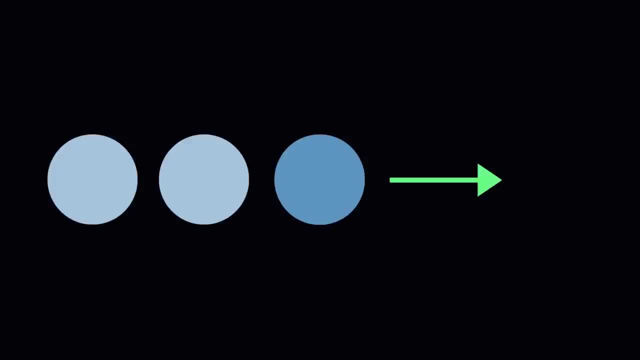 information about the past was supplied. I'm expecting you to understand what I mean by dog Now in the first example. if I give you the previous position states of the ball and now ask you to predict the future trajectory of the ball, you're going to be able to do this. 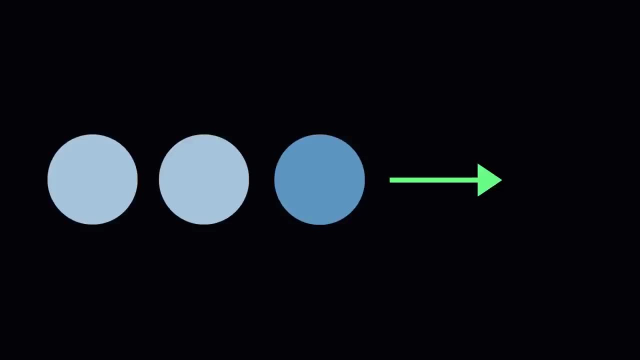 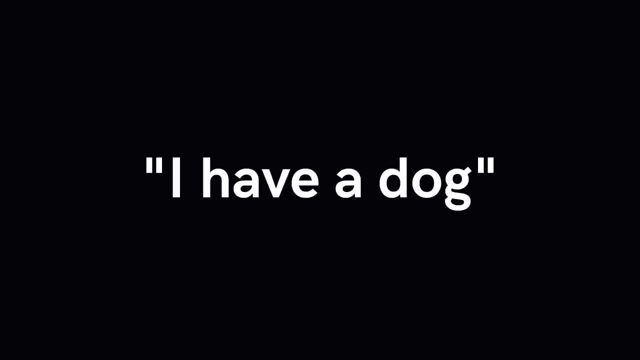 accurately. and, in the second case, if I give you a full sentence saying I have a dog, This makes sense, because now you understand that, out of the trillion possible combinations involving a dog, my original intent was for you to understand that I have a dog. Why did I give you this example? How? 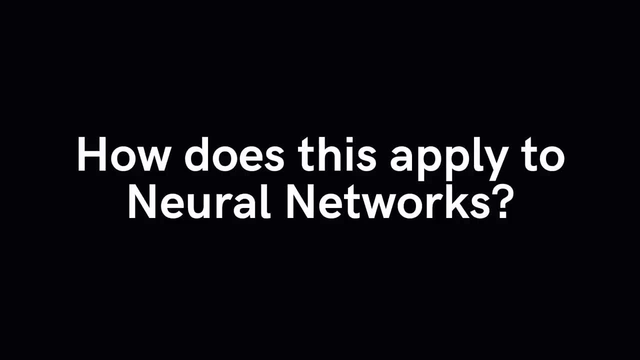 does this apply to new situations? Well, let's start with the first example. How does this apply to new situations? neural networks. In the introduction I said vanilla neural networks can't model every single situation or problem that we have and the biggest problem it turns. 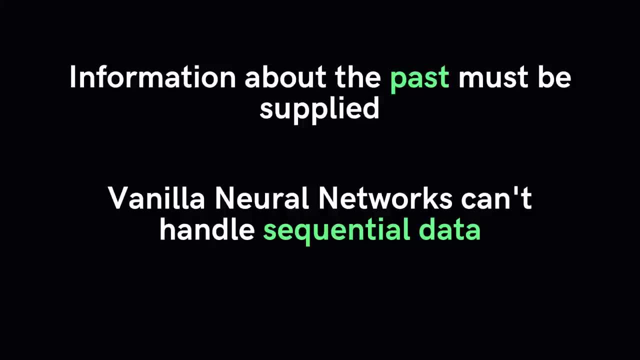 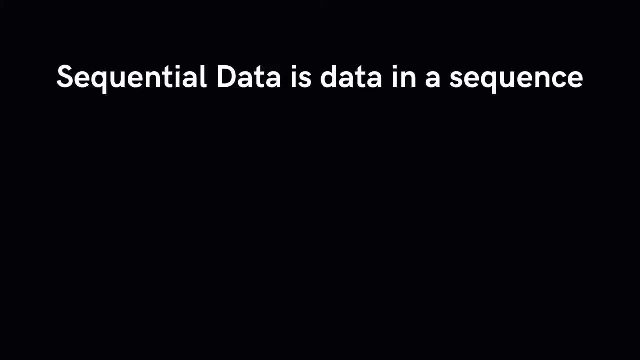 out is that plain vanilla feed-forward neural networks cannot model sequential data. Sequential data is data in a sequence. For example, a sentence is a sequence of words. A ball moving in space is a sequence of all its position states In the sentence that I'd shown you. you understood each word based off your 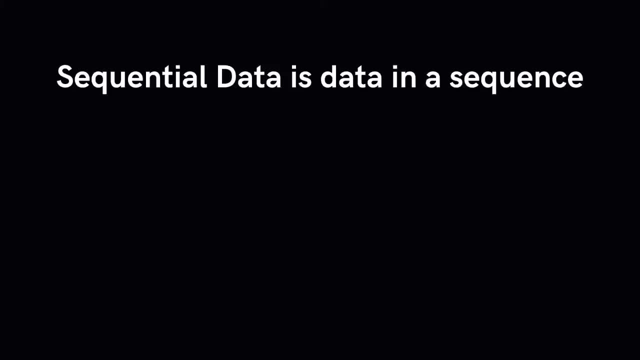 understanding of the previous words. This is called sequential memory. You were able to understand the data point in the sequence by your memory of the previous data point in that sequence. Traditional neural networks can't do this and it seems like a major shortcoming, One of the disadvantages of 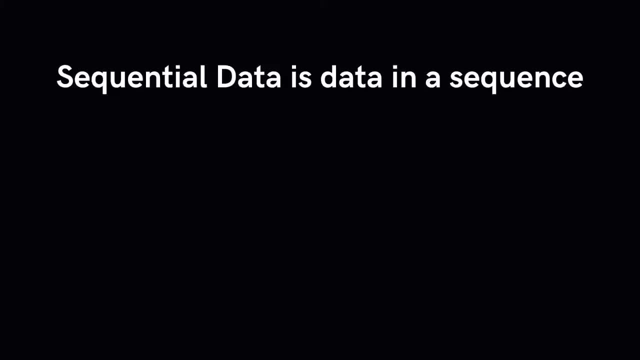 modeling sequences with traditional neural networks is the fact that they don't share parameters across time. Let us take, for example, these two sentences: On Tuesday, it was raining and it was raining on Tuesday. On Tuesday, it was raining and it was raining on Tuesday. 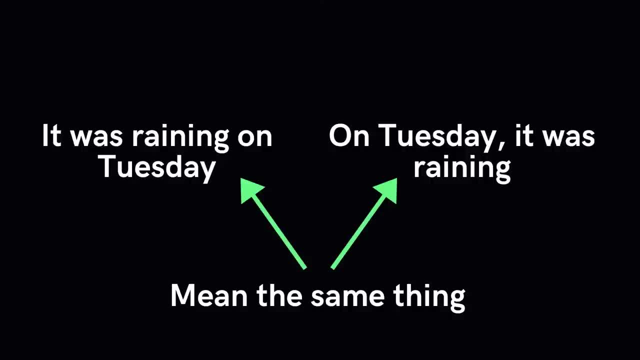 On Tuesday it was raining and it was raining on Tuesday. These sentences mean the same thing, although the details are in different parts of the sequence. Actually, when we feed these sentences into a feed-forward neural network for a prediction task, the model will assign different weights to on Tuesday and it was raining at each moment in time. 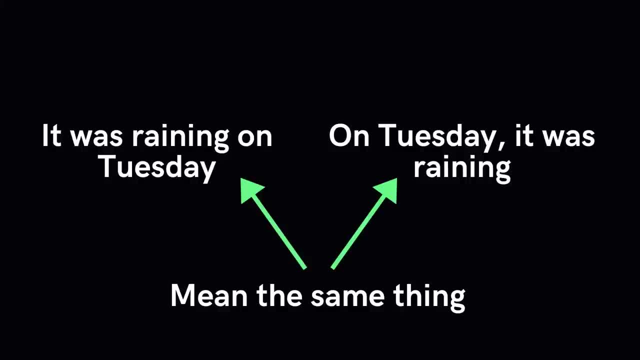 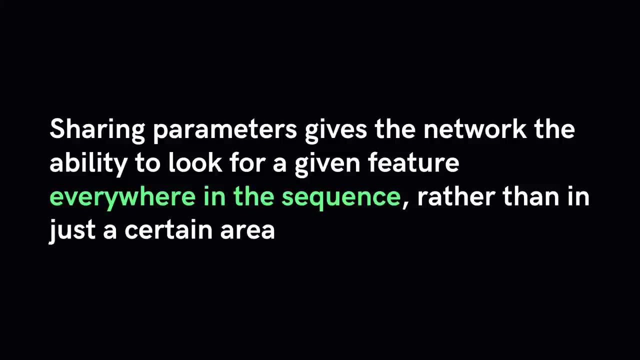 Things we learn about the sequence won't transfer if they appear at different points in the sequence. Sharing parameters gives the network the ability to look for a given feature everywhere in the sequence, and it will be able to look for a given feature everywhere in the sequence. 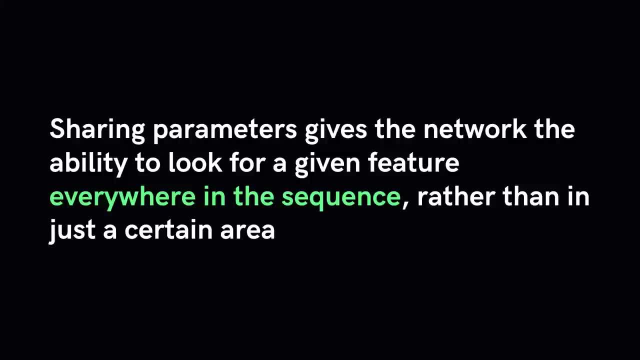 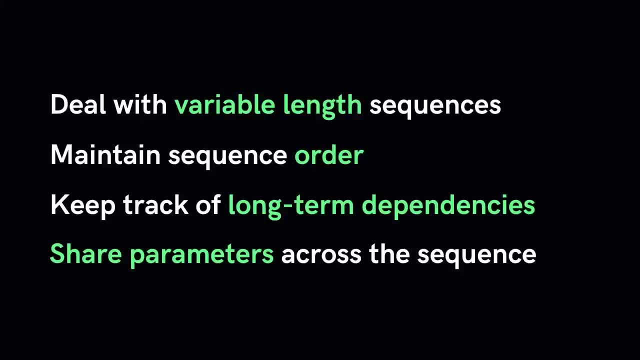 rather than just in a certain area. Thus, to model sequences, we need a specific learning framework able to deal with variable length sequences, maintain sequence order and to keep track of long-term dependencies rather than cutting input data too short, and, finally, to share parameters across the sequence so as to not relearn things. 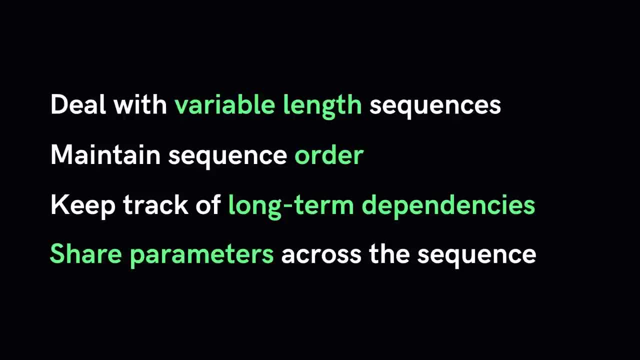 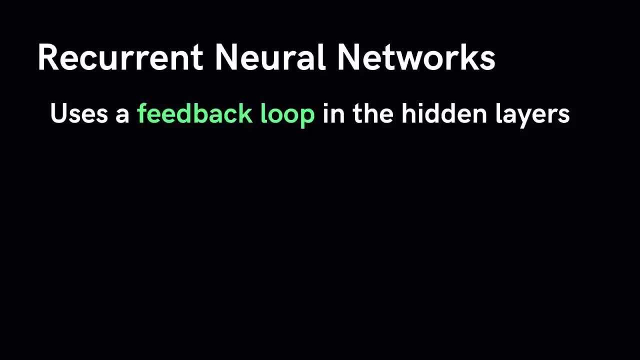 And that's where recurring neural networks come in. RNNs are a type of neural network architecture that use something called a feedback loop in the hidden layer. Unlike feed-forward neural networks, the recurring neural network, or RNN, can operate effectively on sequences of data with variable input length. 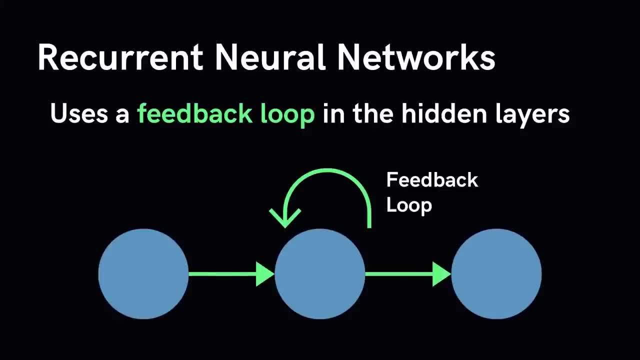 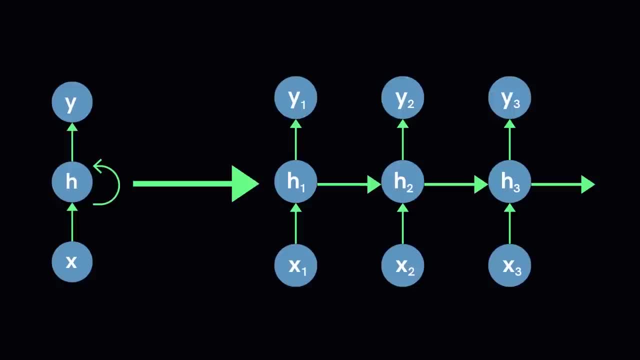 This is how an RNN is usually represented. This little loop here is called the feedback loop. Sometimes you may find the RNNs depicted over time like this: The first path represents the network in the first time step, The hidden node H1. 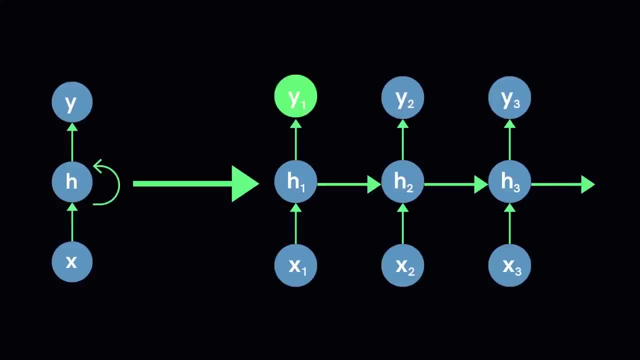 The hidden node H1 uses the input time step. The hidden node H1 uses the input time step to produce output y1.. This is exactly what we've seen with BFF manual networks. However, at the second time step, the hidden node at the current time step H2 uses both the new input, X2,. 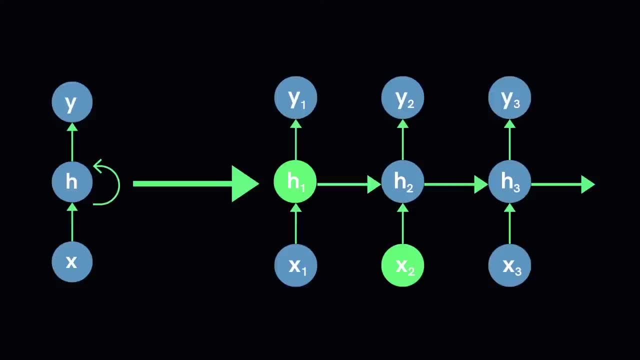 as well as the state from the previous time, step H1 as input to make new predictions. This means that an RNN uses knowledge of its previous states as input for its current prediction, And we can repeat this process for an arbitrary number of states. 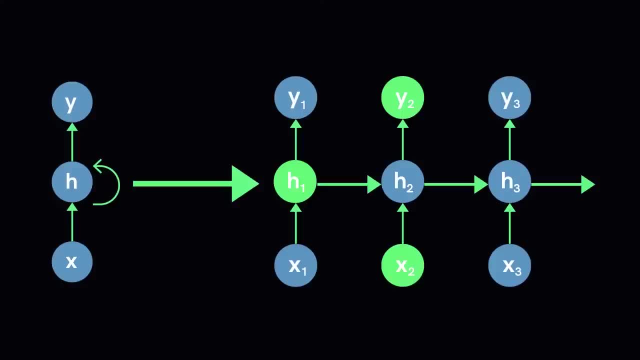 of steps allowing for the network to propagate information by its hidden state throughout time. This is almost like giving a neural network a short-term memory. They have this abstract concept of sequential memory and because of this we're able to model certain areas of data: sequential data. 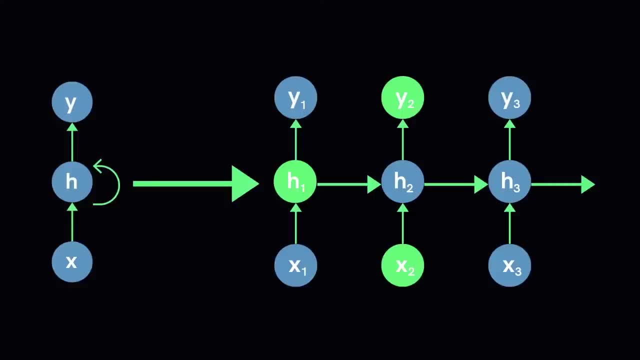 that standalone neural networks aren't able to model. Recurrent neural networks remember their past and their decisions are influenced by what it has learned from the past. Basic feedforward networks remember things too, but they remember things they learned during training. For example, an image classifier learns what a 3R looks like. 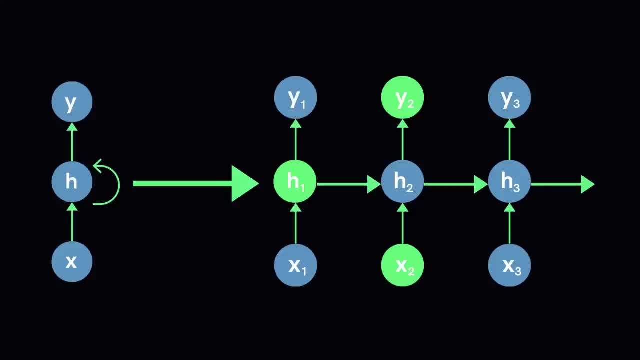 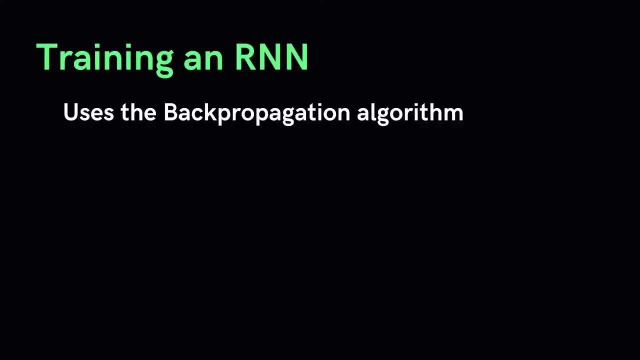 during training and then uses that knowledge to classify things in production. So how do we train an RNN? Well, it is almost the same as training a basic, fully connected feedforward network, except that the back propagation algorithm is applying for every sequence data point rather than the entire sequence. 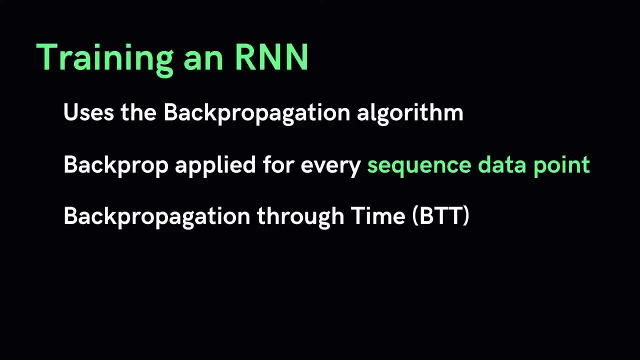 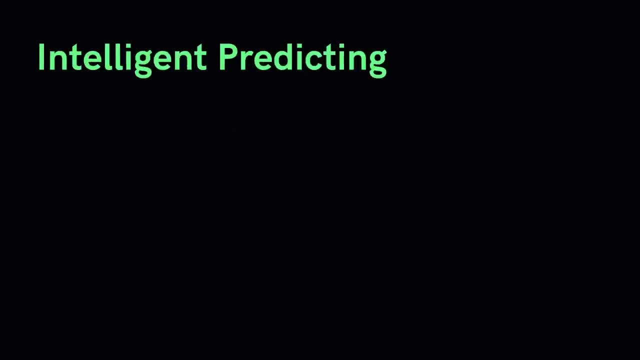 This algorithm. The algorithm is sometimes called the Backpropagation Through Time algorithm or the BTT algorithm. To really understand how this works, imagine we're creating a recurring new network to predict the next letter a person is likely to type based on the previous letters they've 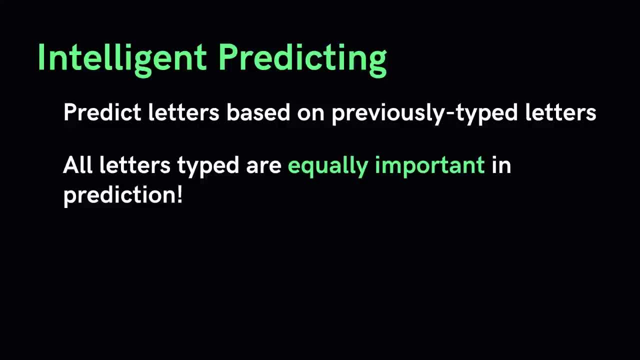 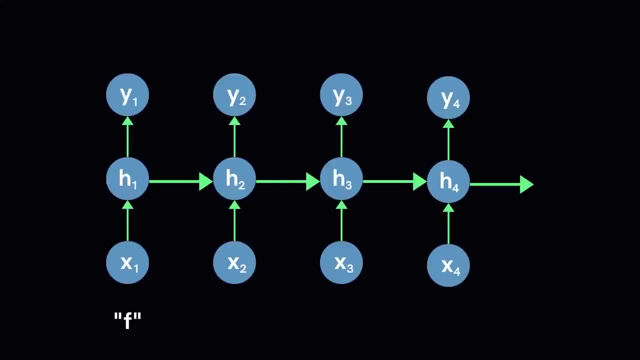 already typed. The letter that a user just typed is quite important to predicting the new letter. However, all the previous letters are also very important to this prediction as well. At the first time step, say, the user types the letter f so our network might predict. 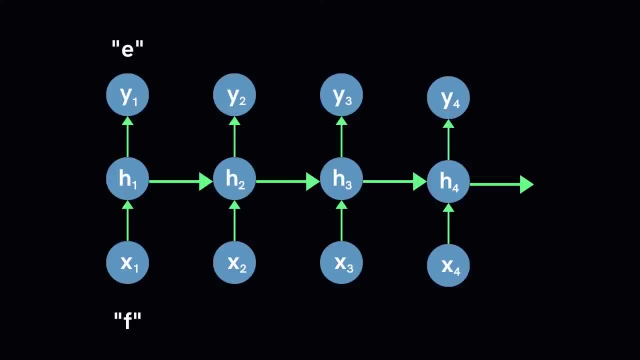 that the next letter is an e. based on all of the previous training examples that included the word fe. At the next time step, the user types the letter r, so our network uses both the new letter r plus the state of the first hidden neuron in order to compute the next prediction. 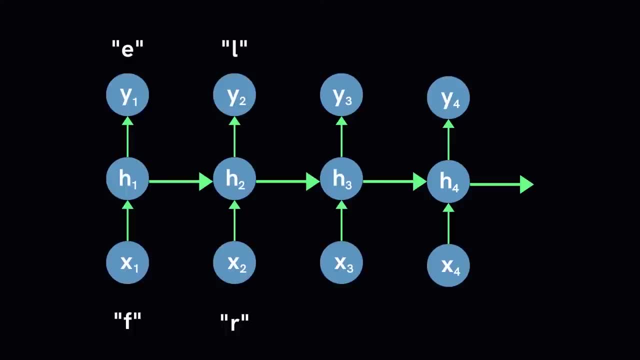 l. The network predicts this because of the high frequency of occurrences in the word fel in our training dataset. Adding the letter a might predict the letter t. adding an n would predict the letter k, which would match the word our user intended to type, which is frank. 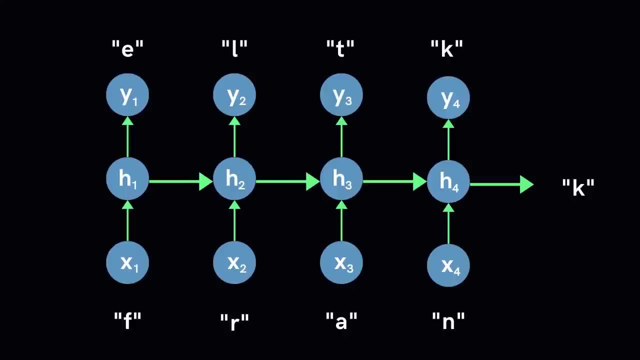 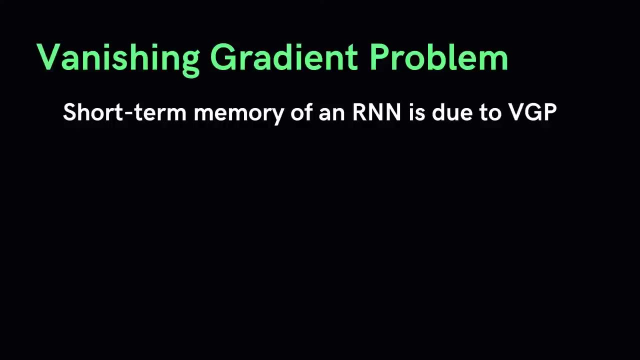 There, however, is an issue with RNNs, known as short term memory. Short term memory is caused by the infamous vanishing and exploding gradient problems. As the RNN processes more words, it has trouble retaining information from previous steps, kind of like our memory. 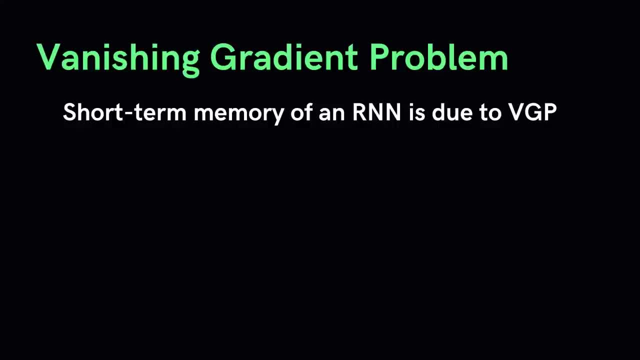 If you're given a long sequence of numbers like pi and you try reading them out, it's probably going to forget the initial few digits right. Short term memory and the vanishing gradient is due to the nature of back propagation, the algorithm used to train and optimize neural networks. 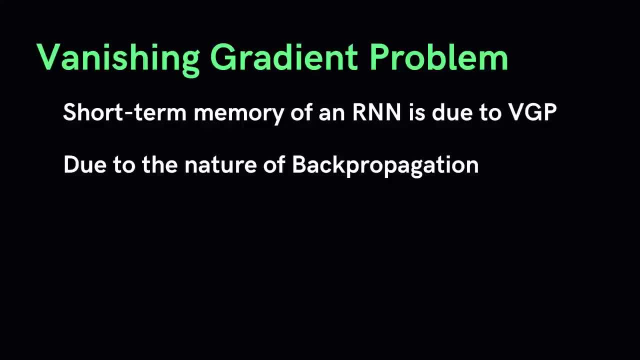 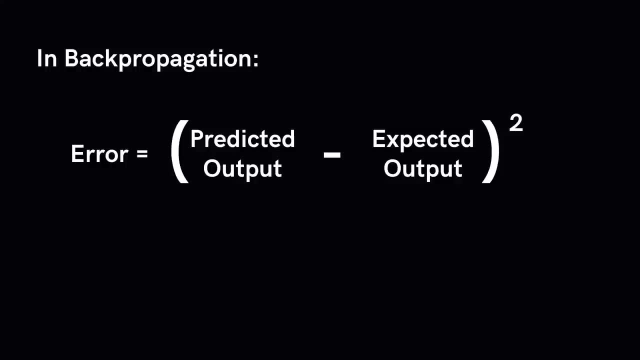 After the forward propagation or the pass, the network compares this prediction to the ground truth using a loss function, which outputs an error value, an estimate of how poorly the network is performing. The network uses that error value to perform back propagation, which calculates the error. 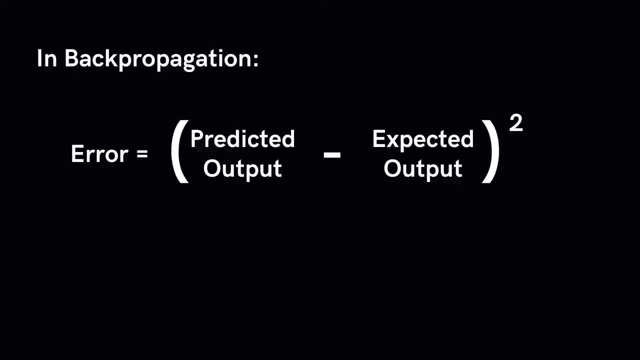 value for each node in the network. The gradient is a value used to adjust the network's internal weights, allowing for the network to learn. The bigger the gradient, the bigger the adjustments are, and vice versa. Here's where the problem lies. 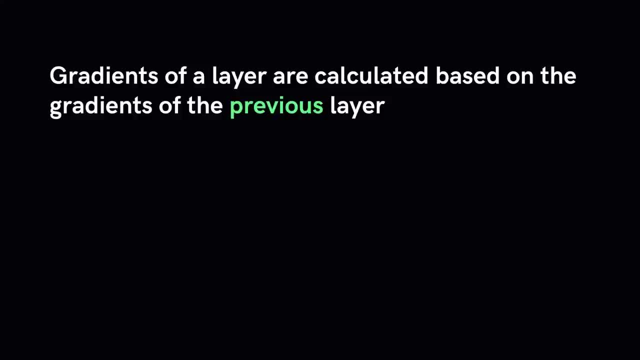 When performing back propagation, each node in a layer calculates its gradient with respect to the effects of the gradient in the layer before it. So if the adjustment to the layers before it is small, then the adjustments to the current layer will be even smaller. 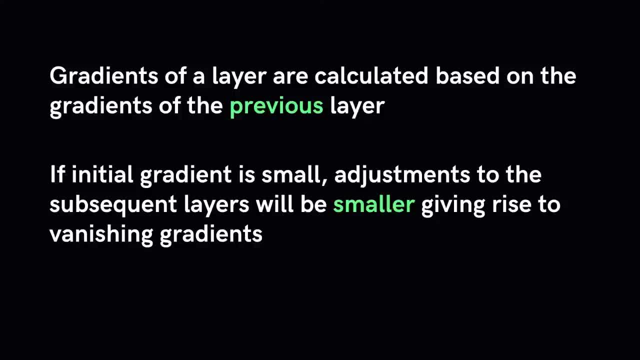 And this causes gradients to exponentially shrink as it back propagates down. The earlier layers fail to do any learning, as the internal weights are barely being adjusted due to extremely small gradients, And that is the vanishing gradient problem. Let's see how this applies to recurrent neural networks. 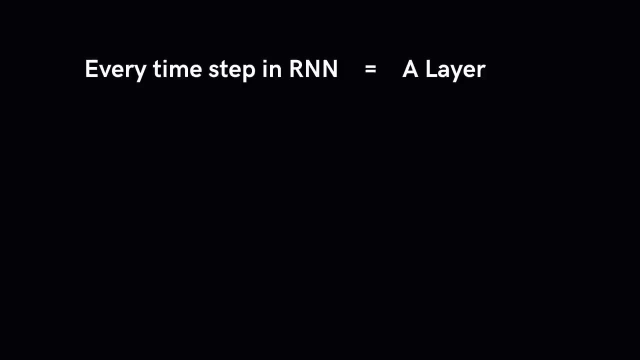 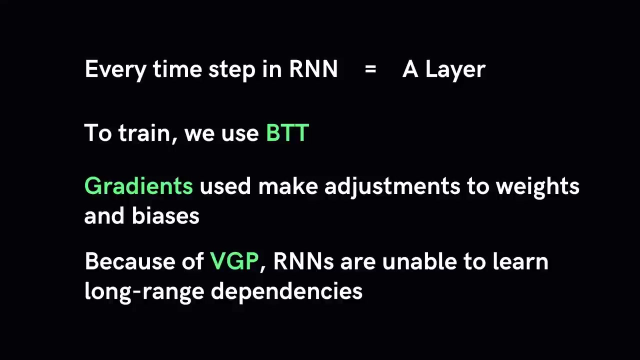 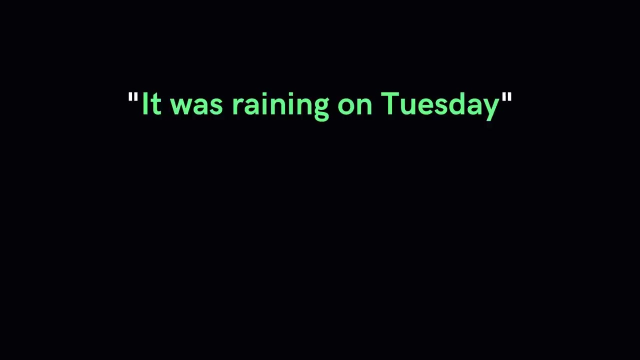 You can think of each time step in a recurrent neural network as a layer. To train a recurrent neural network you use an application of back propagation called back propagation through time. awaa. 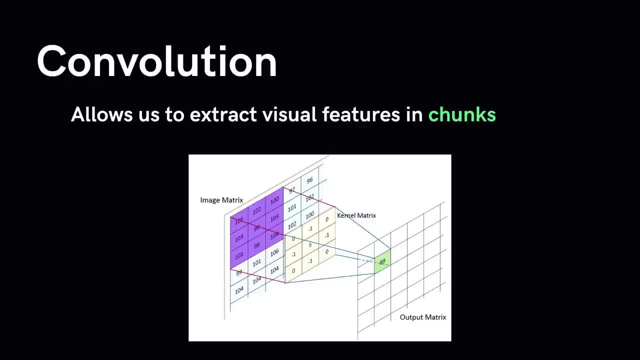 Each neuron in a convolution layer is responsible for a small cluster of neurons in the preceding layer. The bounding box that determines the cluster of neurons is called a filter, also called a kernel. Conceptually you can think of it as a filter moving across an image. 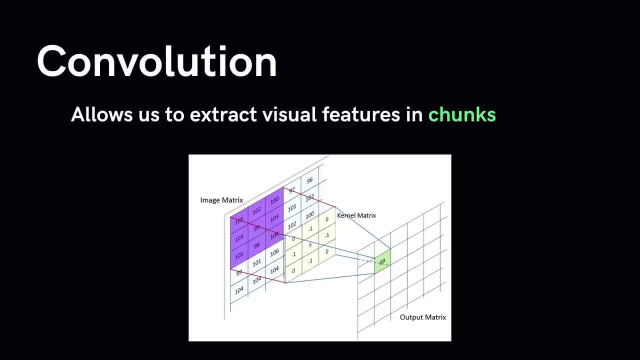 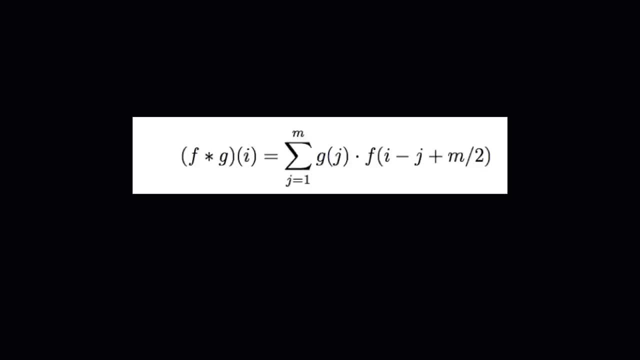 and performing a mathematical operation on individual regions of the image. It then sends its result to the corresponding neuron in the convolution layer. Mathematically, a convolution of two functions, f and g, is defined as follows, which is in fact the dot product of the input function and the kernel function. 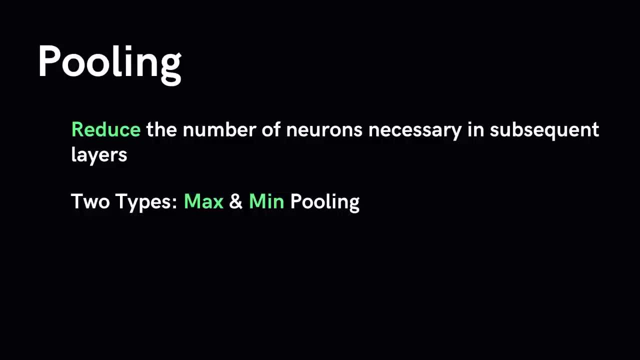 Pooling, also known as subsampling or downsampling, is the next step in a convolutional neural network. Its objective is to further reduce the number of neurons necessary in subsequent layers of the network, while still retaining the most important information. There are two different types of pooling that can be performed. 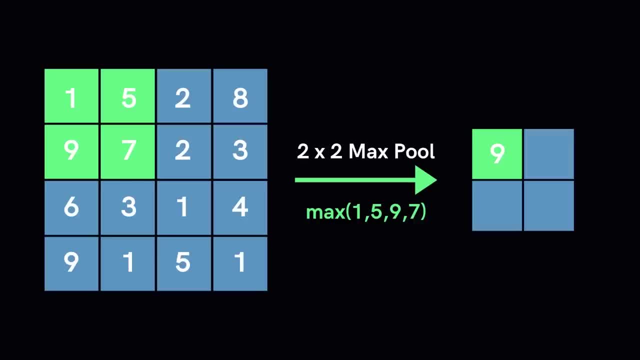 Max pooling and min pooling. As the name suggests, max pooling is based on picking up the maximum value from the selected region, and min pooling is based on picking up the minimum value from that region. When we put all these techniques together, we get an architecture for a deep neural network. 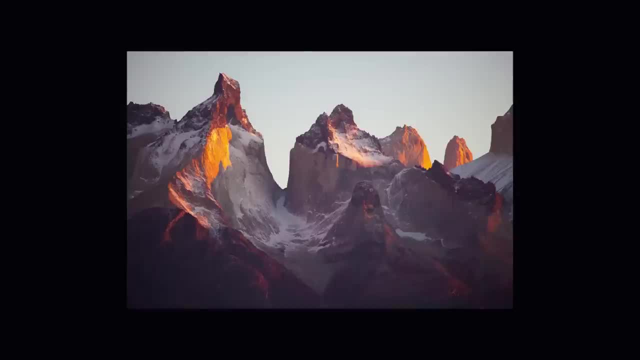 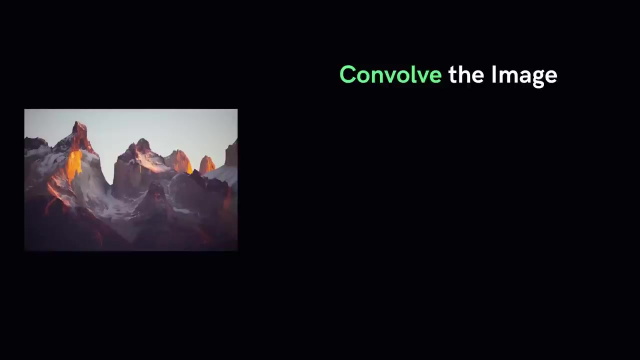 quite different from a fully connected neural network For image classification, where CNNs are used heavily. we first take an input image, which is a two-dimensional matrix of pixels, typically with three color channels. Next, we use a convolution layer with multiple filters to create a two-dimensional feature. 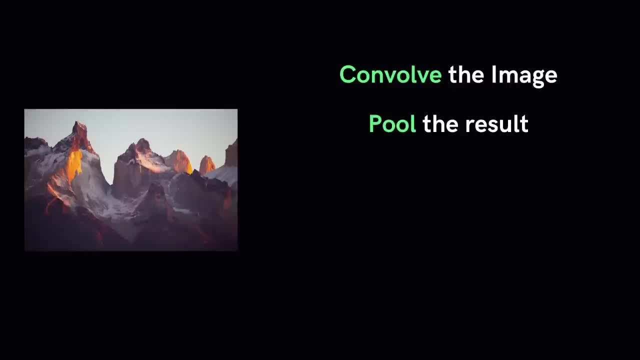 matrix as the output for each filter. We then pool the results to produce a downsample feature matrix for each filter in the convolution layer. Next we typically repeat the convolution and pooling steps multiple times, using previous features as input. Then we add a few fully connected hidden layers to help classify the image. 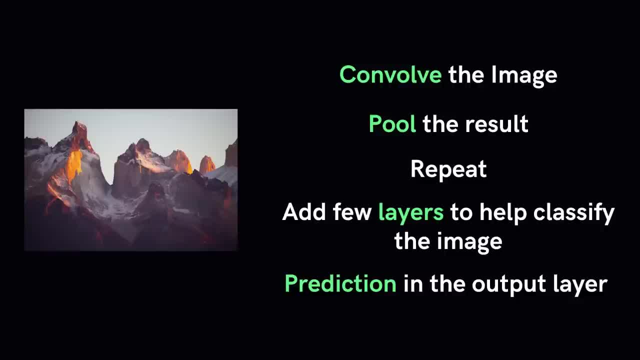 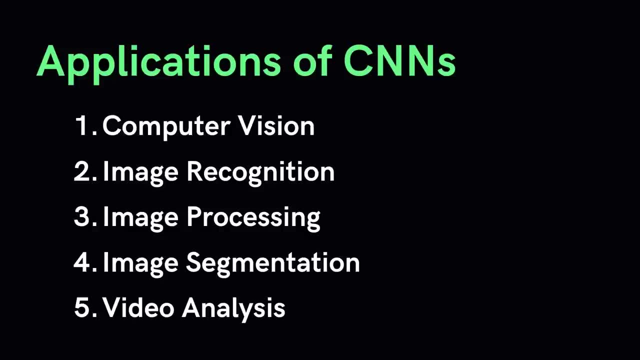 Finally, we produce a classification prediction in the output layer. Convolutional neural networks are used heavily in the field of computer vision and work well for a variety of tasks, including image recognition, image processing, image segmentation, video analysis and natural language processing. 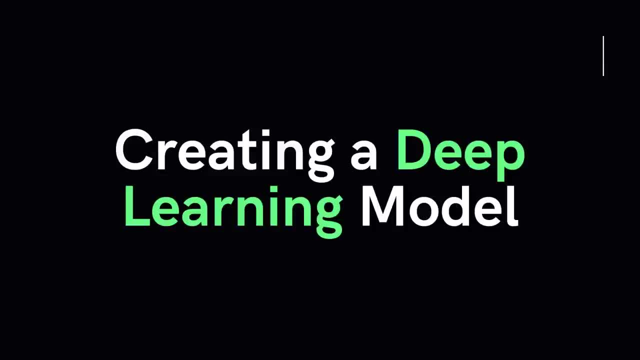 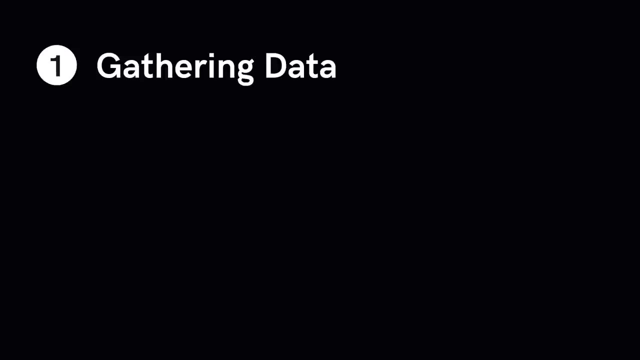 In this section, I'm going to discuss the five steps that are common in every deep learning project that you build. These can be extended to include various other aspects, But at its very core, they are very fundamentally five steps. Data is at the core of what deep learning is all about. 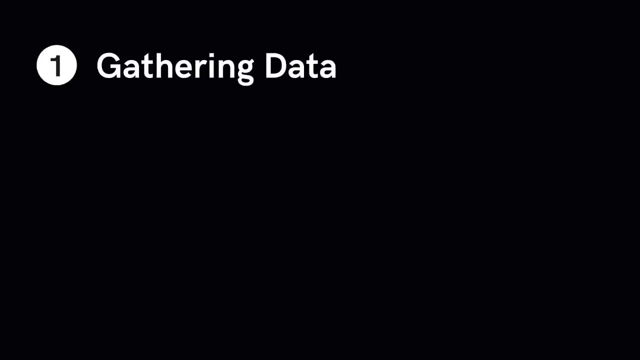 Your model will only be as powerful as the data you bring. Which brings me to the first step: gathering your data. The choice of data and how much data you would require entirely depends on the problem you're trying to solve. Picking the right data is key, and I can't stress how important this part is. 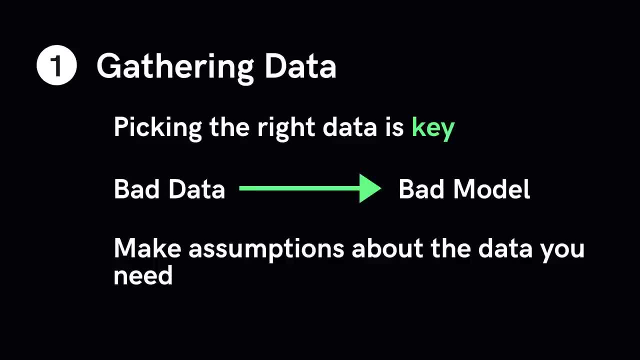 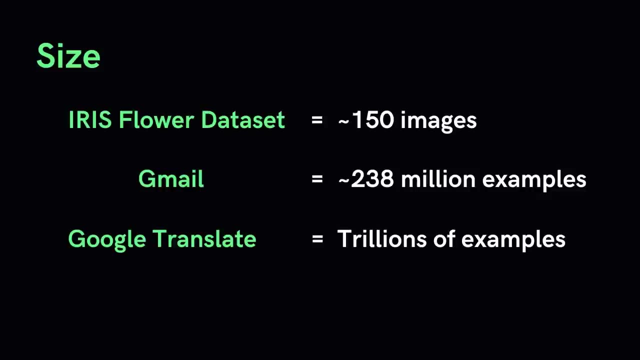 Bad data implies a bad model. A good rule of thumb is to make assumptions about the data you require and be careful to record these assumptions so that you can test them later if needed. Data comes in a variety of sizes. For example, Iris flower dataset contains about 150 images in the total set. 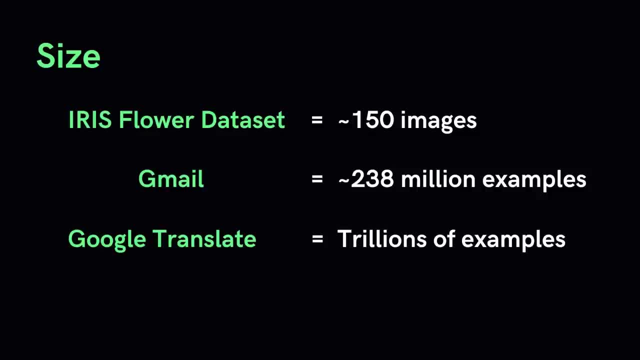 Gmail Smart Reply has around 238 million examples in its running set, and Google Translate reportedly has trillions of data points. When you're choosing your dataset, this is the first step. The second step is to make assumptions about the data you require and be careful to record. 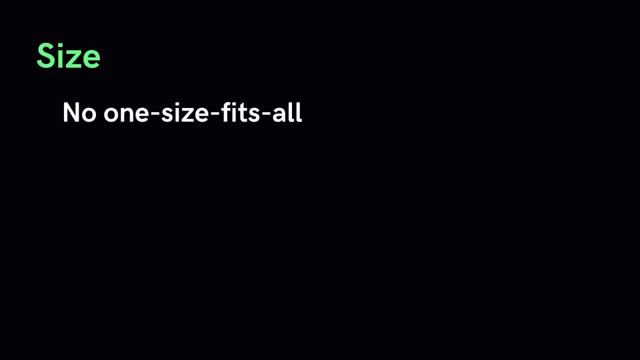 these assumptions so that you can test them later if needed. In general, this data is not exactly a one-size-fits-all, but the general rule of thumb is that the amount of data you need for a well performing model should be 10 times the number of parameters. 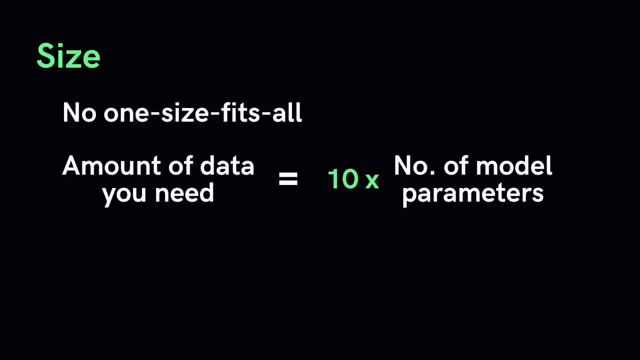 in that model. However, this may differ from time to time depending on the type of model you're building. For example, in regression analysis you should use around 10 examples per predictor variable For image classification. the minimum you should have is around a 1000 images per class. 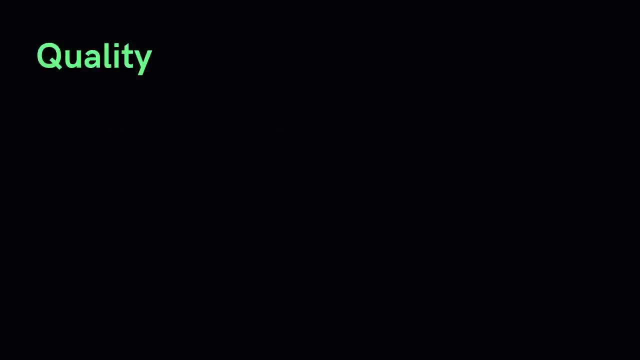 that you're trying to classify. While quantity of data matters, quality matters. Quality matters too. There is no use having a lot of data if it's bad data. There are certain aspects of quality that tend to correspond to well-performing models. 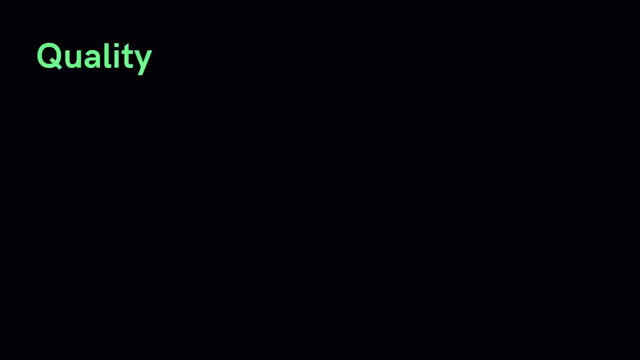 One aspect is reliability. Reliability refers to the degree in which you can trust your data. A model trained on a reliable dataset is more likely to yield useful predictions than a model trained on unreliable data. How common are label errors? If your data is labeled by humans, sometimes there may be mistakes. 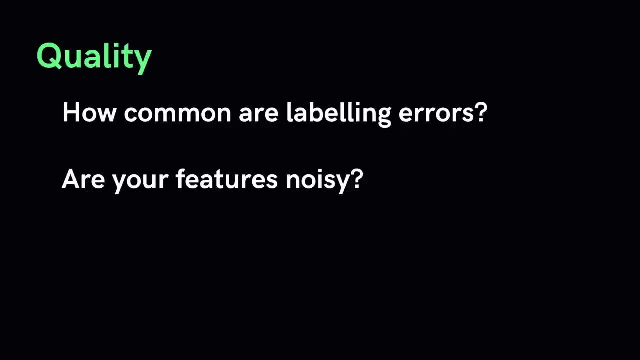 Are your features noisy? Is it completely accurate? Some noise is alright. you'll never be able to purge your data of all the noise. There are many other factors that determine quality For the purpose of this video, though I'm not going to talk about the remaining. 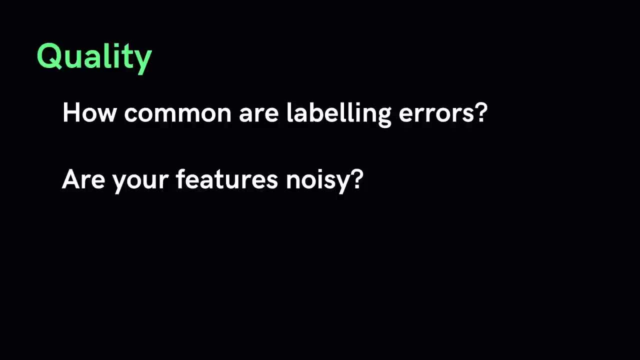 Although, if you're interested, I'll leave them in the show notes below. Luckily for us, there are plenty of resources on the web that offer good datasets for free. Here are a few sites where you can begin your dataset search. The UCI Machine Learning Repository maintains around 500 extremely well-maintained datasets. 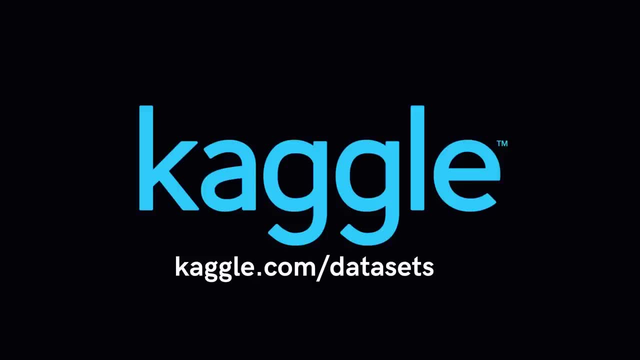 that you can use in your deep learning projects. Kaggle is another one. You'll love how detailed their datasets are. They give you info on the features, data types, number of records and so on. You can use their kernel too, and you wouldn't have to download the dataset. 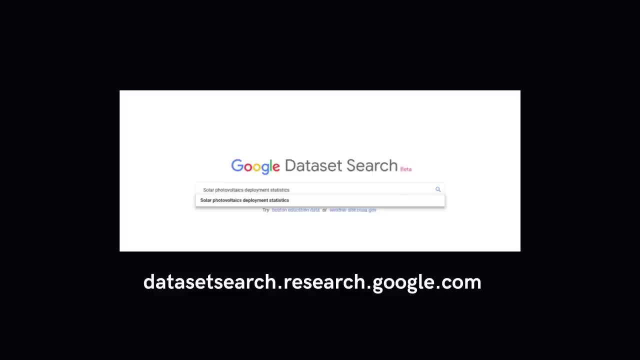 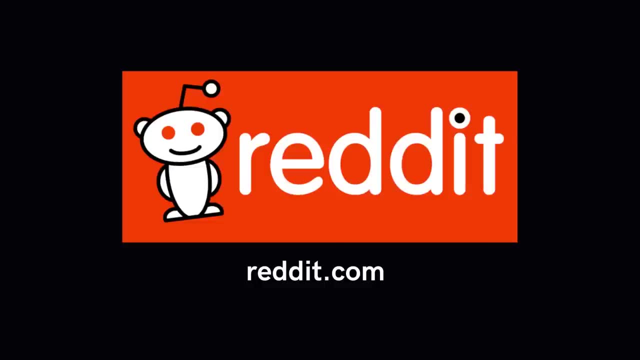 Google's dataset search is still in beta, but it's one of the most amazing sites that you can find today. Reddit, too, You can place a request for datasets you want, but again there is a chance of it not being properly organized. 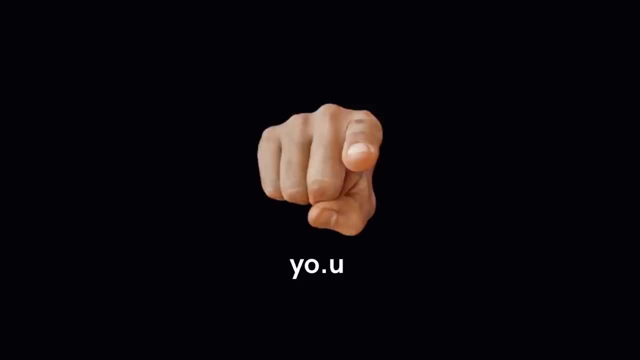 Create your own dataset. That'll work too. You can use web scrapers like Beautiful Soup to get your required data for the dataset. After you've selected your dataset, you now need to think of how you're going to use this data. There are some common pre-processing steps that you should follow. 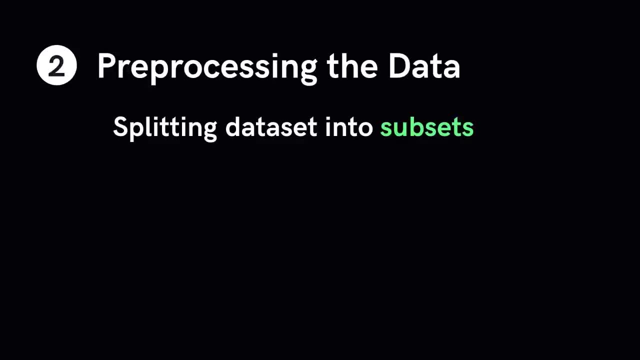 First splitting the dataset into subsets. In general, we usually split a dataset into sub-sets. In general, we usually split a dataset into sub-sets. In general, we usually split a dataset into 3 parts: training, testing and validating. 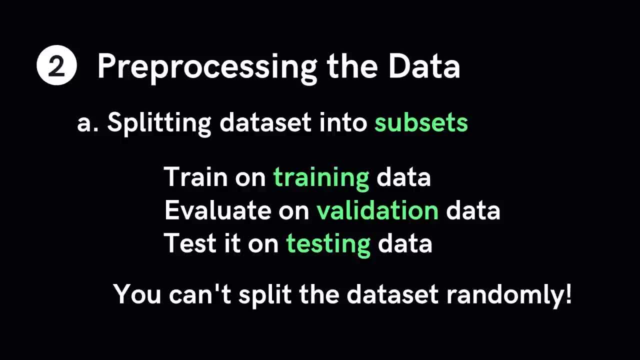 sets. We train our models with the training set, evaluate it on the validation set and finally, once it's ready to use, test it one last time on the testing dataset. Now it's reasonable to ask the following question: Why not have two sets, training and testing? 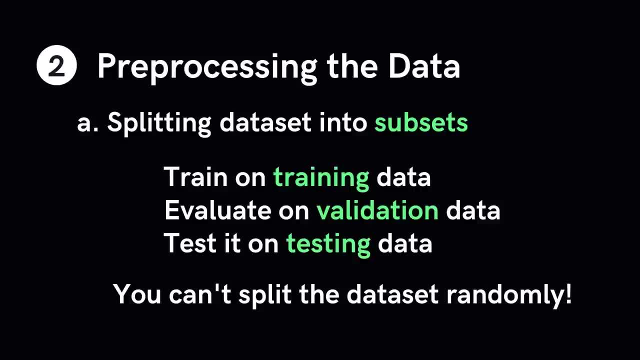 In that way, the process will be much simpler: Just train the model on the training data and test it on the testing data. The answer to that is developing a model that will be able to do this much better. We don't need to process your model. 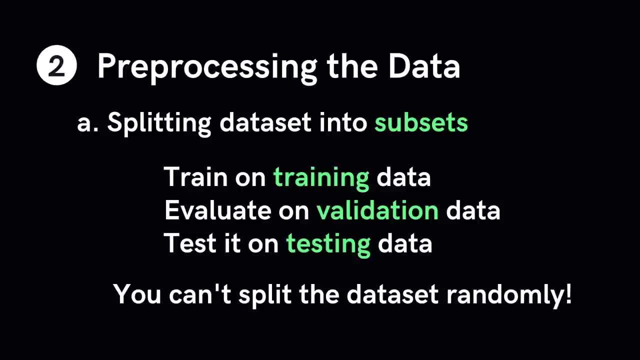 We just have to train it on. the testing dataset model involves tuning its configuration, In other words choosing certain values for the hyperparameters or the weight and biases. This tuning is done with the feedback received from the validation set and is, in essence, a form of learning. 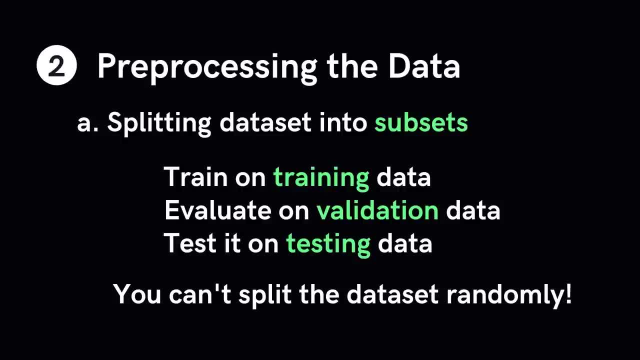 It turns out we just can't split the data set randomly. Do that and you'll get random results. There has to be some kind of logic to split the data set. Essentially, what you want is for all three sets: the training, testing and 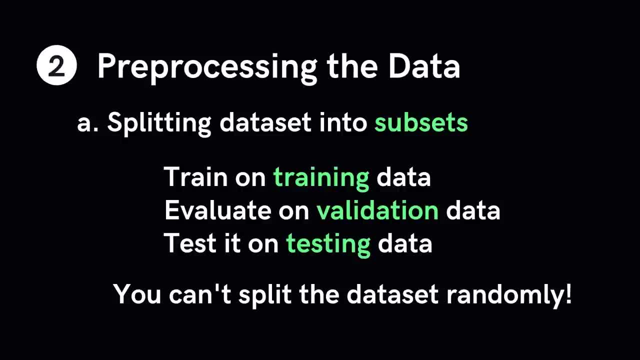 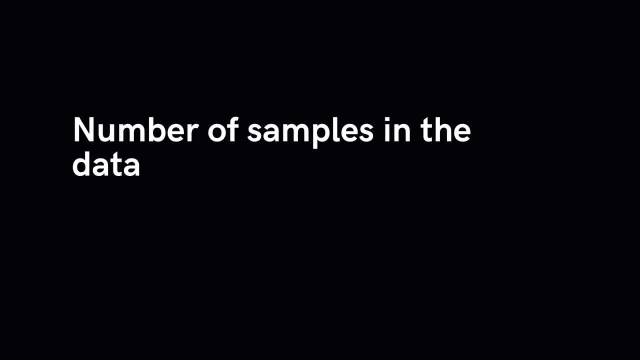 validation sets to be very similar to each other and to eliminate skewing as much as possible. This mainly depends on two things: The first, the total number of samples in your data and the second, well, the actual model you're trying to train. 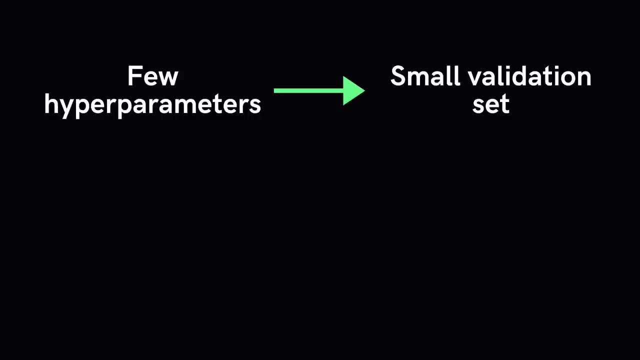 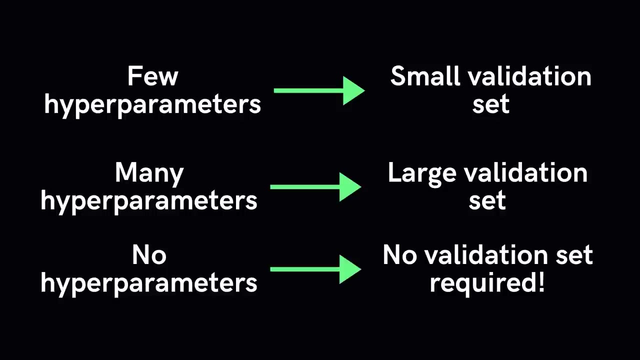 Models with very few hyperparameters will be very easy to validate and tune, So you can probably reduce the size of your validation set. But if your model has many hyperparameters, you would want to have a large validation set as well as consider a cross-validation. Also, if you happen to have a model with no hyperparameters whatsoever, 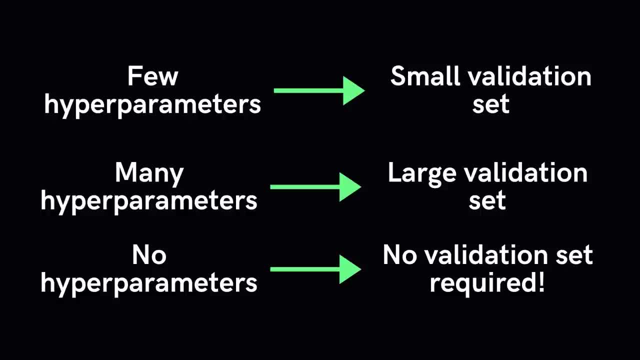 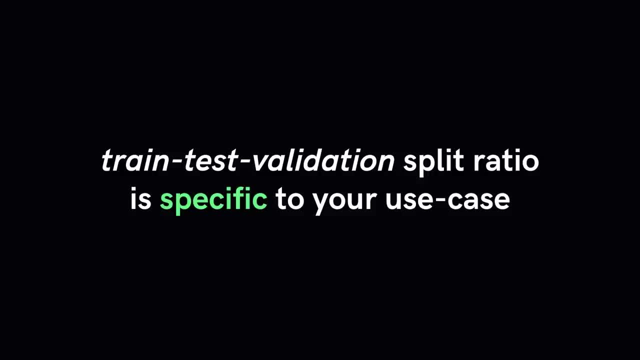 or ones that cannot be easily tuned, you probably don't need a validation set. All in all, like many other things in machine learning and deep learning, the train-test validation split ratio is also quite specific to your use case and it gets easier to make. 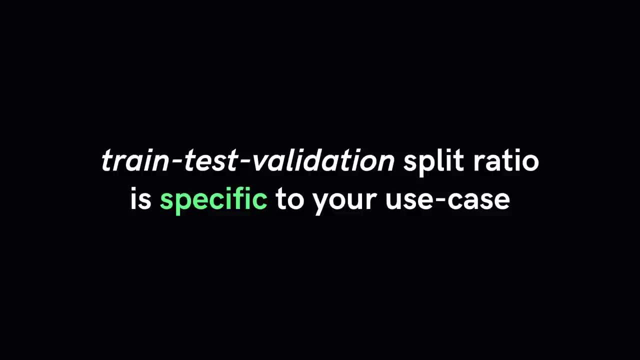 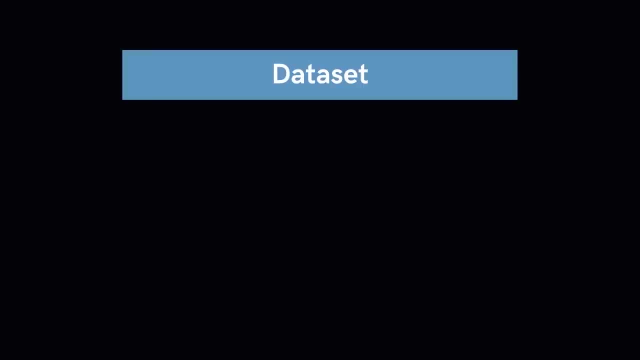 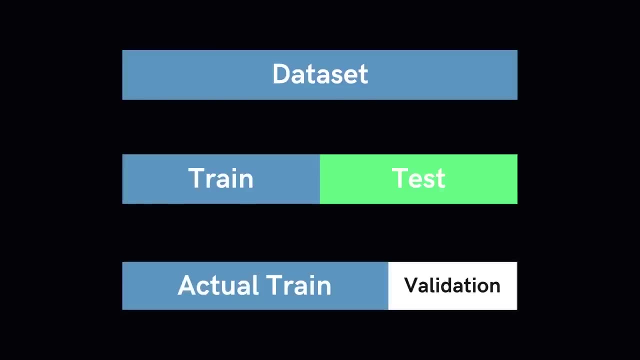 judgment as you train and build more and more models. So here's a quick note on cross-validation. Usually you'd want to split your dataset into two: the train and the test. After this, you keep the test set aside and choose some percentage of the training set to be the actual. 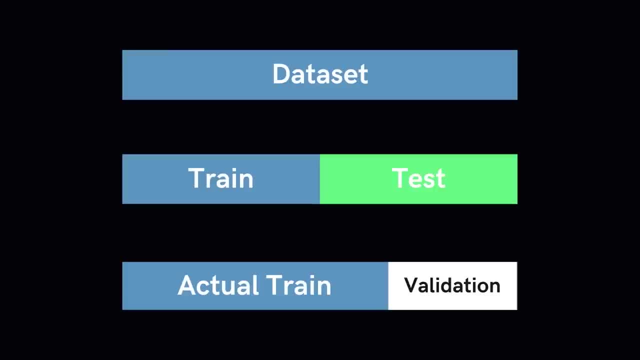 trained set and the remaining to the validation set. The model is then iteratively trained and validated on those different sets, And there are multiple ways to do this, and this is commonly known as cross-validation. Basically, you use your training set to generate. 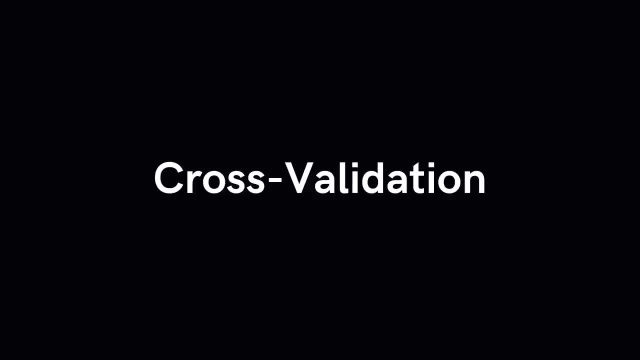 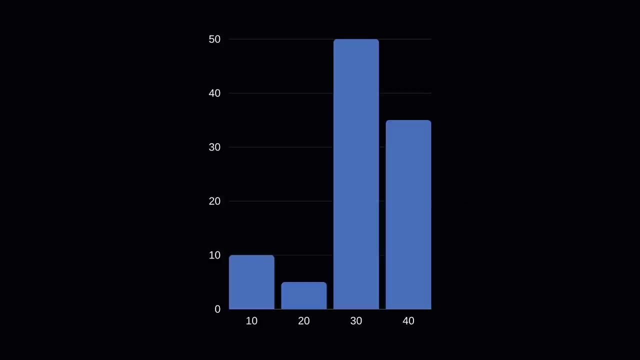 multiple splits of the train and validation set. Cross-validation avoids overfitting and is getting more and more popular, with k-fold cross-validation being the most popular method. Additionally, if you're working on time series data, a frequent technique is to split the data by time. For example, if 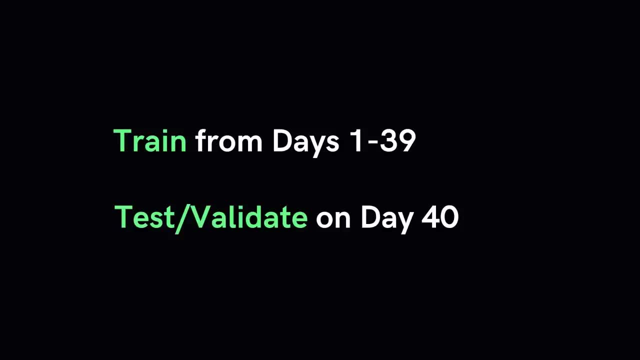 you have a data set with 40 days of data. you can train your data from days 1 to 39 and evaluate your model on the data from day 40.. For systems like this, the training data is older than the serving data, so this technique ensures your. 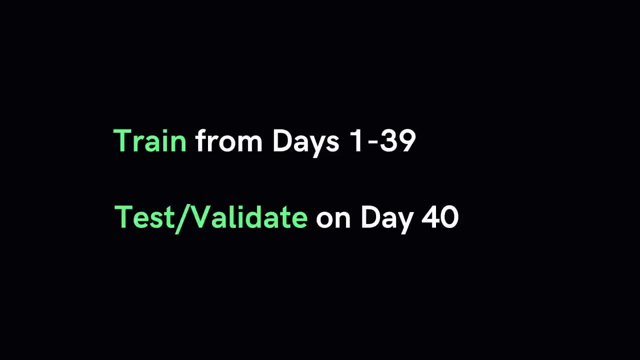 validation set mirrors the lag between training and serving. However, keep in mind that time-based splits work best for very, very large data sets, such as those with tens of millions of examples. The second method that we have in pre-processing is formatting. The data set you've picked might not be in the 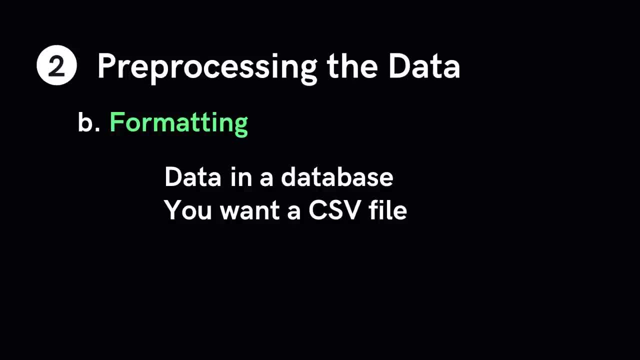 right format that you like. For example, the data might be in the form of a database, but you'd like it as a CSV file. vice versa, Of course. there are a couple of ways to do this, and you can Google them if you'd like. Dealing with missing data is one of the most challenging steps in the 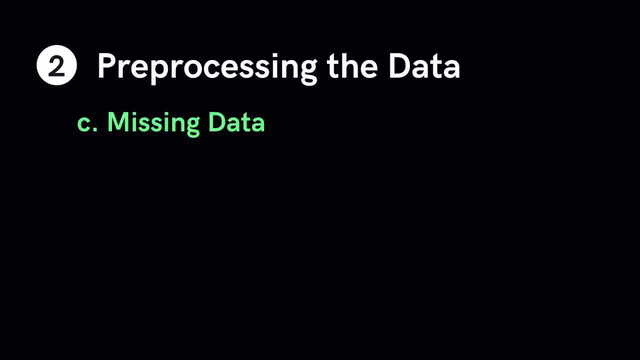 gathering of data for your deep learning projects. Unless you're extremely lucky to land with the perfect data set, which is quite rare, dealing with missing data will probably take a significant chunk of your time. It is quite common in real world problems to miss some values of our data samples. This may be due to 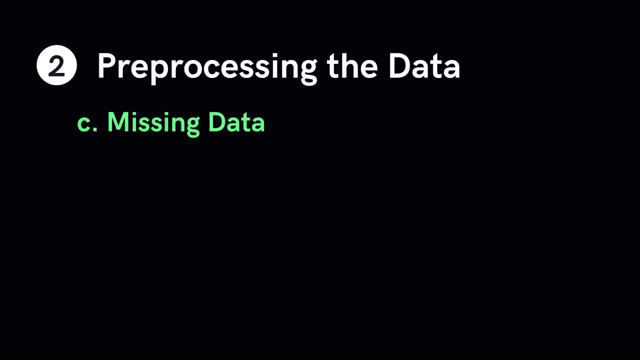 errors on the data collection, blank spaces on surveys, measurements not applicable, and so on. Missing values are typically represented with the NAN or the null indicators. The problem with this is that most algorithms can't handle these kind of missing values, so we need to take 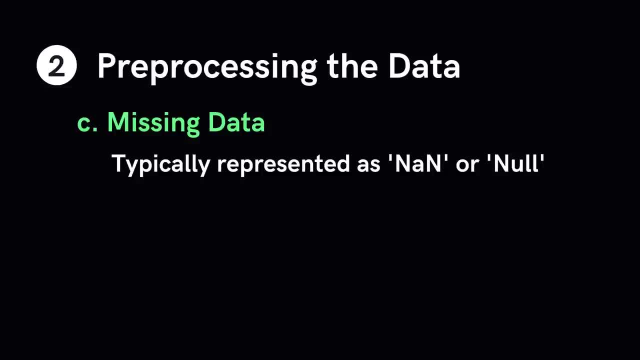 care of them before feeding data to our models. There are a couple of ways to deal with them. One is eliminating the samples of the features with missing values. The downside, of course, is that you risk to delete relevant information. The second step is to impute the missing data. 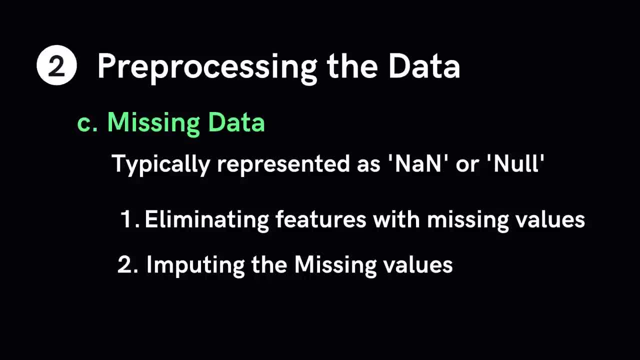 A common way is to set the missing values as the mean value for the rest of the samples, But of course there are other ways to deal with specific data sets. Be smart, as handling missing data in the wrong way can spell disasters. Sometimes you may have too much data than what you require More. 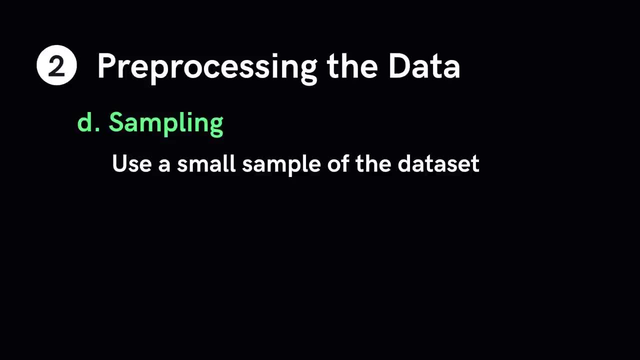 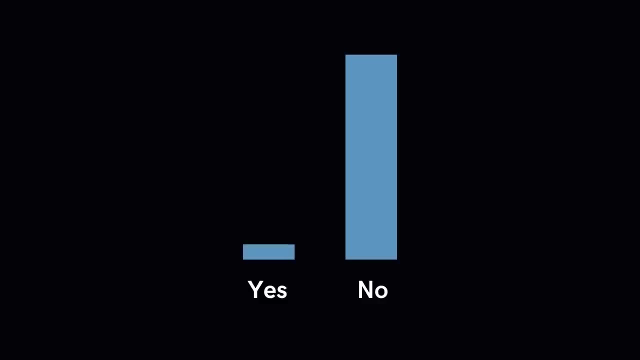 data can result in larger computational and memory requirements. In cases like this, it's best practice to use a small sample of the data set. It will be faster and ultimately, an increase in time for you to explore and prototype solutions In most real-world data sets you're going to 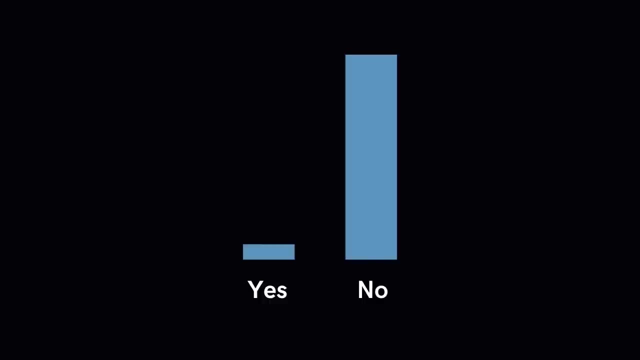 come across imbalanced data, That is, classification data that has skewed class proportions, leading to the rise of a minority class and a majority class. If we train a model on data like this, a model will only spend time learning about the majority class and a lot less time on the minority class, And hence a 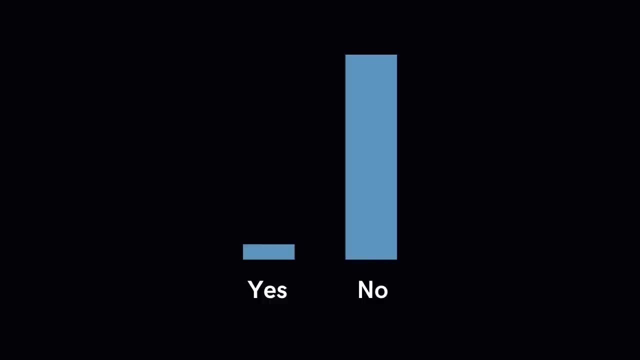 model will ultimately be biased to the majority class, And so, in cases like this, we usually use a process called down sampling and up weighting, which is essentially reducing the majority class by some factor and adding example weights of that factor to the down sample class. For example, if we down sample, the 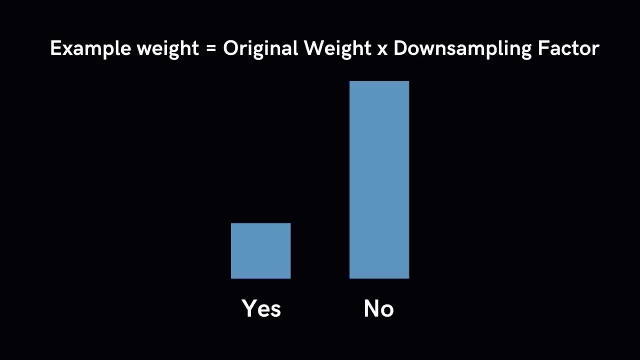 majority class by a factor of 10, then the example weights we add to that class should be 10.. It may seem odd to add example weights after down sampling. What is its purpose? Well, there are a couple of reasons. It leads to faster convergence. 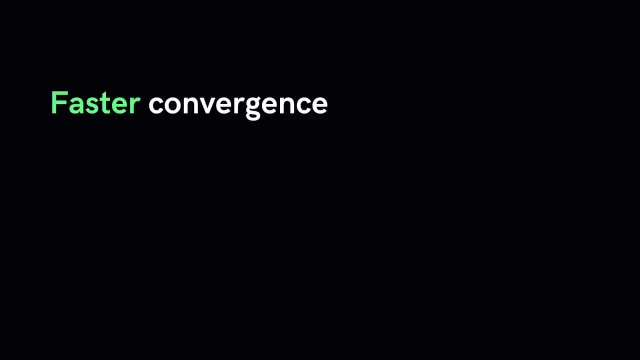 Meaning. we see the minority class more often, which helps the model converge faster By consolidating the majority class into fewer examples with larger weights, we spend less disk space storing them. Up weighting ensures that model is still calibrated. We add up weighting after down sampling so as to keep the 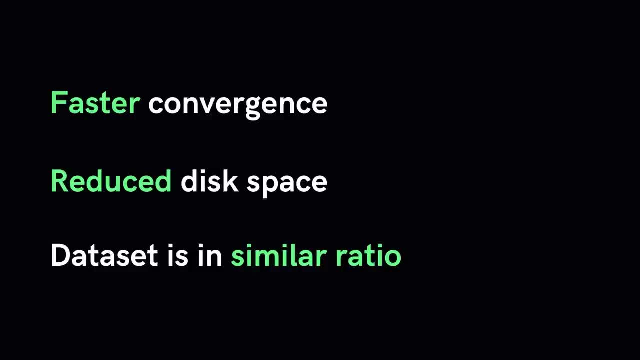 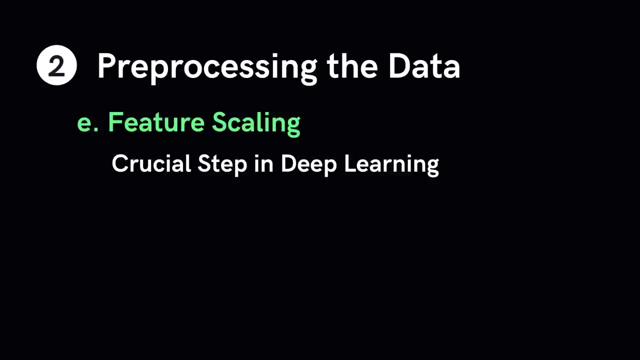 data set in similar proportion. These processes essentially help a model see more of the minority class rather than just solely the majority class. This helps our model perform better in real-world situations. Feature scaling is a crucial step in the pre-processing phase, as the majority of the deep learning. 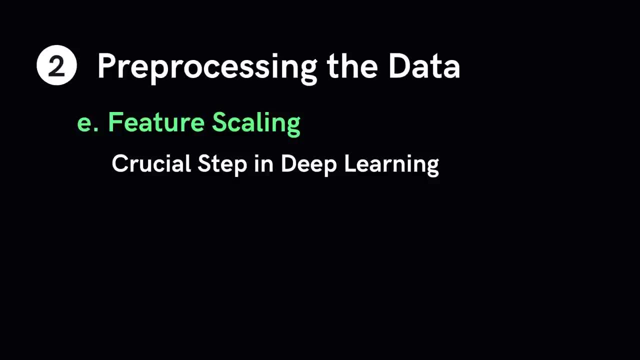 algorithms perform much better when dealing with features that are on the same scale. The most common techniques are normalization, which refers to the rescaling of features to a range between 0 and 1, which, in fact, is a special case of min-max scaling. To normalize our data, we need to apply min-max scaling to each. 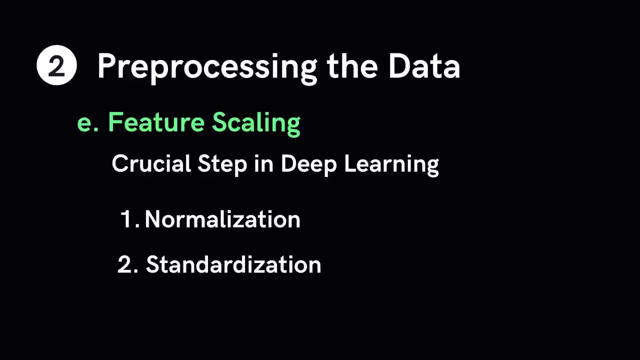 feature column Standardization consists of centering the field at mean 0 with standard deviation 1, so that the feature columns have the same parameters as a standard normal distribution, That is, zero mean and unit variance. This makes it much easier for the learning algorithms to learn the weights of the 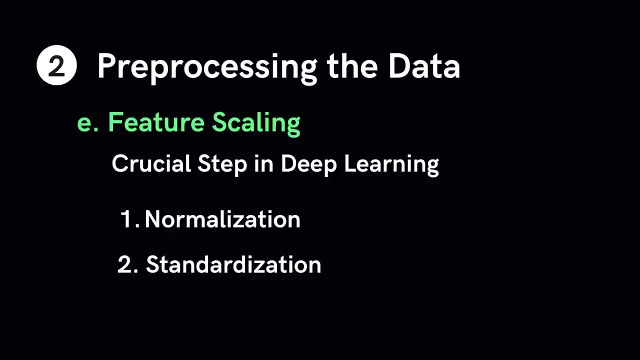 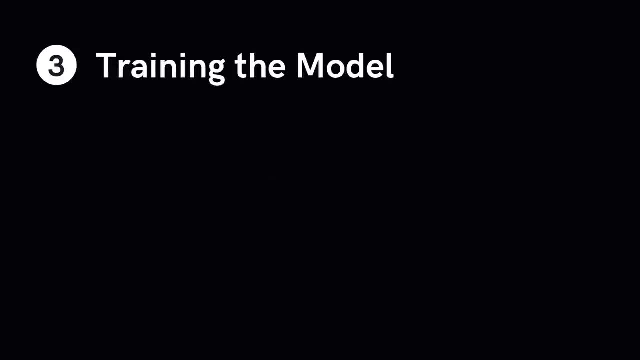 parameters. In addition, it keeps useful information about outliers and makes the algorithms less sensitive to them. Once the data has been prepared, we now feed this into our network to trade. We've discussed the learning process of a neural network in the previous module, so if you aren't sure, I'd advise you to watch that module first. But essentially, 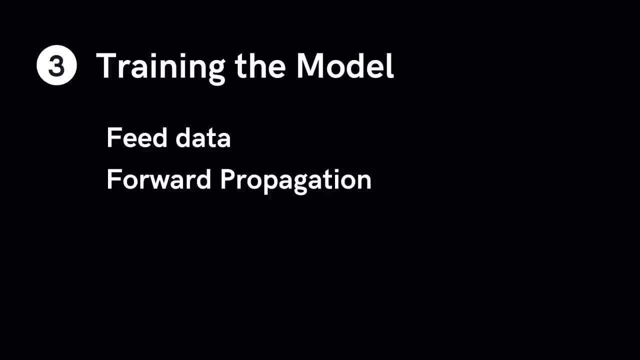 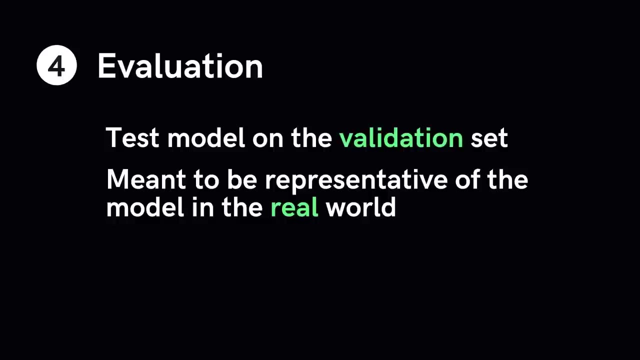 once the data has been fed forward, propagation occurs and the loss is compared against the loss function and the parameters are adjusted based on this loss incurred. Again, nothing too different from what we discussed previously. Your model has successfully trained, Congratulations. Now we need to test how good our model is using the validation set. 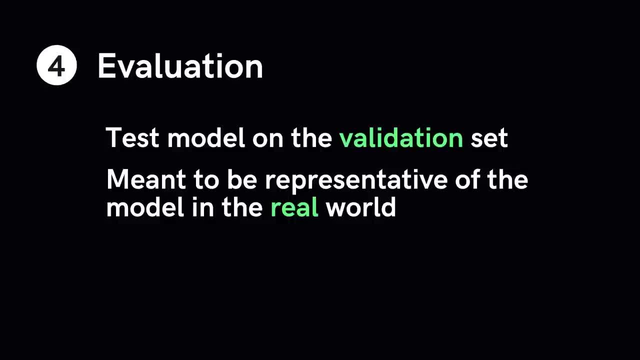 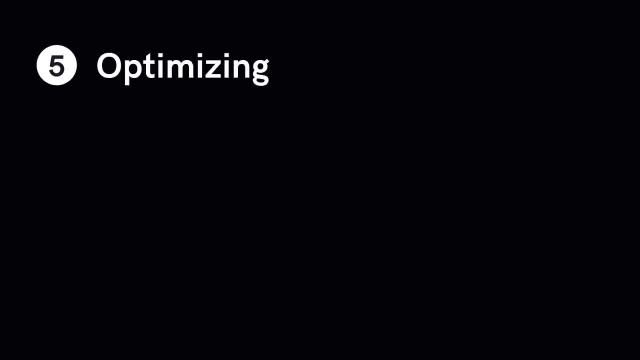 that we had set aside earlier. The evaluation process allows us to test our model against data it has never seen before, and this is meant to be representative of how good the model might perform in the real world. After the evaluation process, there's a high chance that your model could be optimized further. Remember we started with random weights. 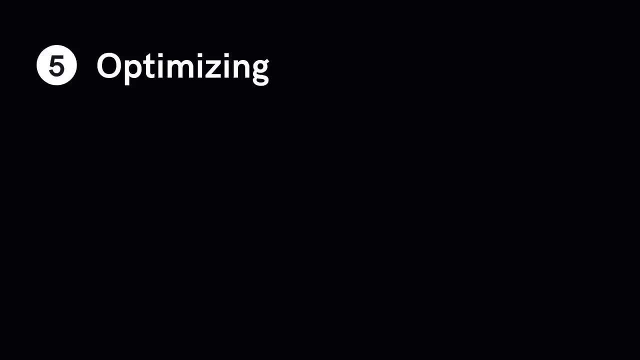 and biases, and these were fine tuned during back propagation. Well, in quite a few cases, back propagation won't get it right the first time, and that's okay. There are a few ways to optimize your model further. Tuning hyperparameters is a good way of optimizing your model's performance. One: 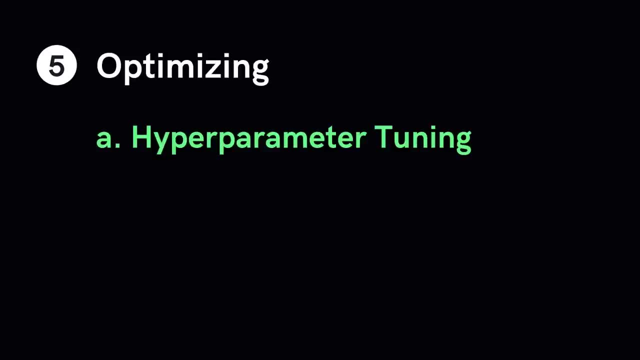 way to do this is by showing the model, the entire data set, multiple times, That is, by increasing the number of epochs. This has sometimes shown to improve accuracy. Another way is by adjusting the learning rate. We talked about what the learning rate was in the previous module, but we'll talk about that in the next video. 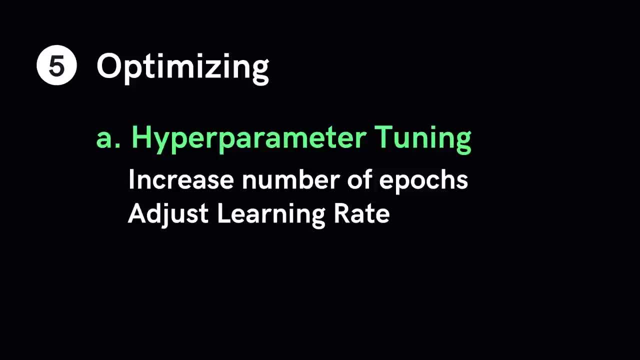 So if you don't know what the learning rate is, I do advise you to check out the previous module. But essentially, the learning rate defines how far we shift the line during each step, based on information from the previous training step in back propagation. These values 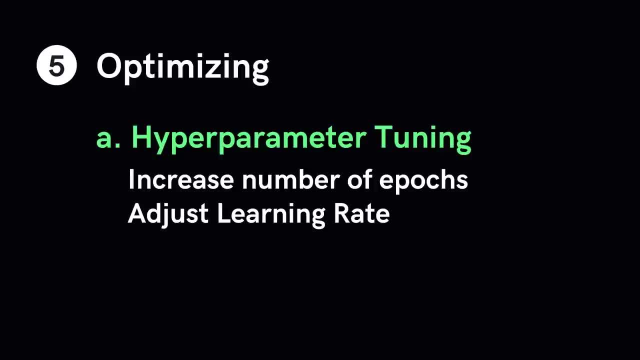 all play a role in how accurate a model can become and how long the training takes. For complex models, initial conditions can play a significant role in determining the outcome of training. There are many considerations at this phase of training and it's important to define what makes a model good enough. Otherwise you might find yourself tweaking. 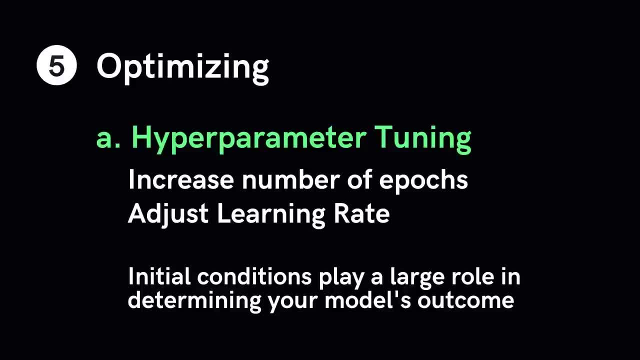 parameters for a long, long time. The adjustment of these hyperparameters remains a bit of an art and is more of an experimental process that heavily depends on the specifics of your data set model and training process. You will develop this as you go more and more. 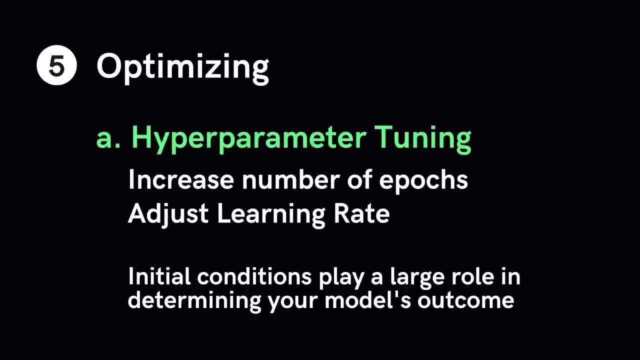 into deep learning, so don't worry too much about this now. One of the more common problems you will encounter is when your model performs well on training data, but performs terribly in the training process. This is because the model does not perform well on training data, but performs terribly in the training process. This is 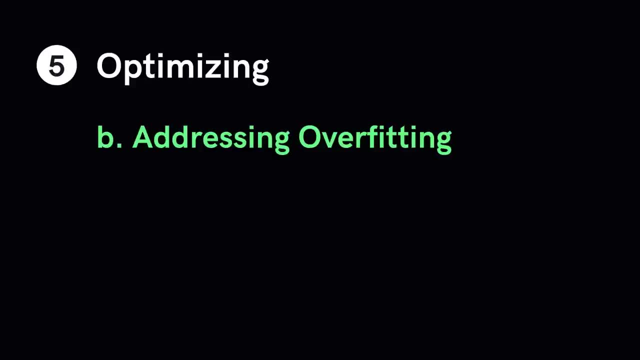 because the model does not perform well on training data, but performs terribly on data it's never seen before. This is the problem of overfitting. This happens when the model learns a pattern specific to the training data set that aren't relevant to other unseen. 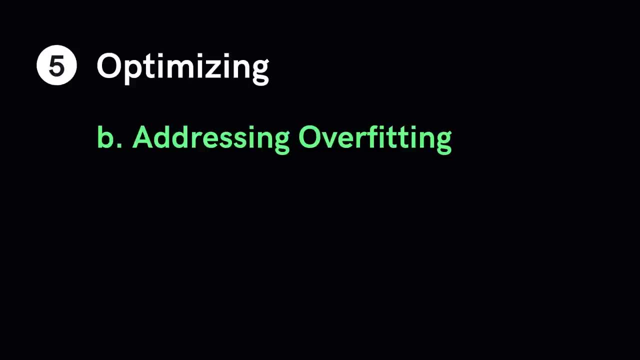 data. There are two ways to avoid this overfitting: Getting more data and regularization. Getting more data is usually the best solution. A model trained on more data will naturally generalize better, Reducing the model's size by reducing the number of learnable parameters in the model and with it, its learning capacity is another. 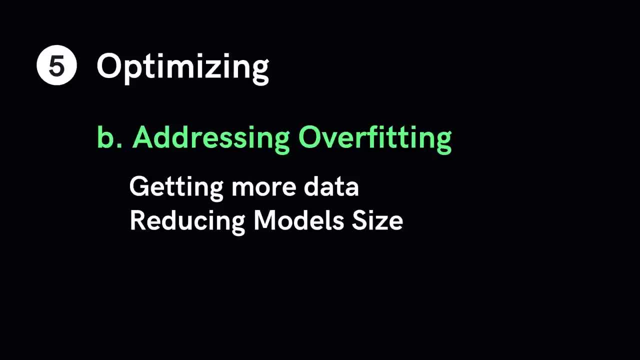 way. However, by lowering the capacity of the network, you force it to learn patterns that matter or that minimize the loss. On the other hand, reducing the network's capacity too much will lead to underfitting. The model will not be able to learn the relevant patterns. 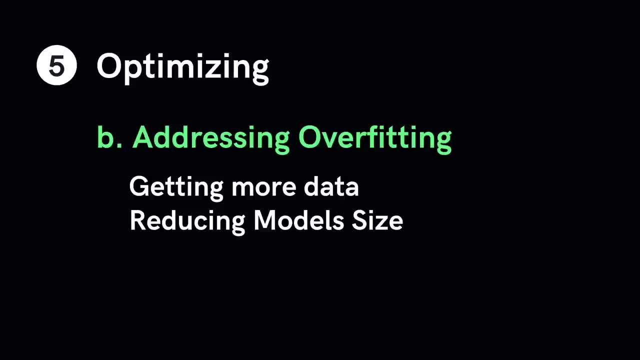 in the trained data. Unfortunately, there are no manageable formulas to determine this balance. It must be tested and evaluated by setting different parameters and observing its performance. The second method to addressing overfitting is by applying weight regularization to the model. A common way to achieve this is to constrain the complexity of the network by 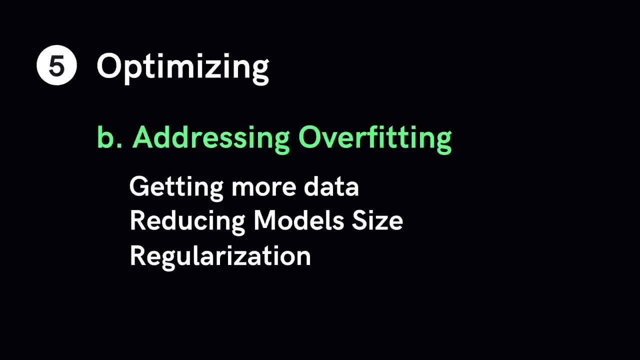 forcing its weights to take only small values. regularizing the distribution of weight values. This is done by adding to the loss function of the network a cost associated with having large weights, And this cost comes in two ways: 1. Regularization at a cost with regards to the absolute value of the weight coefficient. 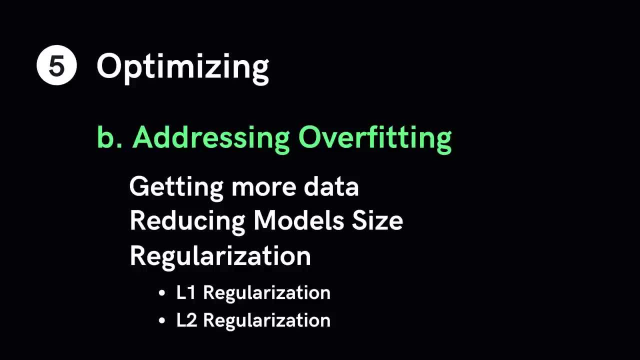 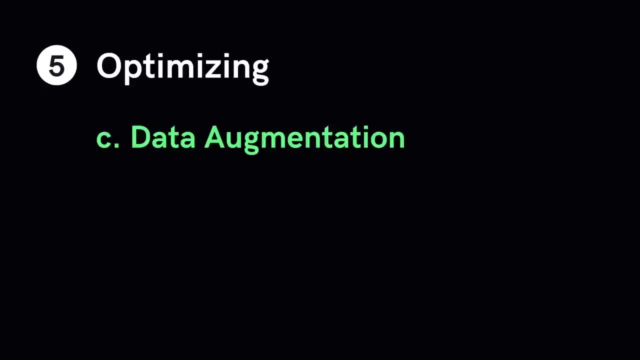 2. Regularization at a cost with regards to the squared value of the weights coefficient. Another way of reducing overfitting is by augmenting data. For a model to perform well or satisfactory, we need to have a lot of data. We've established this already, But 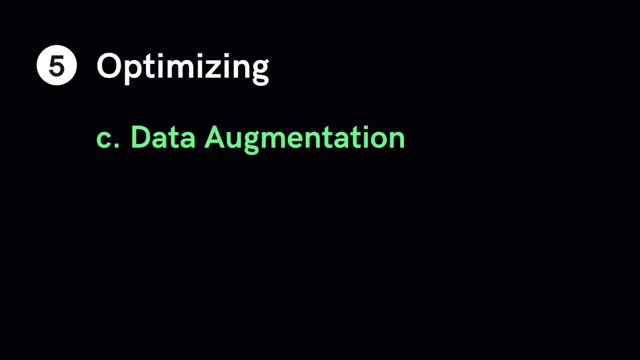 typically, if you're working with images and you want to increase the number of layers, there's always a chance that your model won't perform as well as you'd like it, no matter how much data you have. In cases like this, when you have limited data sets, data augmentation is a 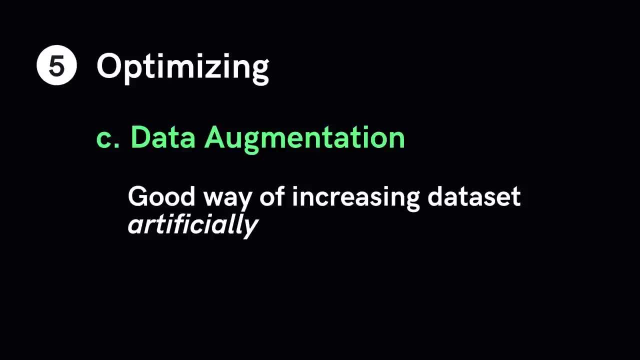 good way of increasing your data set without really increasing it. We artificially augment our data, or in this case, images, so that we get more data from already existing data. So what kind of augmentations are we talking about? Well, anything from flipping the image of the y-axis. 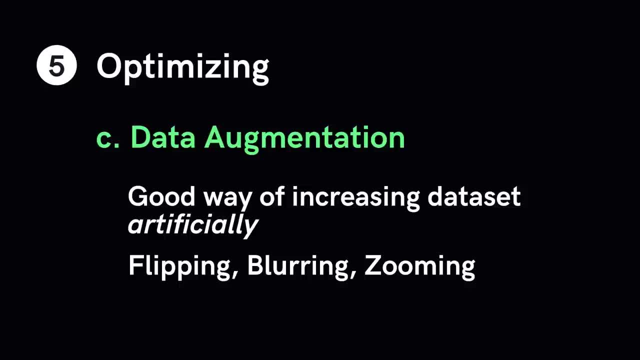 flipping over the x-axis, applying blur to even zooming on in the image. What this does is that it shows your model more than what meets the eye. It exposes your model to more of the existing data so that in testing, it will automatically perform better because it has seen images represented in 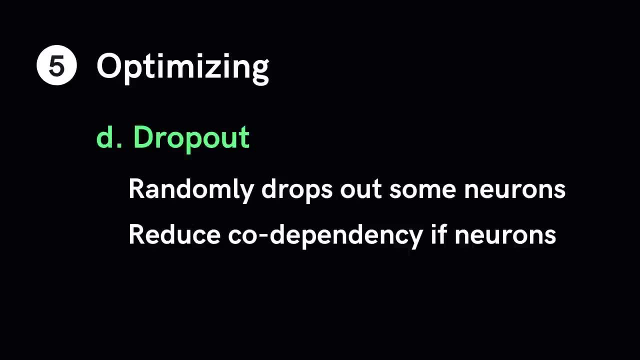 almost every single form. Finally, the last method we're going to talk about is dropout. Dropout is a technique used in deep learning that randomly drops out units or neurons in the network. Simply put, dropout refers to the ignoring of neurons during the training phase of a randomly 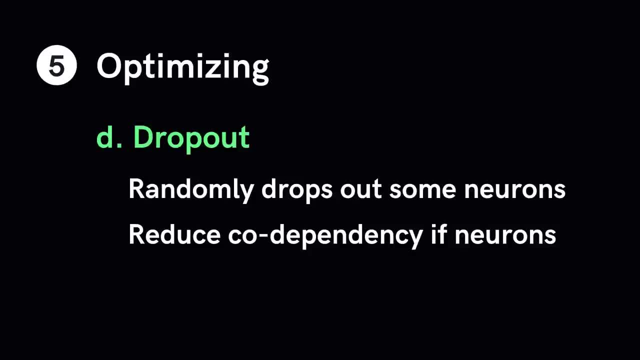 chosen set of neurons. By ignoring, I mean that these units are not considered during a particular forward or backward pass. So why do we need dropout at all? Why do we need to shut down parts of a neural network? A fully connected layer occupies most of the parameters and hence